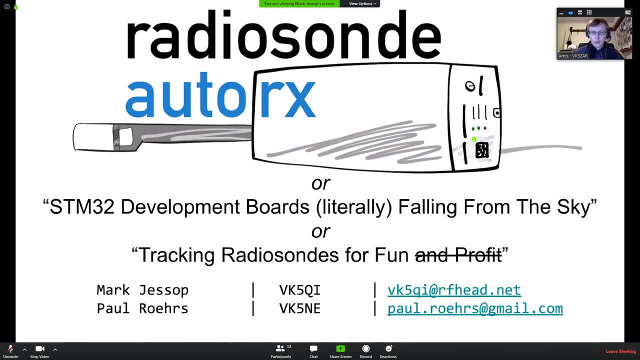 So here we go Right. So again, thanks very much to the Elizabeth Amateur Radio Club for allowing me to do this presentation and thanks, Paul as well for letting me kind of jump in and give this presentation. This is a presentation. it's an amalgam of some presentations that I've 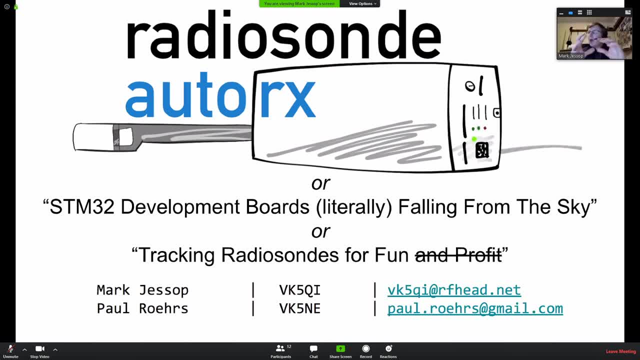 given previously at Linux Conference and at the AREG Club, and also that I was going to be giving at other radio clubs as well. So EARC's the first. You're welcome. So this talk is all about radio songs and how we can track them and reuse them. There's a number of different titles that I've 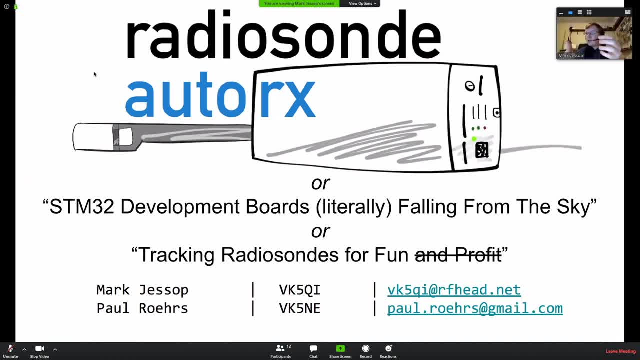 used for this presentation, but I'm going to start with the first one, which is the one I've used for this talk in the past, one of which is, you know, tracking radio songs for fun and no profit, And the other one is STM32 development boards literally falling from the 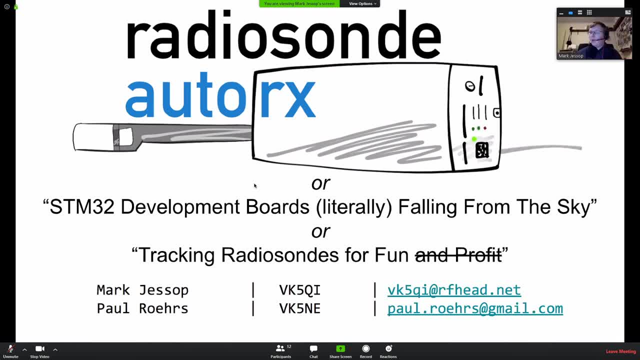 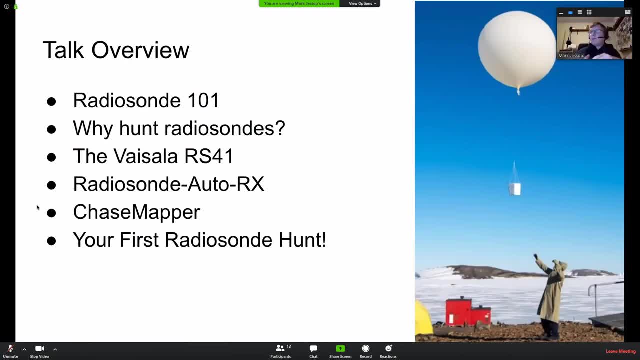 sky, which is exactly what they are. If I make sure I'm focused on the right window, I can actually change slides. Here we go. So in this talk I'll cover you know what a radio song is, how they work, why we bother chasing them. I'll give some details. 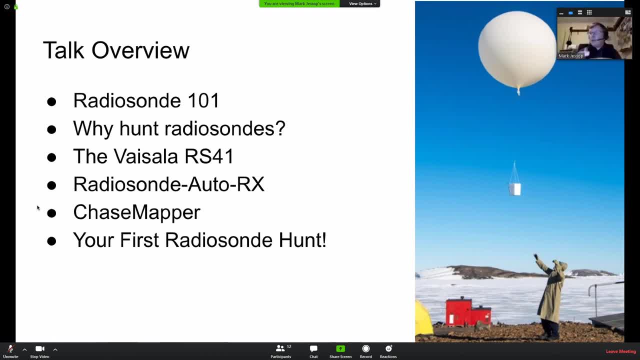 on a couple of different radio song types and in particular the Vysala RS41,, which is what's most commonly flown here in Australia and around the world in fact. And then I'll talk about the radio song decoding software which I've developed and then how you can go in and track and recover. 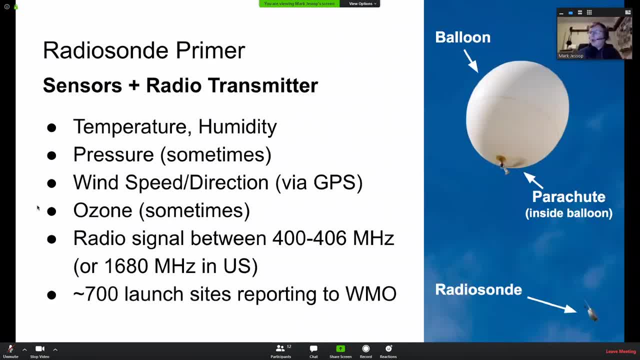 these radio songs for yourself. So RadioSongs 101, what is a radio song? Well, it's a scientific device launched underneath the weather balloon, used for radio songs, and it's used for radio songs to take measurements of the upper atmosphere, the measurements of the stratosphere, I should say. 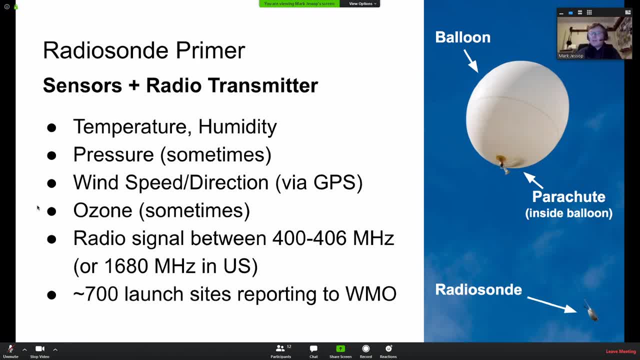 And generally it's some kind of sensors and a radio transmitter of some sort to get telemetry back to the ground. Most commonly you'll find the radio songs have temperature and humidity sensors. Some of them have pressure sensors. They almost always have some kind of way. 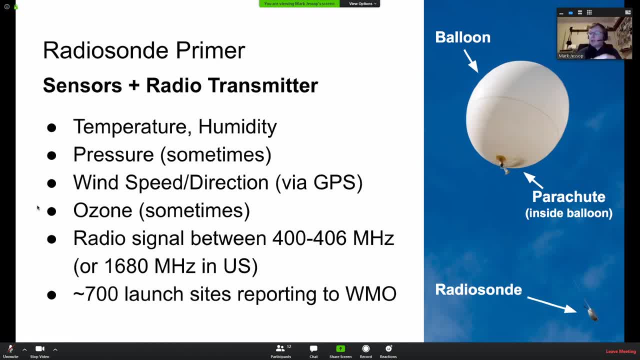 of measuring wind speed and direction, which nowadays is via GPS, but back in the day it was via radar. Sometimes you find they have ozone sensors on board as well, which I'll talk about in a little bit. There's one sitting down beside me, And in most parts of the world they transmit a radio. 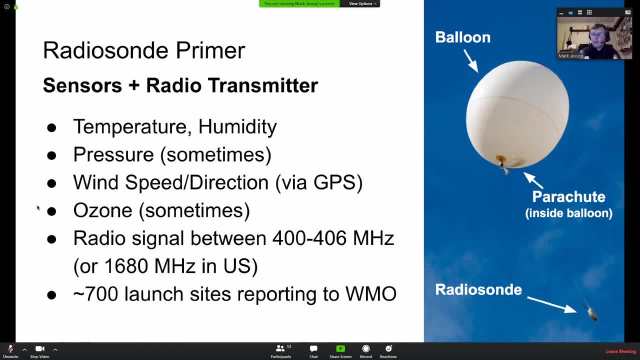 signal somewhere between 400 and 406 megahertz. It's almost the case all around the world, except for the United States, who have to do things differently as usual, And many of their radio songs transmit on L bands. so 1.68 gigahertz. 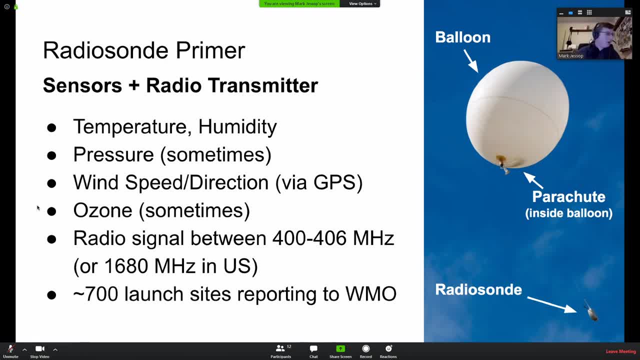 And that's the timeout timer. Here we go. DK5QI- Though the US is transitioning back to 400 megahertz as well- for commonality in hardware. At the moment there are 700 radio song launch sites which report to the World Meteorological Organization. There are more that don't report. 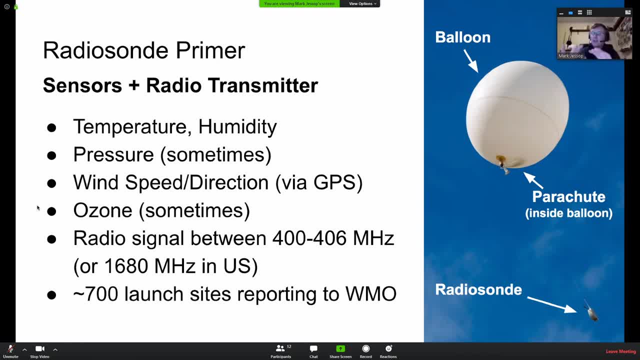 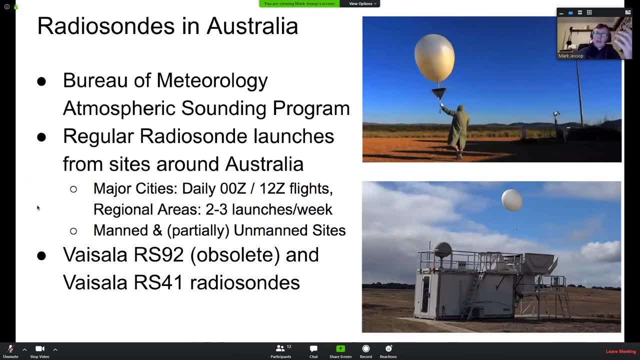 to that organization, but it's somewhere in the vicinity of 700 to 1,000 launch sites that are launching daily In Australia. of course we have the Bureau of Meteorology and the Atmospheric Sounding Program. They launch from various sites around Australia in major cities, so state capitals. They usually launch in twice. 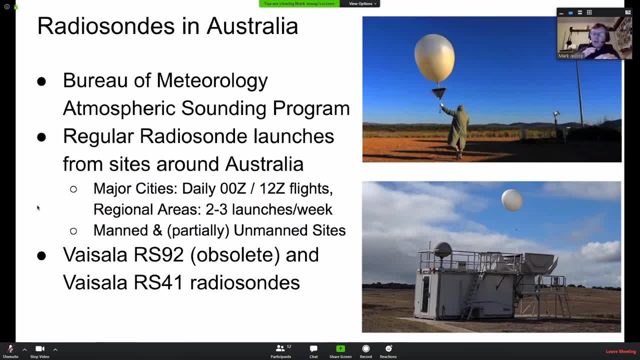 per day- not always but mostly- And there are also many launch sites in regional areas which may not be launching every day- Normally it's a couple of days a week- And there's also a combination of manned, so mostly manual. Someone presses a button and the radio song. 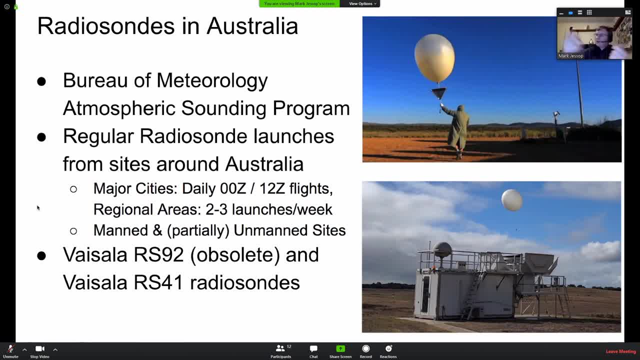 launches Or they go outside and release it, as you can see in the top picture in that slide. And there's also automatic sites as well. I like the one in the bottom of that slide which is a Vaisala Auto-Song Station. That particular one is in Mount Gambier, Mount Gambier. 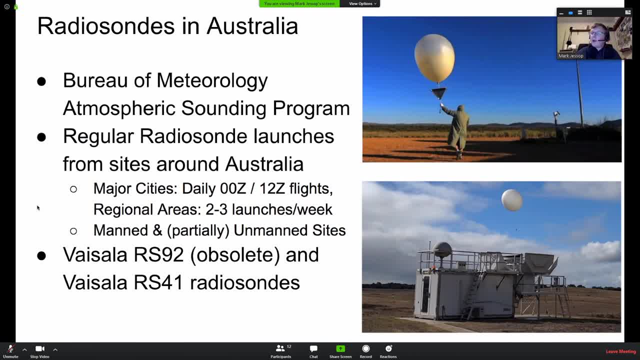 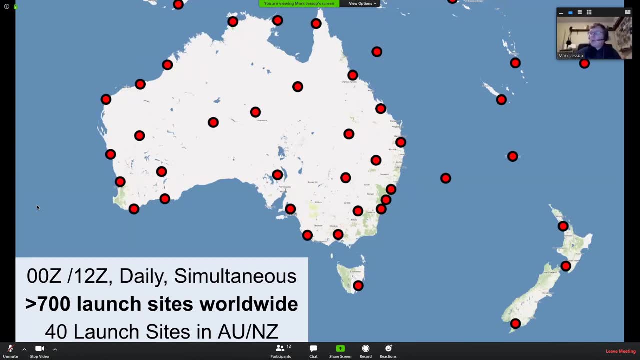 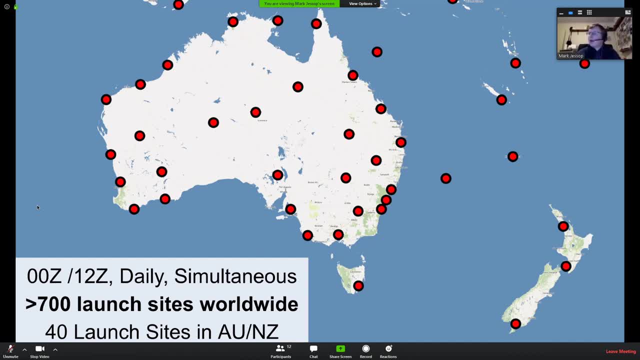 which is a Vaisala RS-41.. Some launch sites are more large strip-ishment zones that have alarm tones. in a couple of hours' drive of them They're all over the country, some very far inland and obviously a lot around the coast. 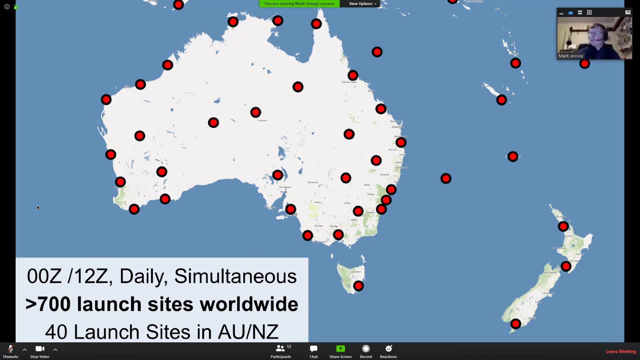 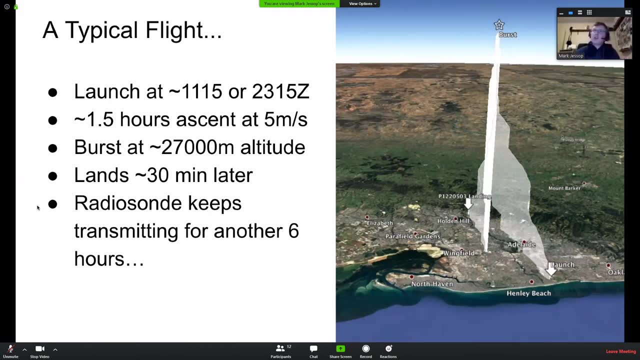 And then there's 40 launch sites within Australia and New Zealand. So a typical radius on flight will launch usually. So the launches are targeted around the times of 0,, 6,, 12, and 18, Zulu. The idea is that. 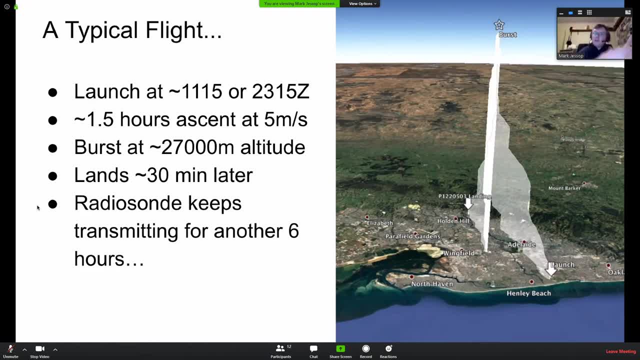 global weather models set out, work around these, around these particular times, and the radiosonde launches a time to capture data throughout that particular time. so to capture data for zero zulu, they launch 45 minutes before at 23: 15 zulu. for capturing data for 12 zulu, they'll launch at 11: 15.. it takes roughly one. 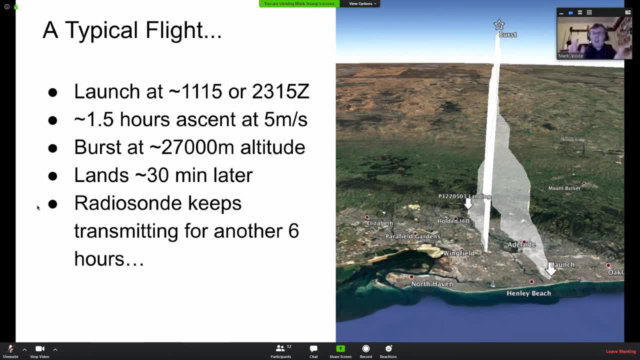 and a half hours for the sonde to ascend to about, you know, 27 kilometers. it really depends upon the launch site. they ascend at about five meters per second, and this value is particularly critical because the sensors are usually calibrated for a certain wind speed or certain air speed past them. 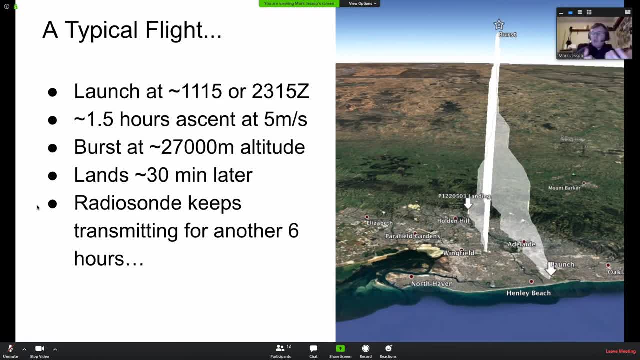 and the balloon bursts and then the sonde will land, usually about half an hour, half an hour later, depending upon what's above the sonde. so something i didn't quite cover. before you know, we're using latex balloons. in the picture before you didn't see a parachute in that particular. 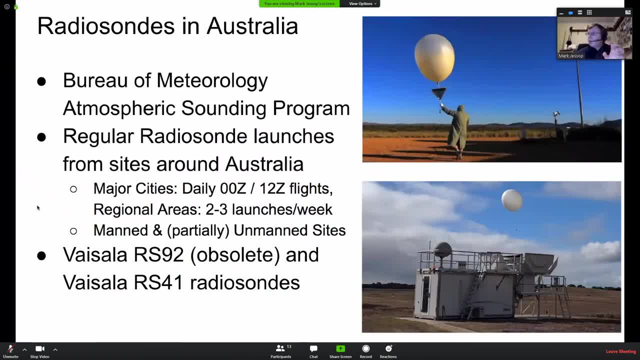 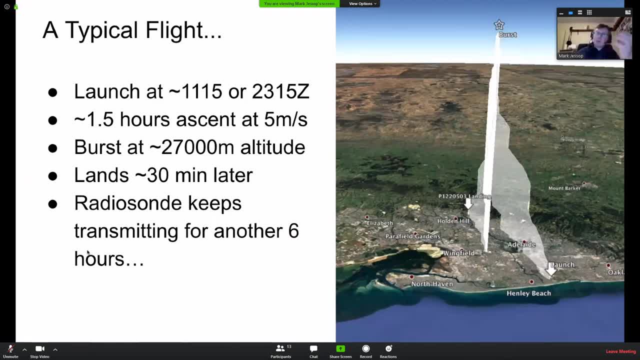 picture, the parachute is actually within the balloon up here. other cases: there may be a separate parachute. in case of launches in adelaide, they're actually using a radar reflector as a pseudo parachute. the reason they're using those is because they have a huge amount of them in stock and they just want to get rid of them. so, anyway, the 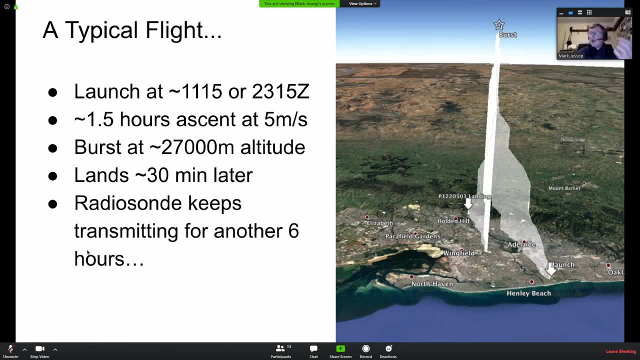 radiosonde, the balloon of earth. the radiosonde will descend, it will land and in the case of the, the visala rsf 41s, they'll keep on transmitting for about another six hours. this is not a battery life limitation, it's actually a timer. so as soon as the balloon bursts, the timer starts up and eight. 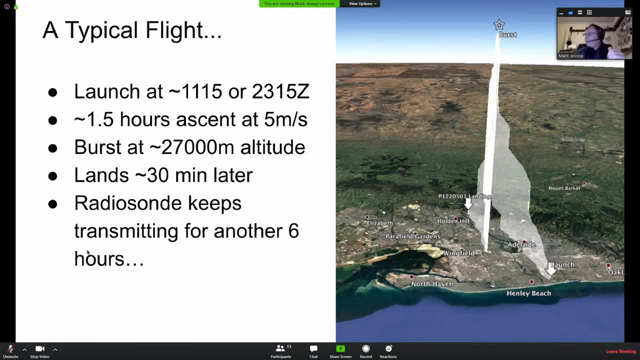 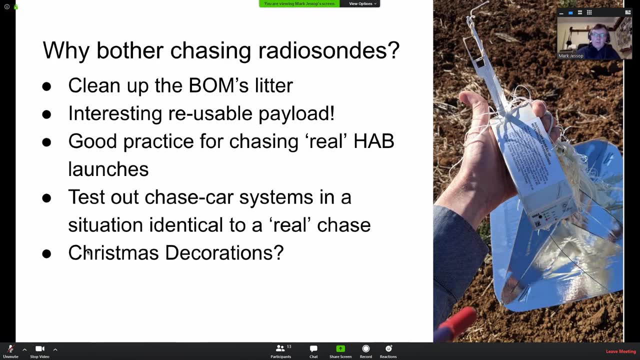 and a half hours later, the balloon, the radiosonde turns off. so why would we bother chasing these devices? well, of all of those 700 radiosonde you know, or more, launches launched per day, uh, precisely none of them are going to be able to launch the radiosonde in adelaide. they're going to. 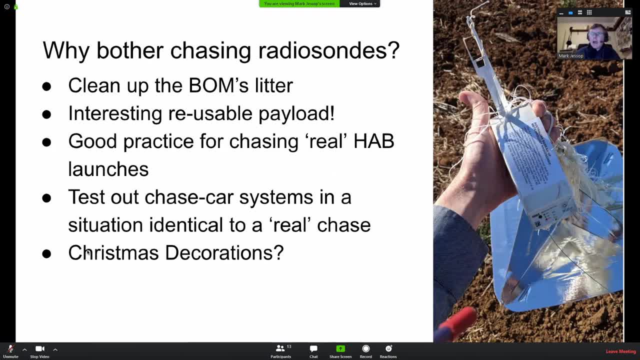 be able to launch ti in adelaide at least once, about four days positive. so this is a very good strategy if you want to go and do your own- higher tube, higher tube, limelight, if you want to go chase someone else's. it's pretty much exactly the same thing, just a bit of a different telemetry. 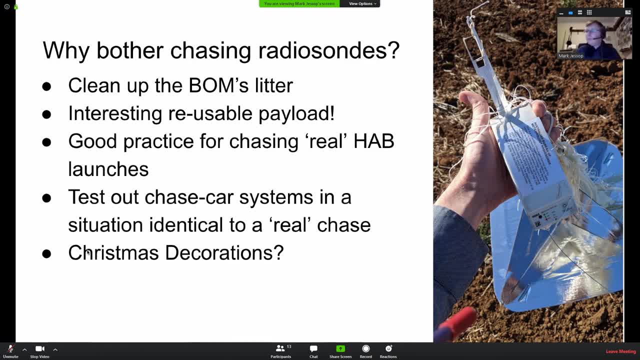 source. yep, there we go. it's a good way of testing out chase car systems to see whether you know that you're going to be able to launch them. it's going to be dangerous to be able to run out of them and you don't want to do it because you don't wing it there's. there's a very massive이�bearing risk of being affected by a landmine explosion from theestersia. there's a big risk to do that, so you don't want to go. that's right. the radiosonde: it's a pretty big risk. the best way to do that is is to do it in an adelaide to see if you can just run in the lab you can. 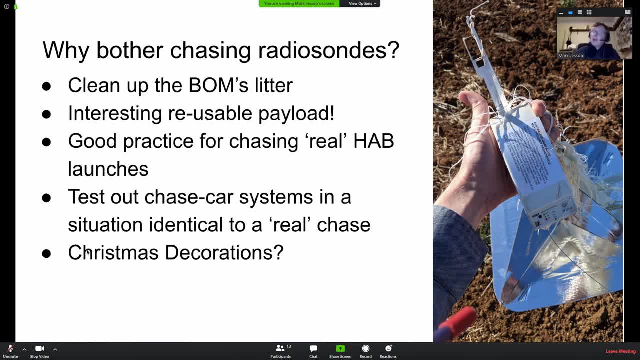 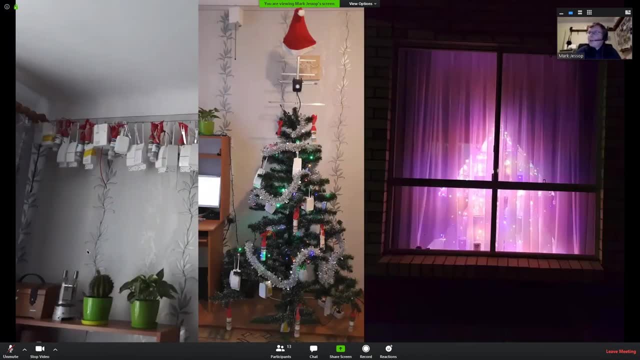 You can chase a balloon flight And of course, the payloads- in the case of Australia- are very, very reusable. You can do all sorts of things with them And finally, you can make really good Christmas decorations out of them. So here's some, a nice Christmas tree. 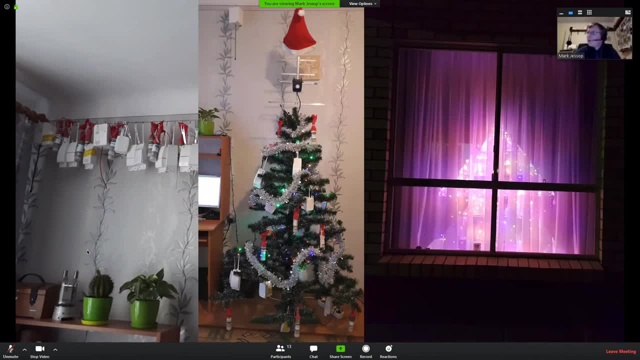 with some radio songs hanging off of it, And on the right hand side there is Paul BK5NE's radar reflector Christmas ornament. I really love what you've done there, Paul. That's brilliant. So there are many different types of radio songs. 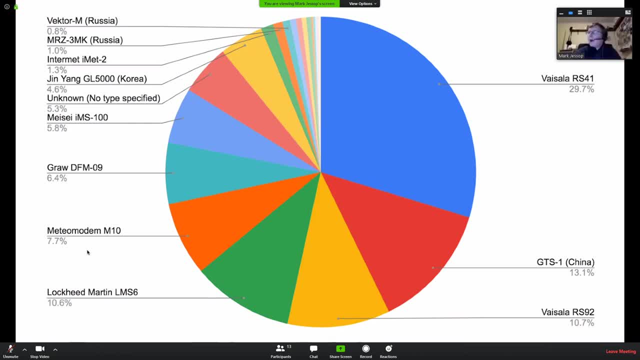 used worldwide. heaps of different models. This pie chart kind of shows the different types that are launched. There's the pretty much the predominant type is the Vaisala RS41, which takes up 30% of the world's market share. 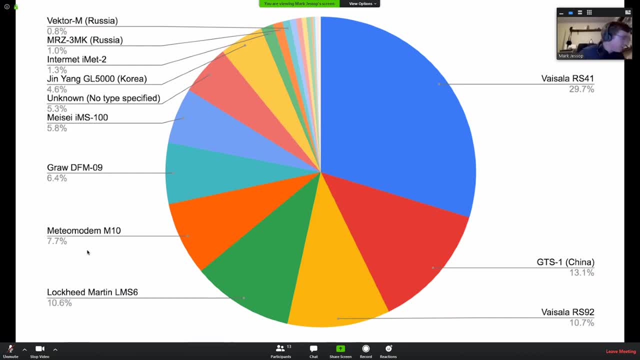 And then there's a number of other types as well, So I'm gonna go through a couple of these now and apologies to the people listening on the repeater, I don't have slides for this part, So I have a selection. I have a selection of different types of radio songs here. 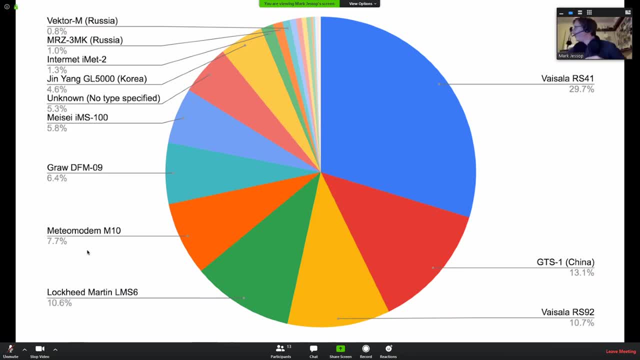 First up, going from, well, biggest to smallest. in some respects, this is a Lockheed Martin LMS-6 radio song And it is probably the biggest. well, neglecting the Ozone song which is down there, This is probably the biggest radio song. 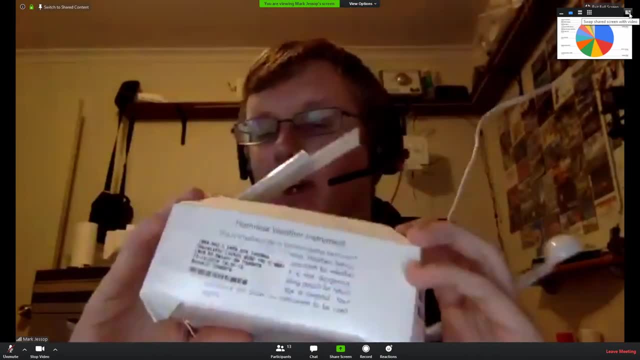 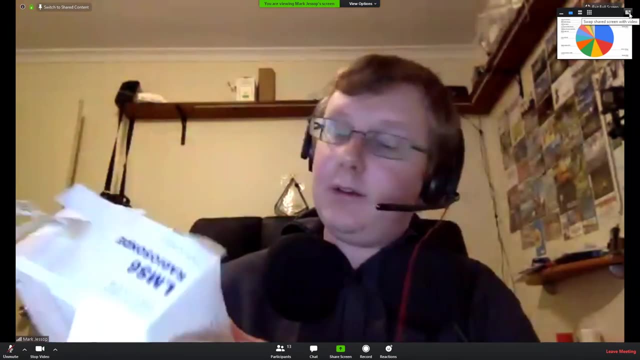 on the market at the moment. It's also ancient. These were designed in about 2005 and they're still flying them. They're heavy. This one actually runs on L-band on 1.6 KW, 6 gigahertz as well. 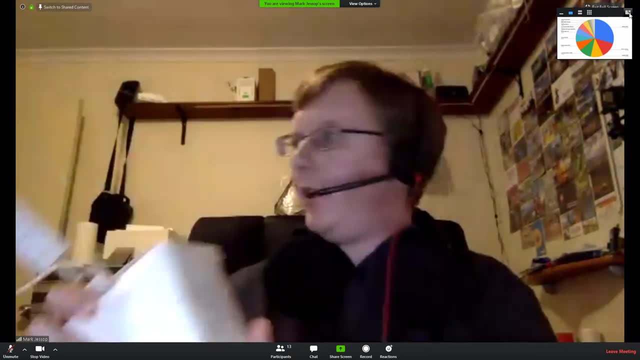 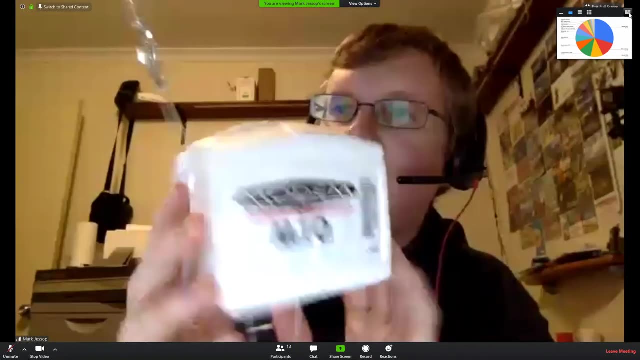 So I was sent this to be able to add support for this particular radio song type to my software. The French did their own thing and made their own a Michio Modem M10.. You'll notice there's a trend here. They're all white boxes made out of foam. 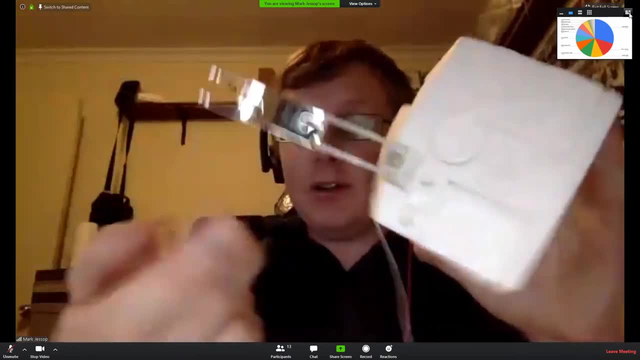 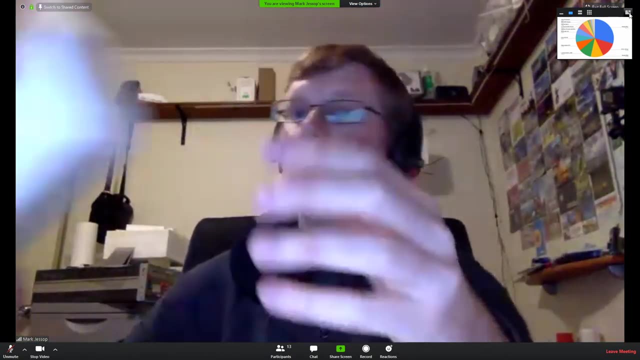 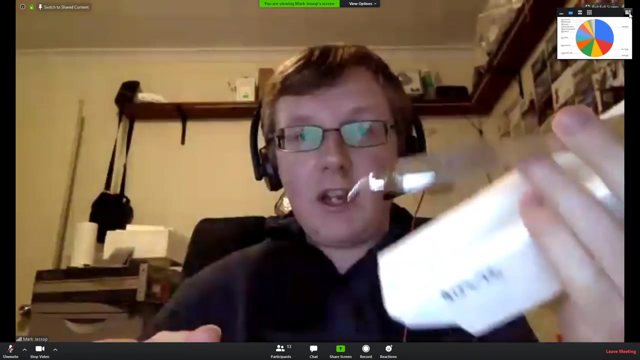 And it does the same thing. There's a temperature sensor and humidity sensor and a GPS inside of it and an antenna. The Germans did their own as well. This is the DFM-09.. Again, same thing: Radio microcontroller, temperature sensor. 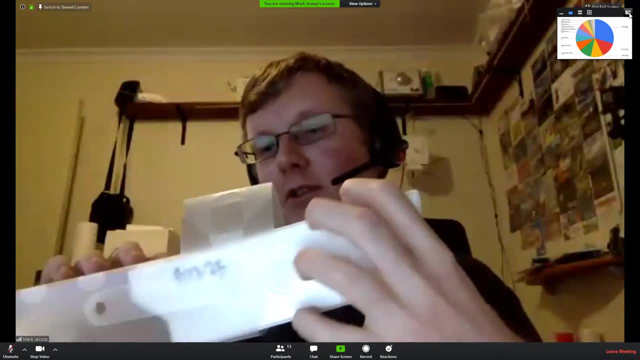 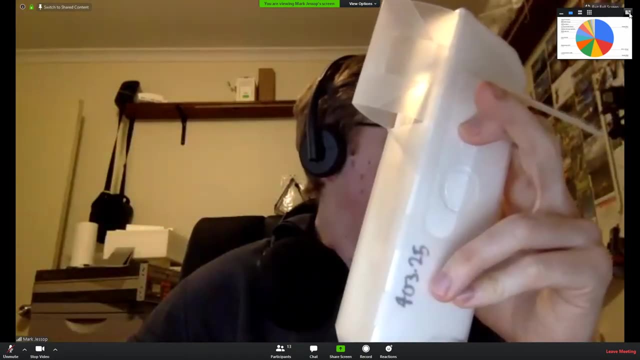 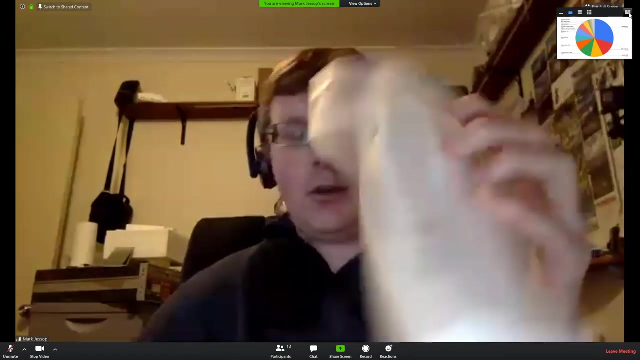 humidity sensor. It's all sounding pretty familiar. Of interesting note, we didn't think these were launched in Australia. We thought these were a European only thing. As it turns out, there is the Snowy Mountains Hydro scheme actually launched these particular radio songs. 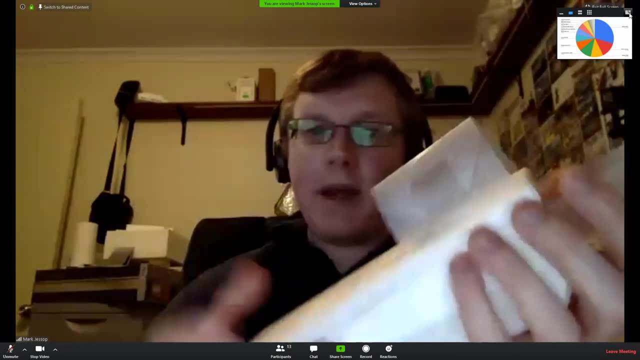 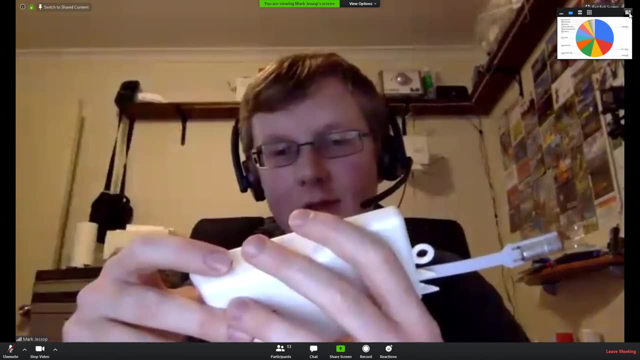 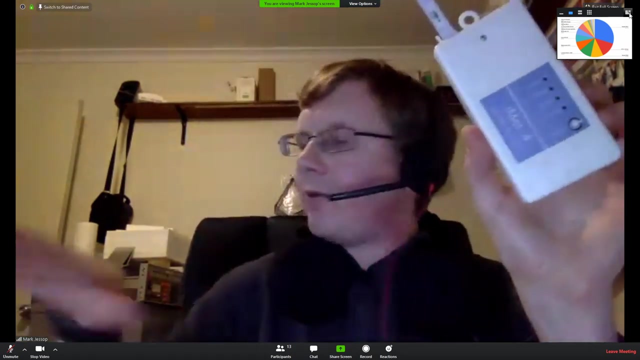 as part of their cloud seeding program in the Snowy Mountains, So occasionally we see one of these things here on the tracking network. The South Africans built their own as well. This is an internet IMET-4.. And while most of these radio songs that I've got here 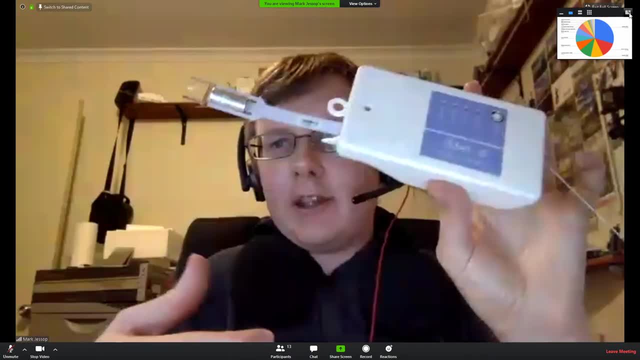 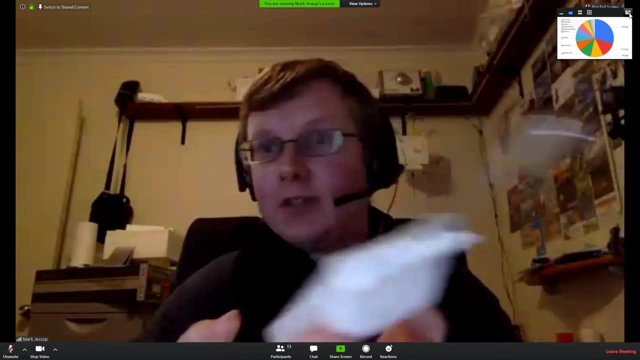 transmit frequency shift keying FSK. This one transmits AFSK at 1200 baud. That might sound familiar to you. It's exactly the same as APRS. Not the same format exactly, but it's very, very similar. 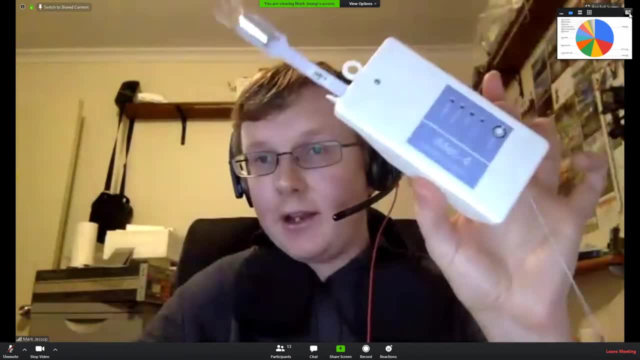 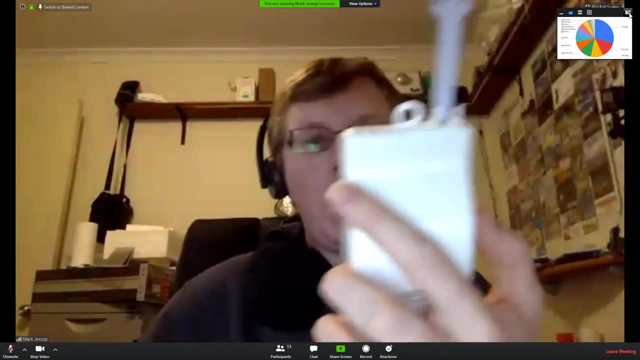 The reason they do that is because the ground stations for these particular radio songs are based in Africa. radiosondes is an ICOM ICR10, which is a big brother, or the newer version of this scanner that I've got here in my hand. So, yeah, they designed it to be as easy as possible to receive. 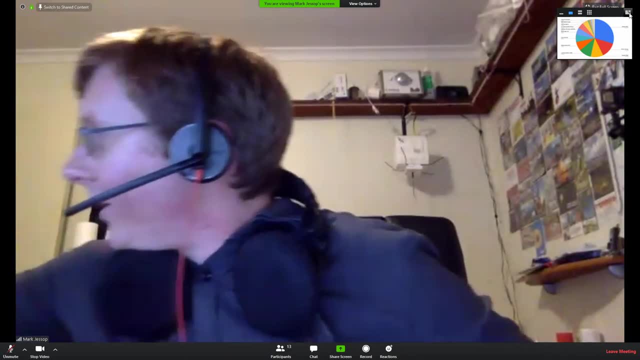 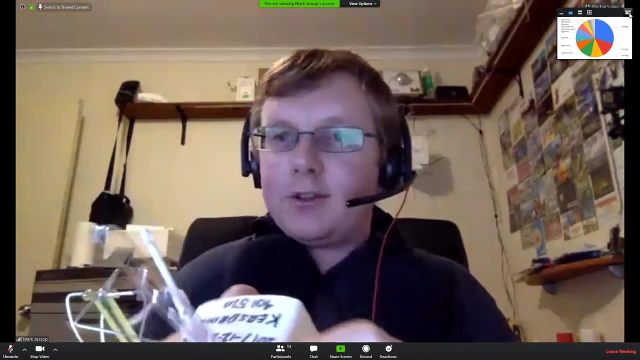 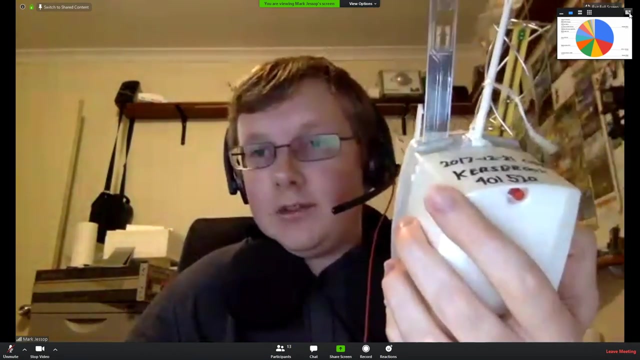 which is pretty interesting. Now we get to the Finnish radiosondes, the Vaisalas- Vaisala being the market leader in radiosondes at the moment. This is an RS92. These are now obsolete, but these were flown for many, many years in Australia and you may, if you've recovered a radiosonde in the. 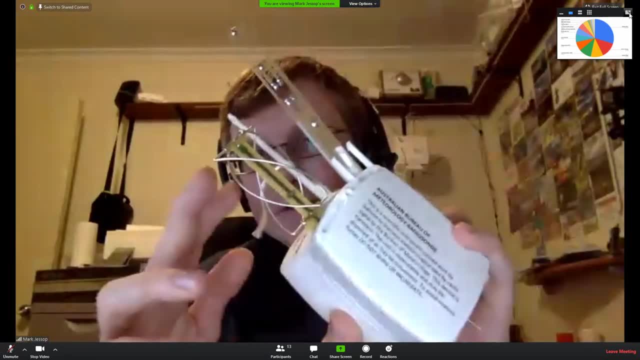 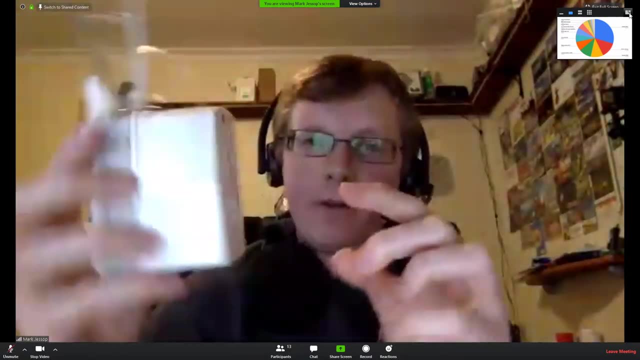 last 10 years. you've probably seen one of these. It's got a nice big fat helical antenna, a GPS on top and the sensor stalk as usual- temperature sensor and humidity sensors and a very large battery in the back. This radiosonde is a little bit interesting in that there's a lot of custom. 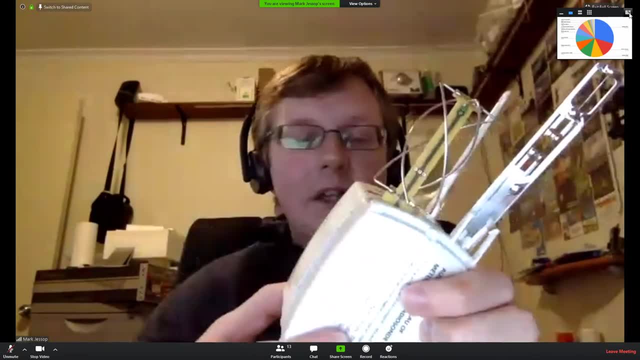 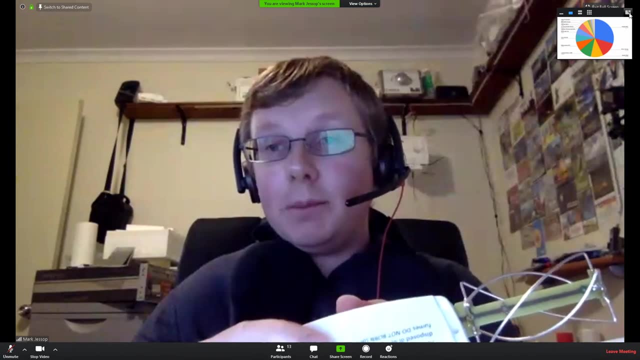 silicon inside of this box, The Vaisala. I don't know why they did it, but they did it and they basically made their own microcontroller And made their own radio transmitter chip. It's all custom silicon. It's incredible. It's also. 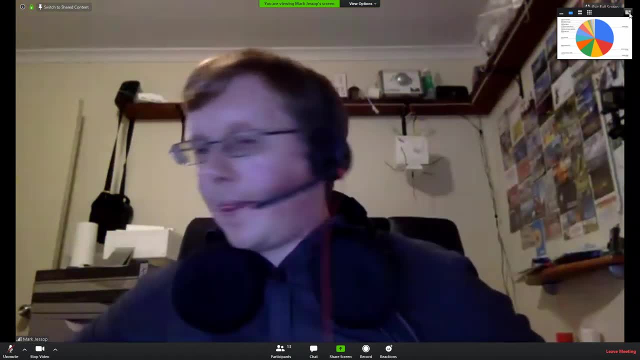 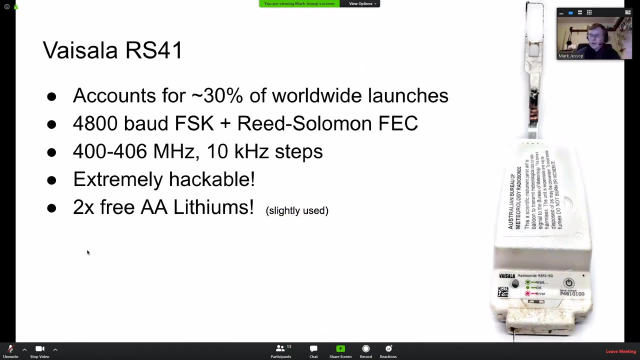 almost impossible to reuse, So anyway. Finally, we end up with the Vaisala RS41.. This is the yeah accounts currently for 30% of worldwide launches, And so the Vaisala RS41 transmits 4,800 board. 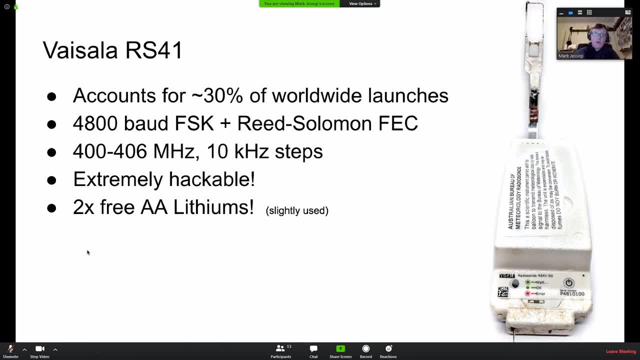 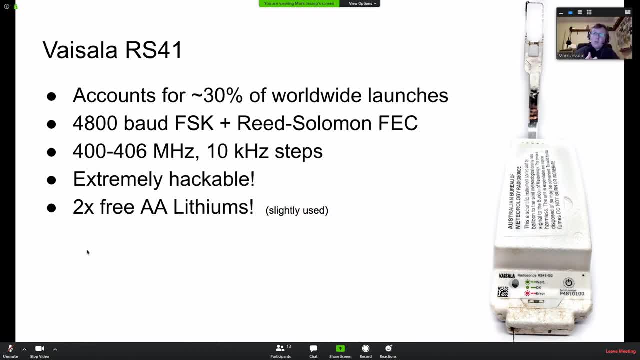 configuration between 400 and 406 megahertz. It will. the radio chip inside of it will go a lot further than that. Being the most common radiosonde out there, it has had the most amount of reverse engineering applied to it. Thankfully, unlike the RS92, it is nothing. it's all commodity. 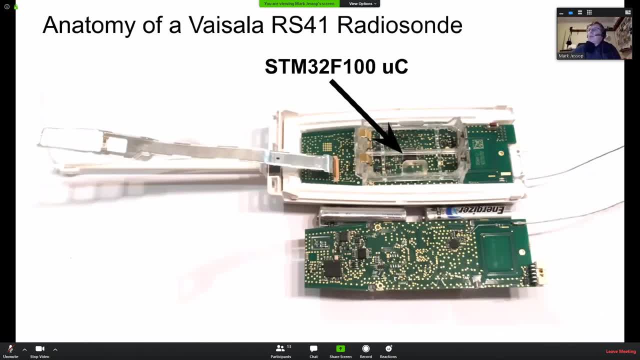 components, So I'll get into that a little bit more. So what's inside one of these RS41s? Well, first up, we have a STM32 microcontroller. Well, first up, we have a STM32 microcontroller, ARM Cortex-M0 microcontroller, Easy to reflash. We have a uBlox chipset, a GPS. 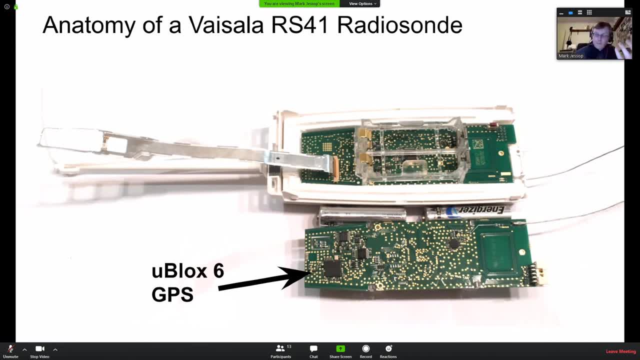 chipset, Again a very, very common GPS chipset, very high-performing chipset, Also very obsolete, this particular version. I don't quite know what Bisal's plans are in this situation. I'm hoping there'll be a broad refresh with a more modern GPS, but we'll see. There is a radio chip which is a Silicon. 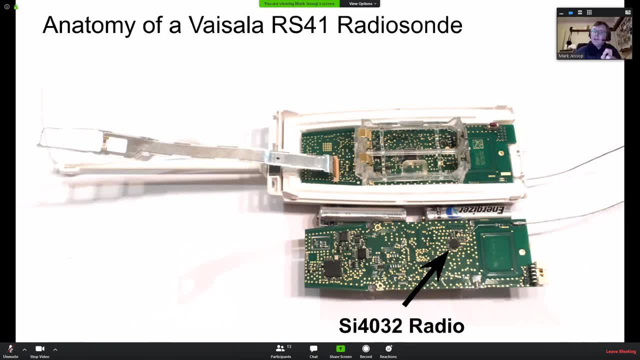 Laboratories SI4032.. This particular radio chip will tune anywhere between about 300 megahertz and about 1 gigahertz, which is pretty cool, Though the matching network between it and the antenna is only good up to about 450 megahertz or so. But we can tune it to the amateur radio band and 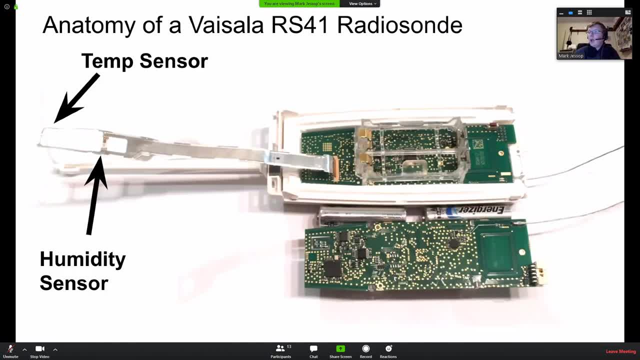 it'll produce about 50 milliwatts of transmit power. The silver stalk that you see is where all of Bisal's secret source lives. This is their temperature and temperature. The temperature sensor is good from about plus 60 degrees to negative 90. 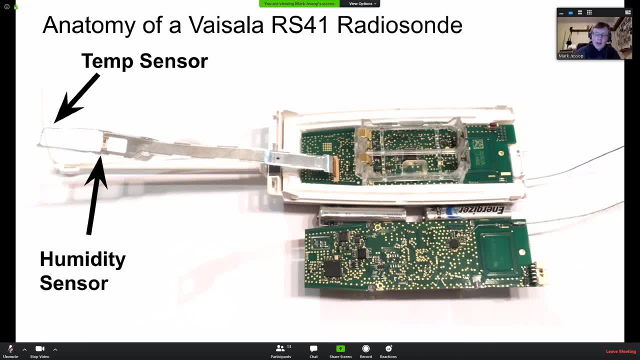 degrees Celsius. It's a platinum wire, it's a resistive sensor, And then there's a capacitive humidity sensor as well. Unfortunately, we don't really know how to reuse any of these at the moment. Bisal have gone and implemented their 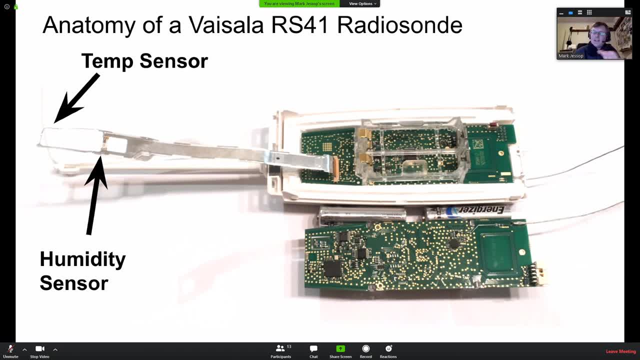 own analog-to-digital converter on the PCB and I think there's a couple of schematics out there for it now, but I don't think anyone's written code to communicate with those sensors. It'd be really cool if someone did, because then you'd have some very nice high-performing temperature and 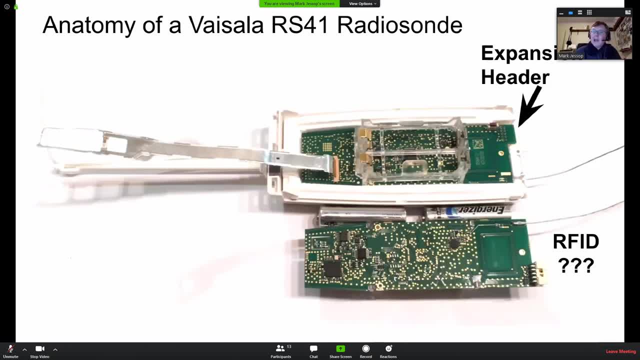 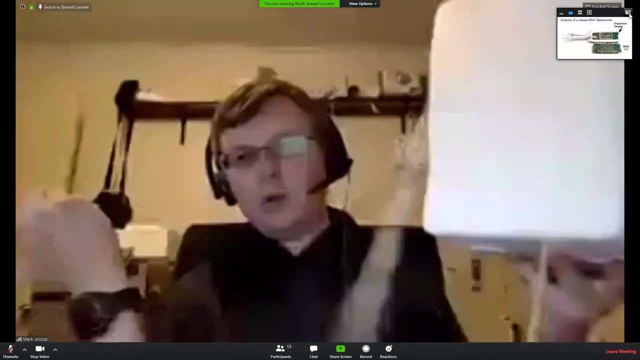 humidity sensors to play with. Last but not least, we have an expansion header, So this is where we would connect things like other sensors. So, for example, this box here is an ozone sonde. Now these are launched in Australia from three places: Melbourne, Macquarie Island and Davis Station. 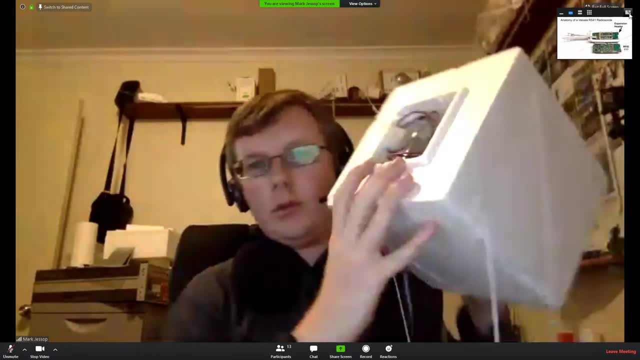 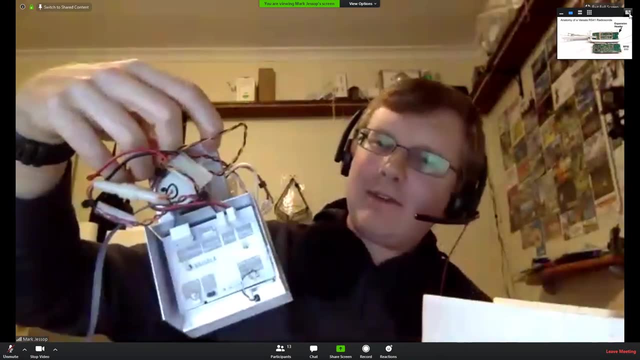 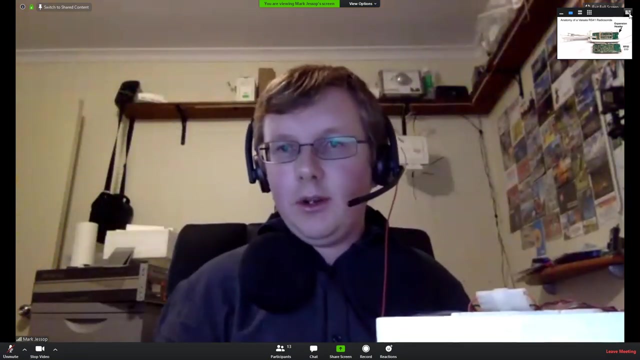 And they're huge. It's mostly foam And inside of it is a. it's some kind of electrochemical cell which can measure ozone And it plugs into the RS-41 via a little connector at the base of the RS-41.. Now the title of this talk was: 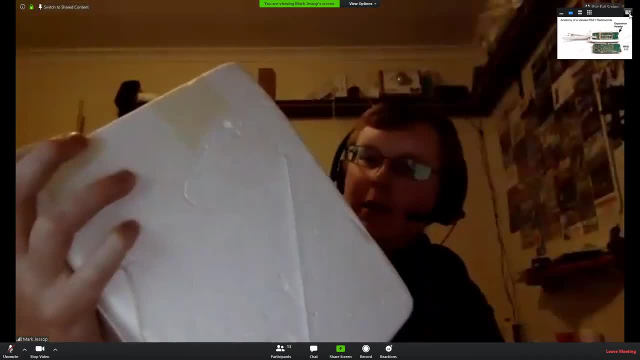 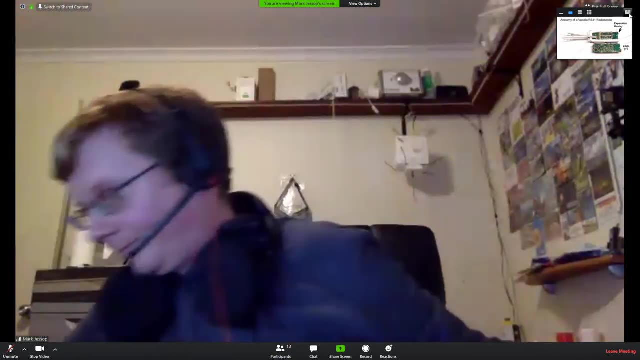 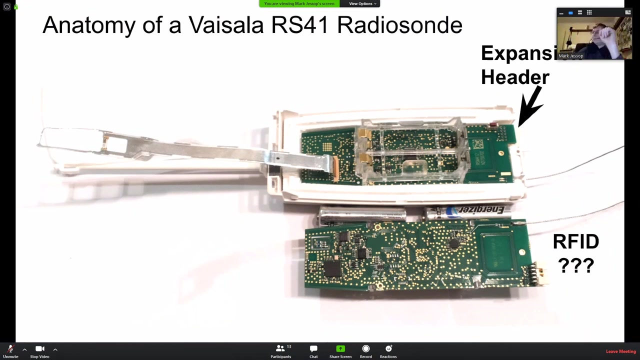 chasing songs for fun and no profit. You get 50 bucks for these if you return them. Doesn't quite cover your fuel. So again, no profit Still holds true. There's also on the RS-41. there's a little coil on the right-hand side of the PCB. This is 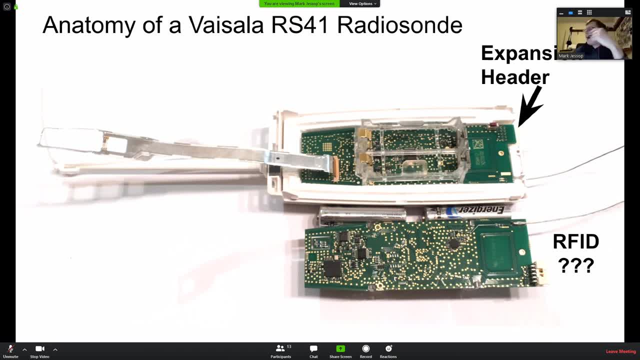 VK-5 Quebec, India, identifying on the VK-5 RLZ, And that coil is used to configure the radio sonde before it's launched. They don't plug into the connector, they just sit it on a little holder and it configures the sonde sets. 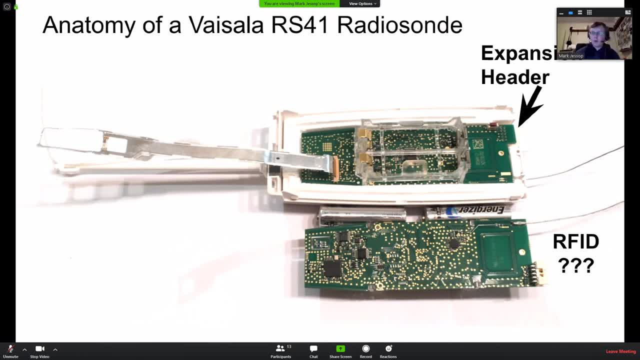 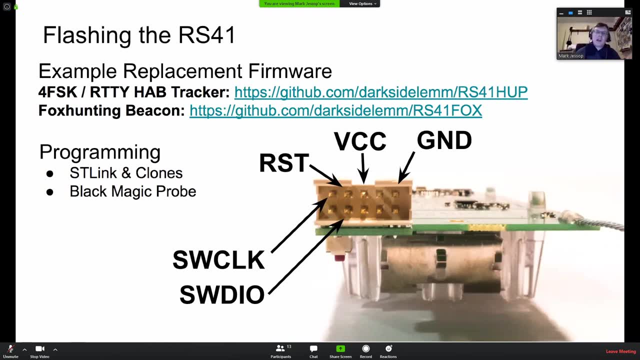 the frequency, applies some calibration parameters and then they take it into the RS-41. outside and launch it So handily that connector at the bottom of the radio sonde also breaks out. programming wires for the microcontroller Makes it very, very. 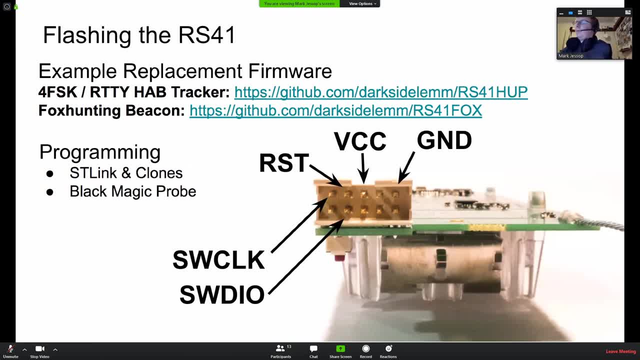 easy for us to reflash them. So I've made up this little adapter here going into an ST-Link programming board. I can plug that into the base of the radio sonde and reprogram it with my own firmware. It's a number of firmwares. 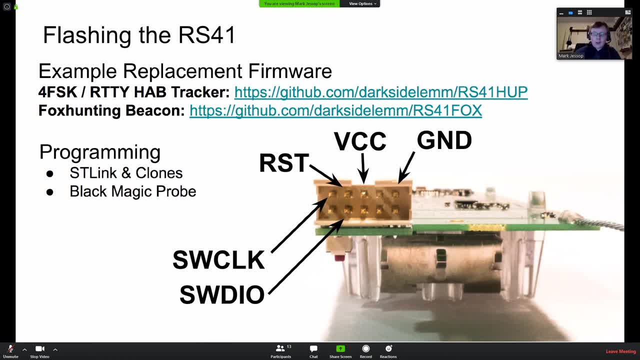 available on GitHub. It's all open source. On the slide are a couple of examples there. For example, RS-41- Fox turns an RS-41 into a fox hunting beacon, So you can make it. you know, here's an RS-41 that I've 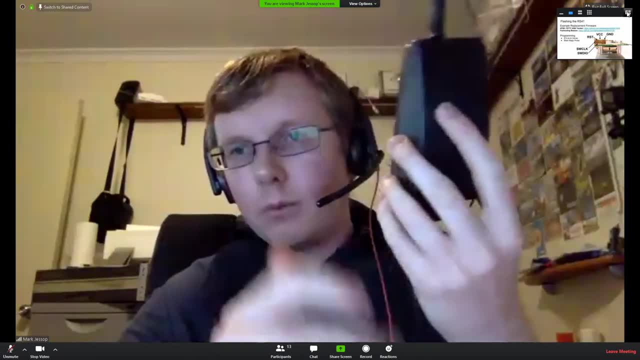 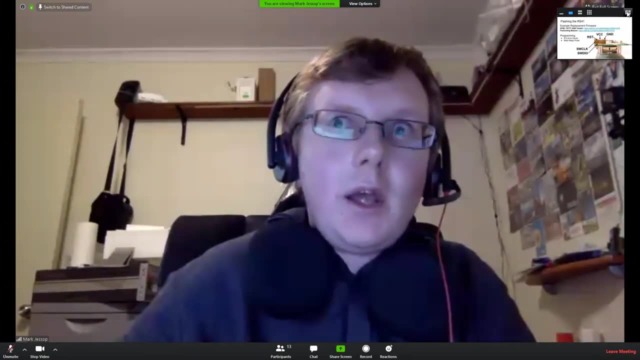 painted black. It's got a magnet in the back of it. I can stick it to metal objects and it will beacon away for quite some time Because there's a GPS on board. when the battery gets flat it'll start beaconing out where it is, so 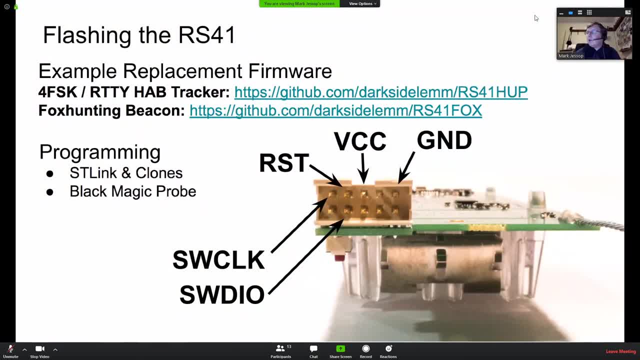 someone can go and find it. The other firmware which I've linked there, the RS-41 HUP, or my specific fork of it, is what we use on all of our Project Horus high-altitude balloon flights. So I launch balloons with Project Horus and yeah, so we. 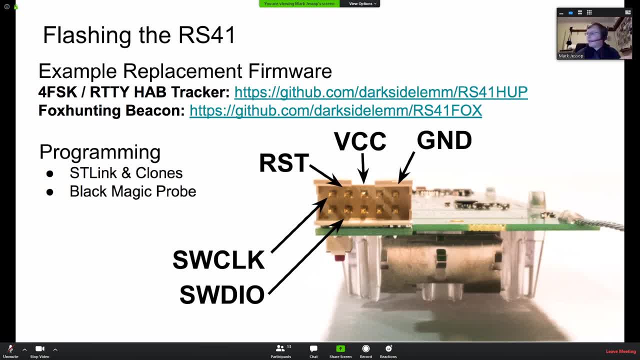 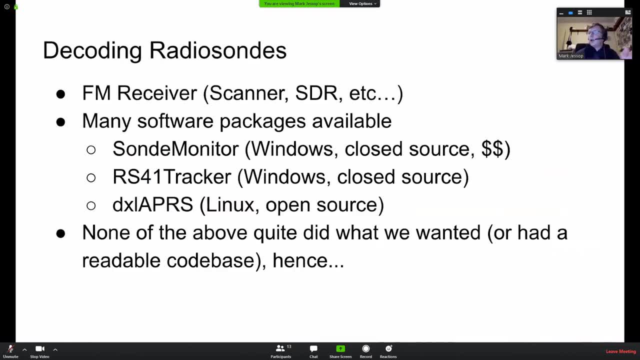 actually use RS-41's reprogrammed ones as our primary telemetry. Now that's a topic for an entirely separate talk. I'm not going to cover it in detail tonight. So how do we go about decoding these? Well, all the radio sondes that I've 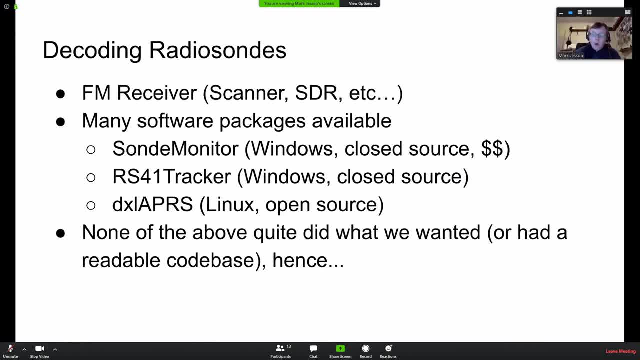 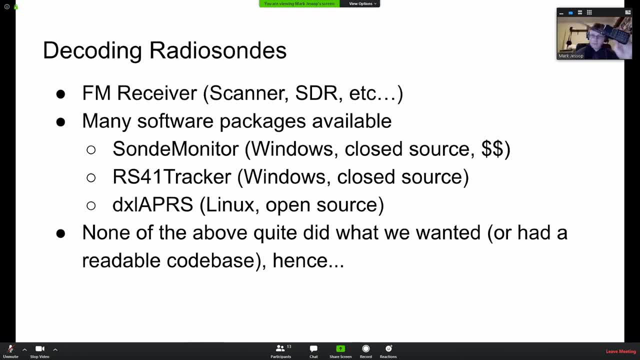 receiver of some description, like a scanner, for example this ICOM IC R10 here. But in many cases, particularly for the radio sondes that use higher board rates, you need something like a discriminator tap So to get unfiltered audio. a standard FM filtered receiver won't work. It's often easier to use. 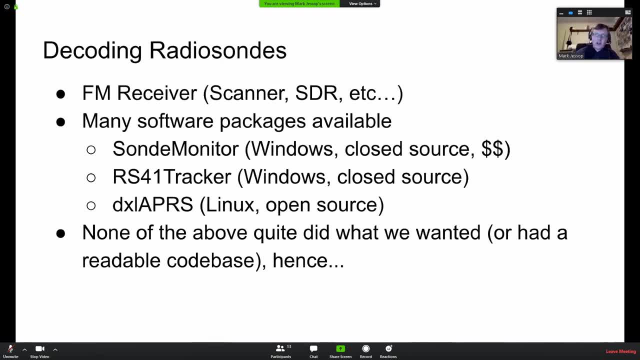 software-defined radio to do this. So using software like SDR sharp or GQ RX- whatever you want to use, there's plenty of options out there. To actually decode telemetry, there's a few options. A sonde monitor is venerable- It's been. 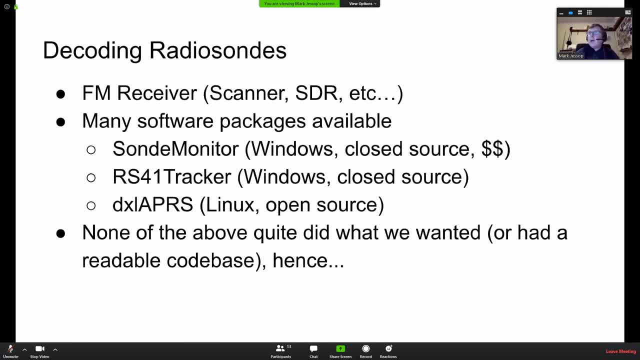 around for at least 12 years, if not more. It costs about 50 bucks and it decodes all sorts of different radio sonde types. The developer, Beb, is a really nice guy. He actually holidays here in South Australia in the 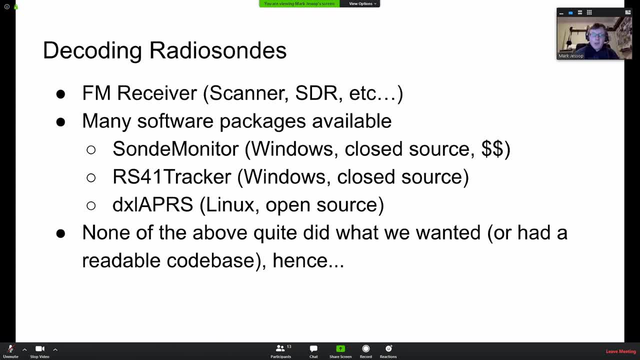 Barossa Valley, So he's here every year. RS-41 tracker is relatively newer and that is specific for RS-41s. It works pretty well. It's got a map. It's quite kind of cool. It's free. It is closed source. You can't go and modify it. There's also 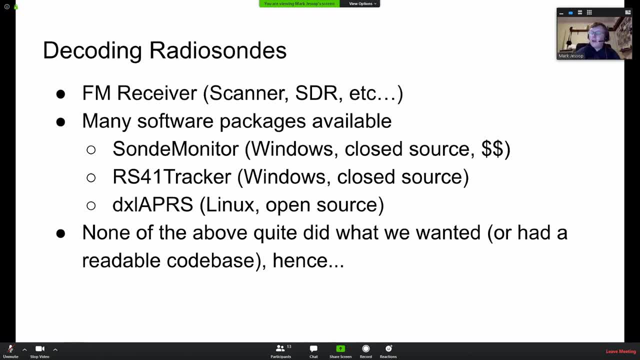 this bit of software called DXL APRS which tracks a few different radio sonde types. It's designed to run on Raspberry Pis as well. It's code base is best described as opaque. It's a little bit hard to work with if you want to modify it. So back when I started this particular hobby, I 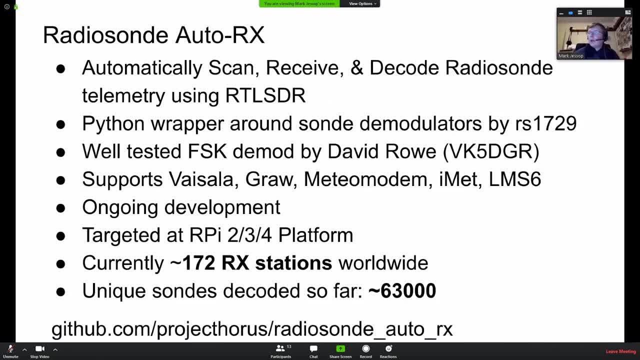 decided I'm going to write my own. So we come to radio sonde auto RX. So the main reason this was written was because back when I started they were launching RS-92s- these songs here- and the frequency would change from launch to launch. Nowadays, 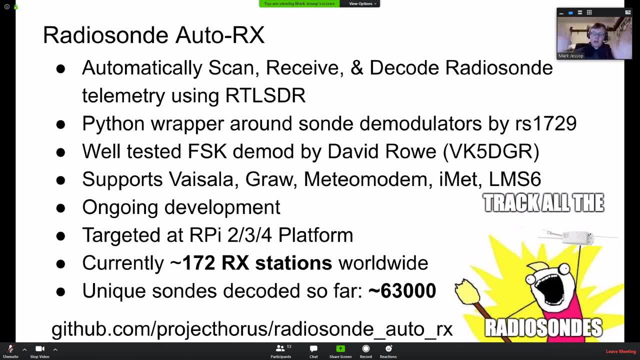 that is running on the same frequency all the time, But back then it would change. Every single launch would be on a different frequency. It was getting very difficult to try and track and decode them, So I wanted a way that I could scan the 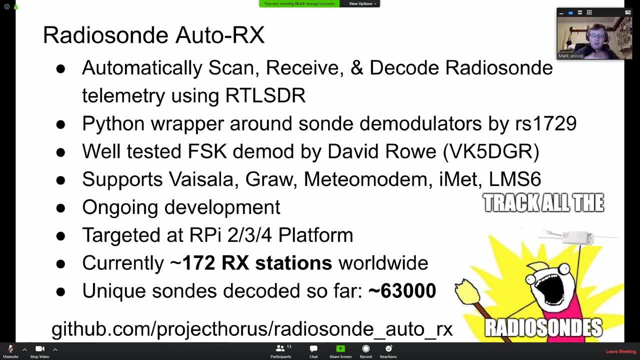 radio sonde frequency range and find and decode them automatically. So I based this around a set of open source decoders written by a guy on github called RS 1729, and I wrote some Python code to automatically scan for the sondes, to decode them and upload the telemetry to the Internet. So at the moment we support 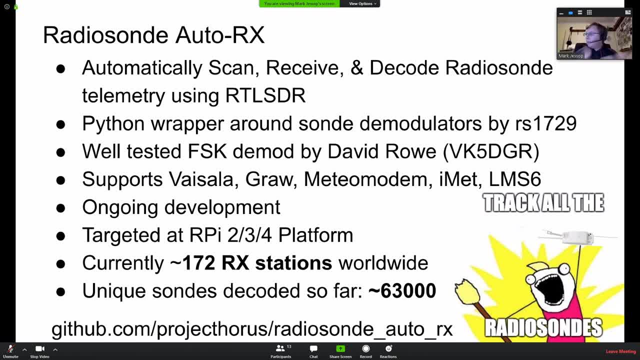 a pretty big range of radio sondes types. So everything that you saw that I showed before, we support those radio sondes. We've had a couple of years now so we're switched in the last year to a very, very high performing frequency shift keying decoder. written. 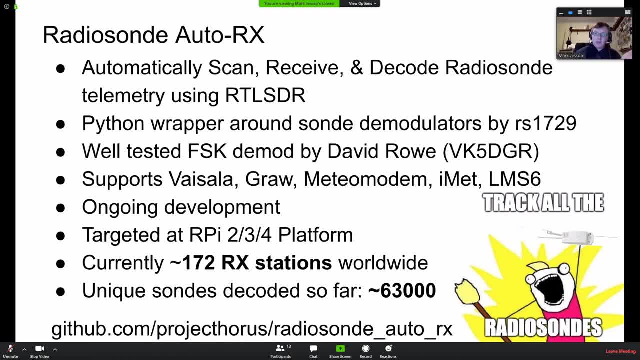 by David Rowe. You may have heard of VK5DGR. He wrote Codec 2 and 3DV. He's a local DSP guru. We're actually working on some improvements right now to this code, So this means that we know the. 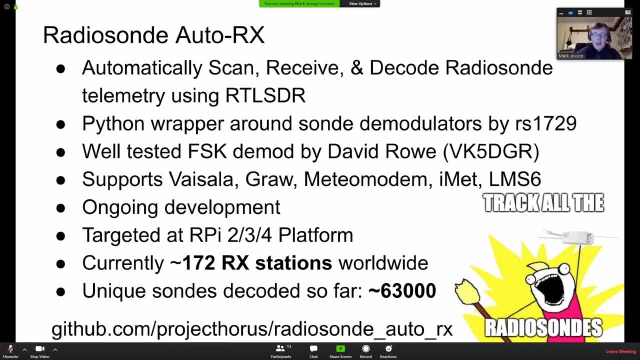 software side of the modem is performing as well as it possibly can be. The RF side is up to you. however, At the bottom of the slide there is a link to the software, and I'll cover a bit more about how to set it up a little bit later on. So when I presented upon this at the beginning of 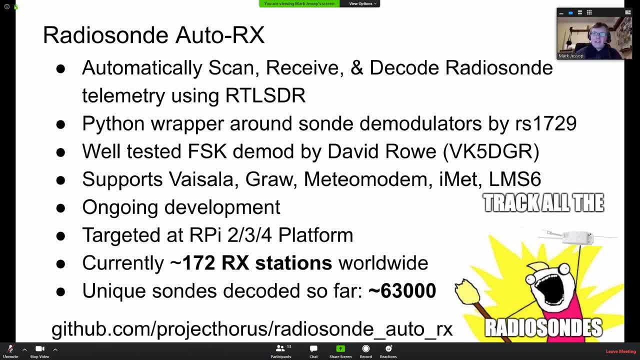 probably about 2019, there were about 60 stations using this software. As of today, there's 172 users worldwide, which kind of freaks me out slightly. And since we started logging Unique Telemetry, we've actually decoded. we, being the AutoRX decoding network has decoded. 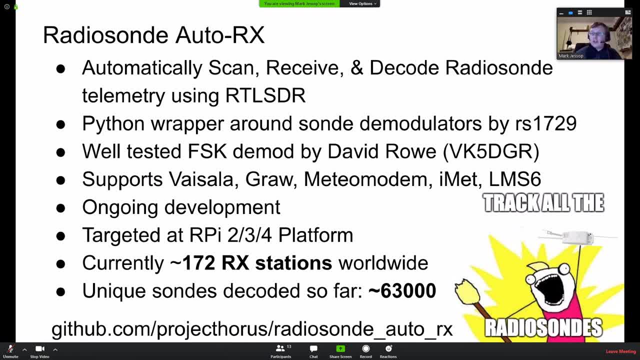 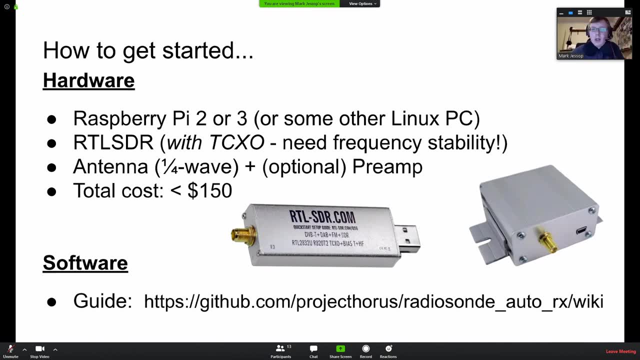 30.. 63 000 unique radio songs. so we're totally meeting the um project aim of tracking all the radio songs, or at least we're getting a long way towards it. so how do we get started? well, um auto rx is designed to run on a raspberry pi and 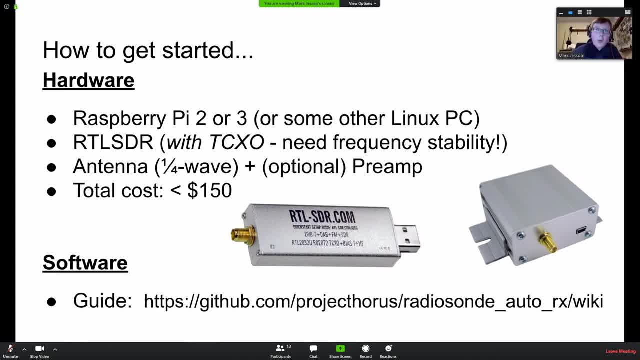 work with a rtl software, defined radio- it's quite possible. you have everything you need to do this in your shack already. so again, you need some kind of linux machine. so raspberry pi is a pretty good candidate for that. you could run it on something else if you. 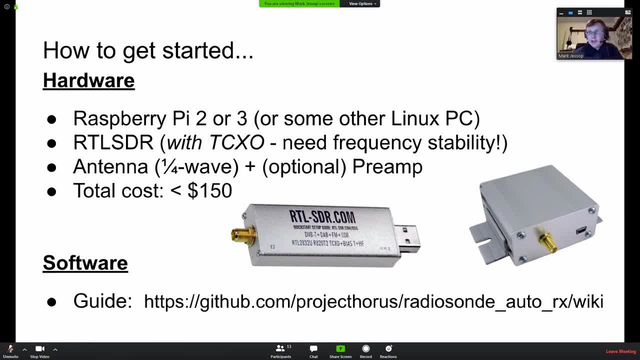 wanted to. you need a software, defined radio, an rtl sdr in particular, and a antenna of some description. we're all hams. we've probably got a 70 centimeter antenna lying around the place. they work pretty well, um, as for the rtl sdr, i recommend the 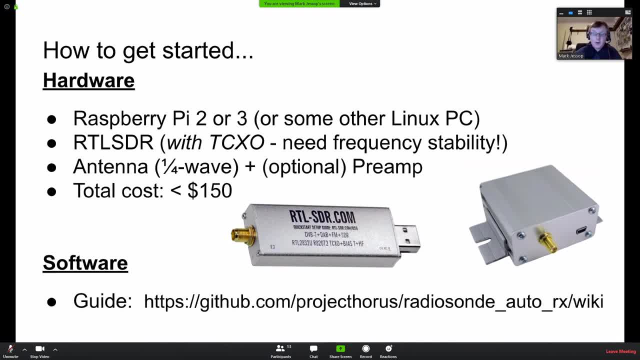 rtl sdr blog- the three sdrs. they're very good, though newelec also do a pretty good version and there's other ones out there as well. the key point is that it should have a temperature compensated crystal. oscillator. frequency is very important into coding these radio songs. a preamplifier is not mandatory. 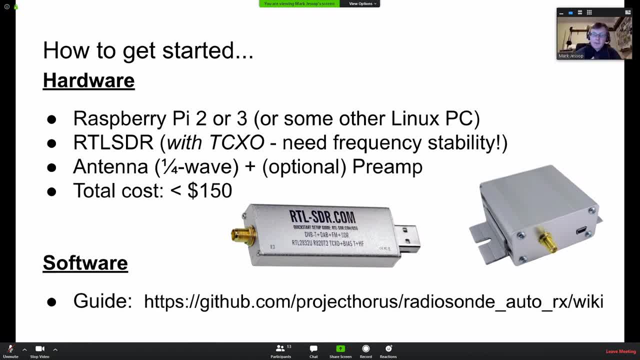 um, you can receive surprisingly well without one, but if you try to track radio songs that might be a long way away from you, then it will help. um, there's a mob called uputronics. uh, thanks for the um. yep, so paul's holding up an rtl sdr. 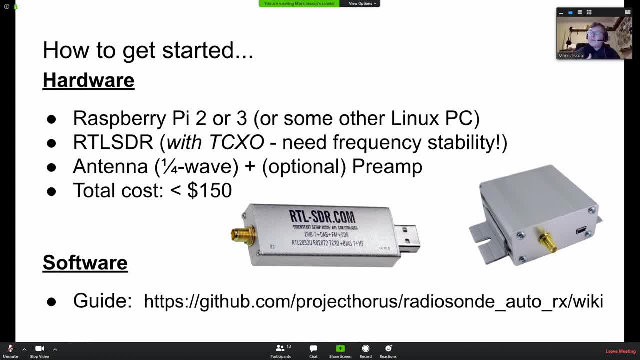 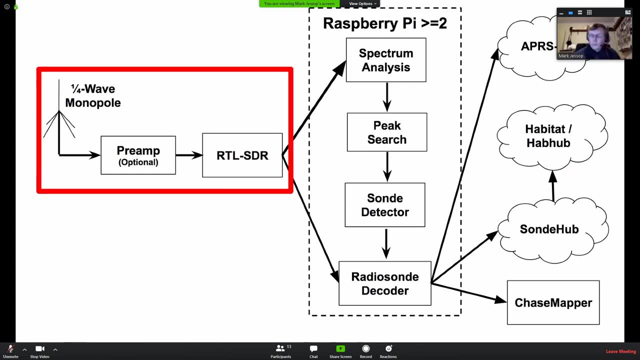 and the uputronics uh sell a very nice preamplifier that has band pass filtering as well, specifically for the radio song band. they work extremely well. um, as mentioned before, all the software is open source available on github and there's a link on the slide on how to get started with the software. 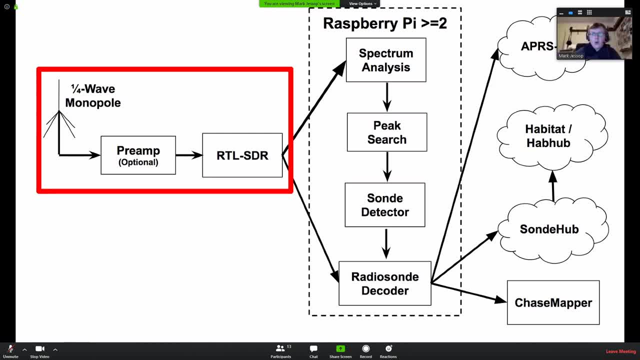 so here's a bit of a flow chart showing how auto rx operates. on the left we have our rf hardware, which captures the radio signal and converts into digital samples which we can then do signal processing on. the first thing that we're going to do is we're going to 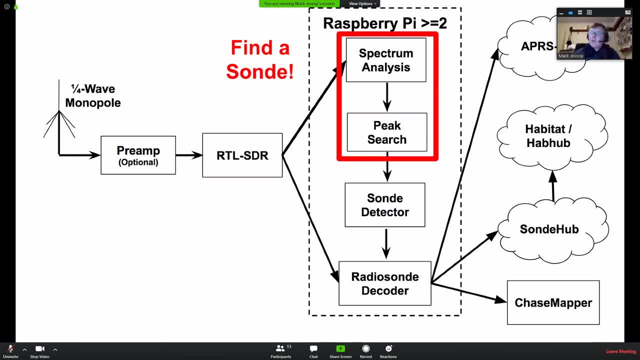 look at some other features as well. so if you look at our rx- uh, a little bit of a different picture here. the rx is sort of more like a. Every radiosonde transmission is unique in some way. They have a particular kind of transmit header. Every sonde has a different one and we can correlate the received signal against a known 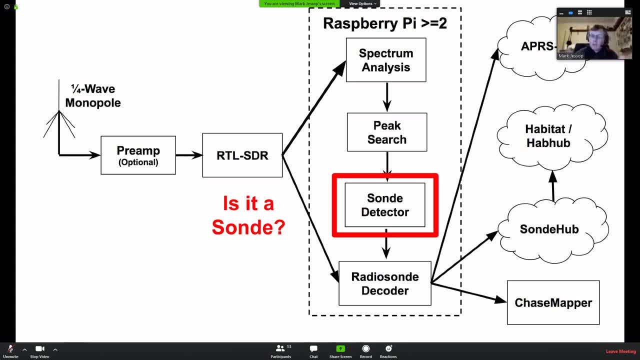 set of headers and we can determine with very good reliability whether we're listening to is a radiosonde and what type of radiosonde it is. Once we know what type of radiosonde it is, we can start decoding it and then upload telemetry. 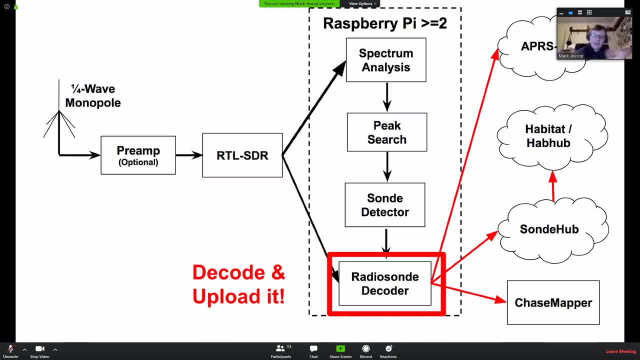 So telemetry can be uploaded to. APRS IS the APRS internet service and you can see it on things like APRSfi. We also have HabHub, the high-altitude balloon tracking website. Now we have SondeHub, which is a proxy in front of that website which does filtering. 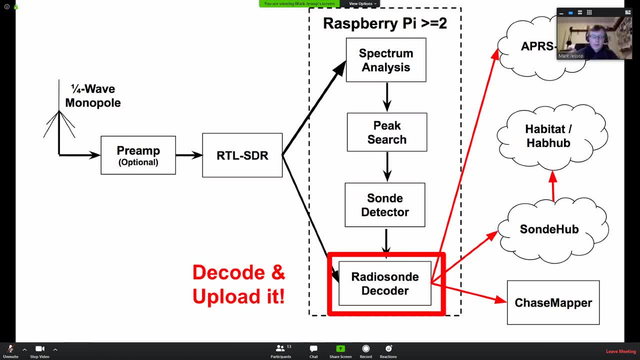 filters out just radiosondes. That's developed by Michael Wheeler, the K3FUR, and we can also send out telemetry to local mapping services like JAN. We also have ChaseMapper, which is a browser-based mapping service, which I'll cover in a bit. 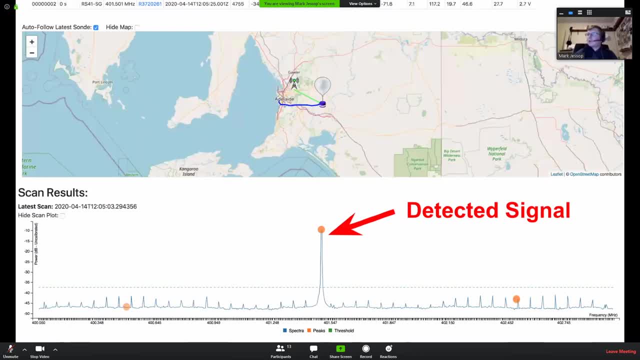 of detail shortly Now. the AutoRx software also provides you with a web interface so you can see what's going on. So here's an example showing the scan results of the spectrum display showing a pretty strong signal right in the center there. 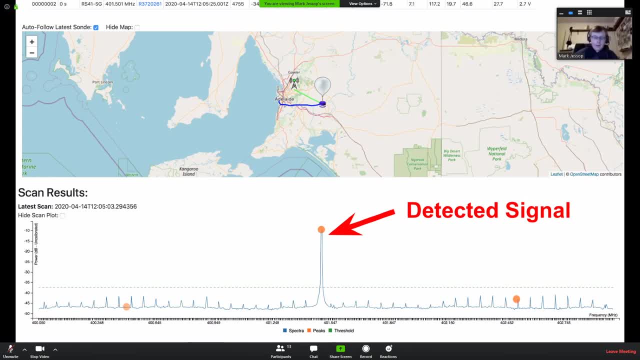 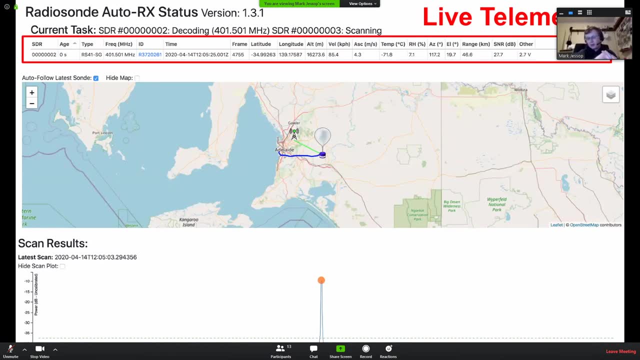 This is our detected radiosonde. Above it, if I scroll up a little bit, we see telemetry data coming from a radiosonde. Now I'd show this live. The radiosonde hasn't launched yet. We want it to launch for about for another, probably half an hour or so. 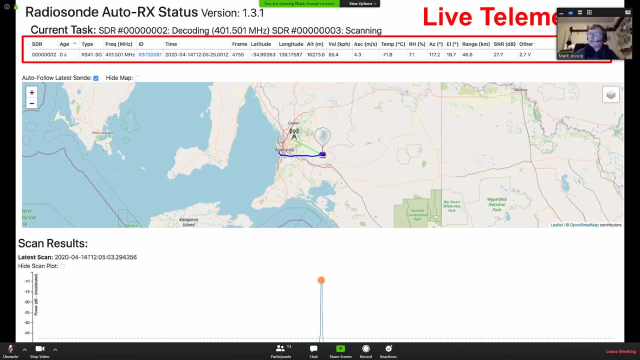 So on the slide there you can see the telemetry data from the radiosonde showing where it is, temperature, humidity, the range to the radiosonde and also the SNR signal to noise ratio of the signal, And in the center of the screen we see a map showing where the radiosonde is and where. 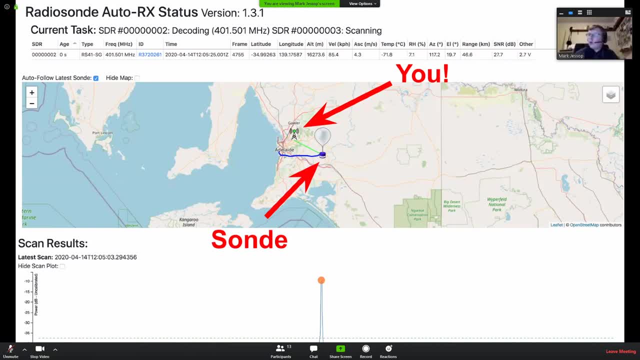 you are. So this is good for just the local display- What is your station doing? But the real power comes when you upload it. So this is the local display. You can upload the data to sondhub or habhub and see it all on that. 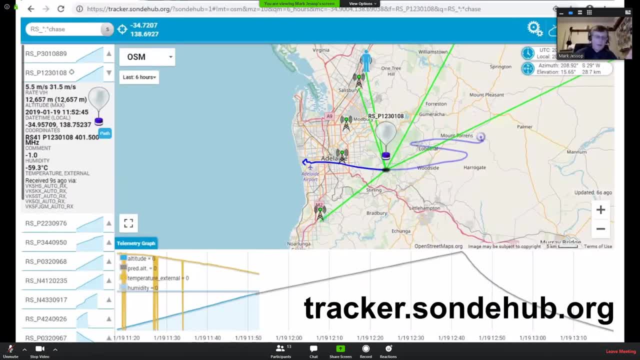 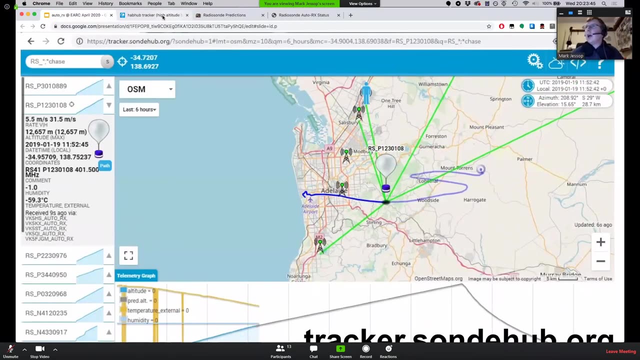 So this is trackersondhuborg. Now I'm just going to drop my screen share momentarily, Actually. so I'm not going to do that, I'm just going to full screen this and show you sondhub live. Sorry to the people that are on the radio, you have to look at the slide. 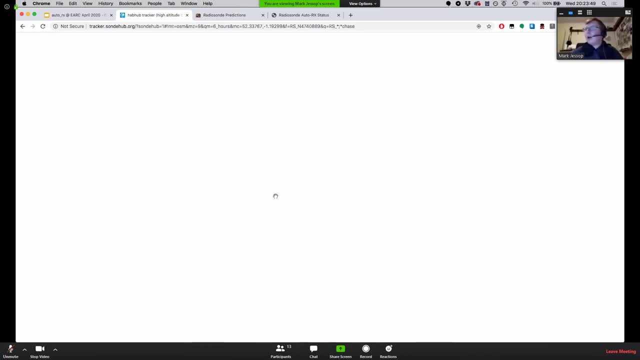 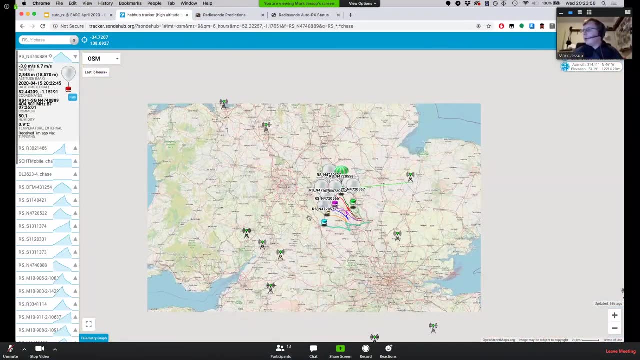 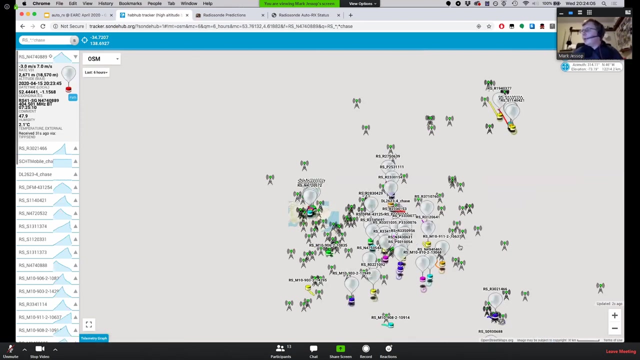 So this is sondhub, Okay, And there are currently quite a few radiosondhub in the air at the moment, And if I just zoom out and show the entire world, come on. well, this is Europe anyway. that will do. 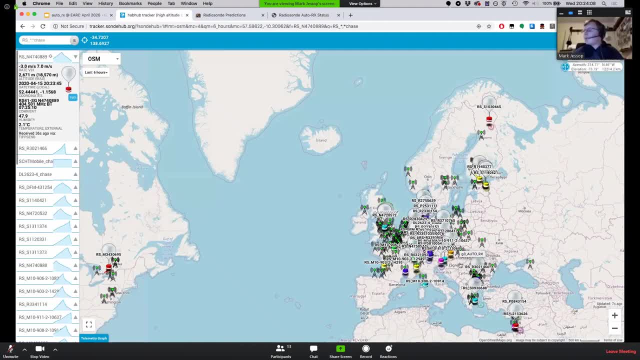 It's a little bit slow at the moment and we can see radiosondhub all over the place. Not all stations launch at those defined times: zero, 12,, et cetera. Some of them launch in between. On the map we can see little antenna icons. 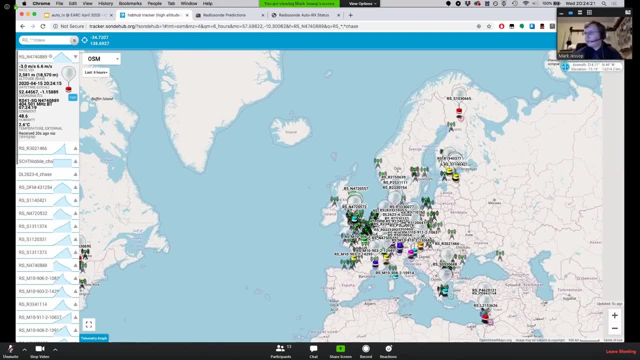 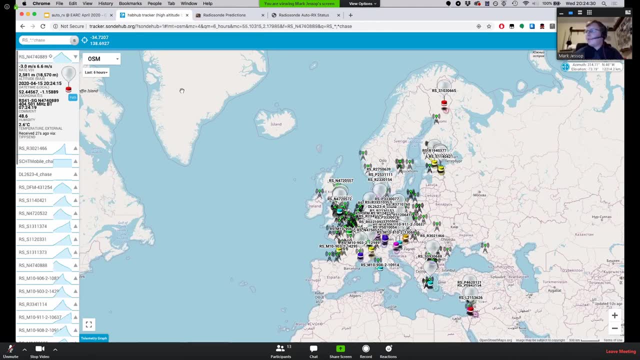 These are all radiosondhuborg. These are all receiving stations. Not all of them are radiosondhub receivers, but many of them are And if we go to Australia we will see there's more than likely no sondhub in the air. 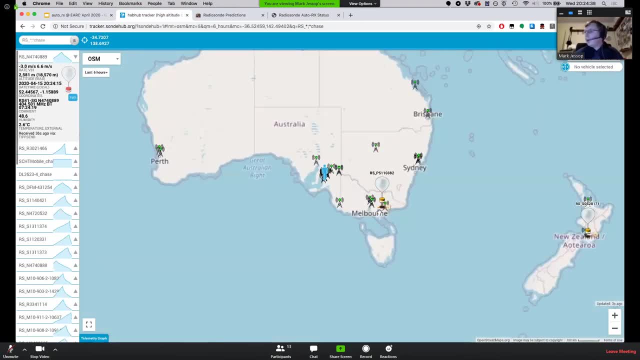 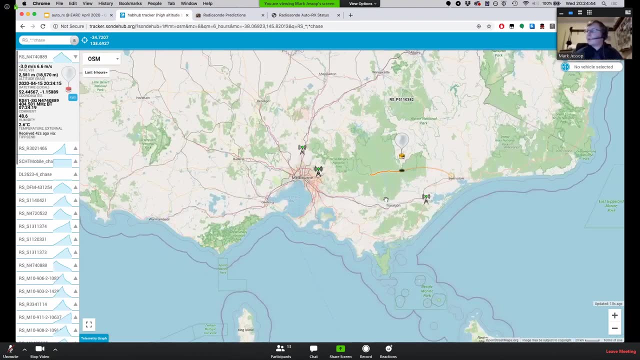 Actually, if we look at Melbourne, what we're actually seeing there is the ozone sondhub. So today, Wednesday, the Bureau of Meteorology launched an ozone sondhub from Broadmeadows in Melbourne. This was the radiosondhub track from Melbourne. 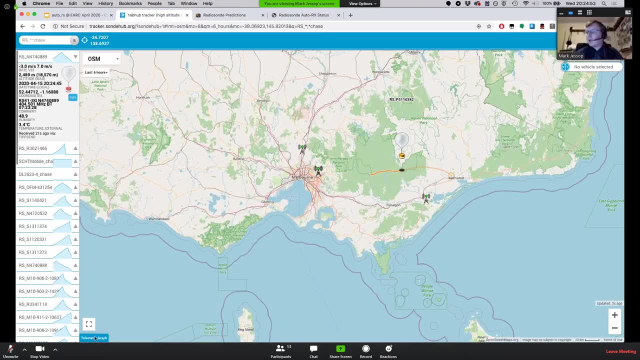 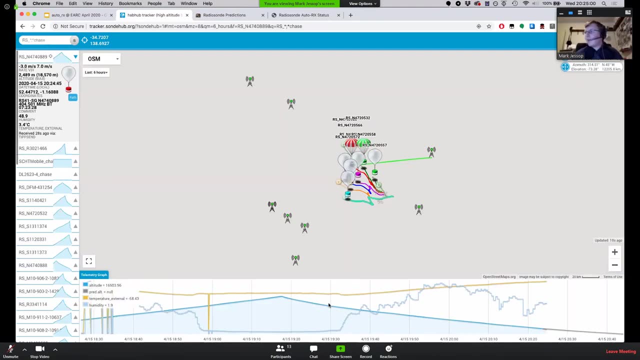 And we can look at telemetry. Okay, And as it's coming in, we can get a plot at the bottom showing the height of the sondhub, the various temperatures and things like that. It's all pretty cool And you can also see who is receiving the signals as well. 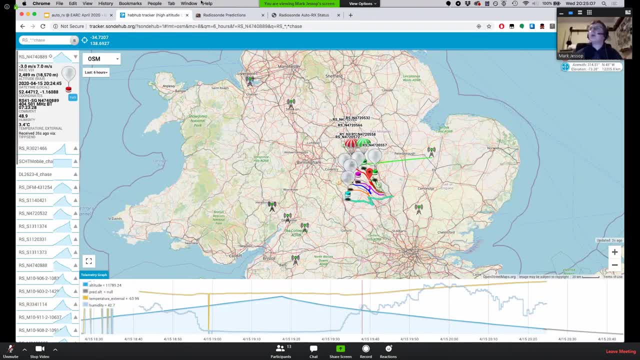 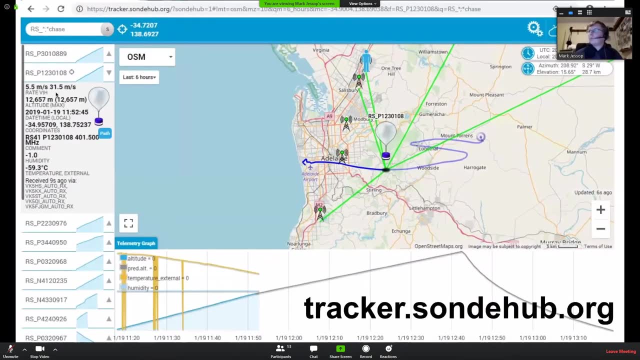 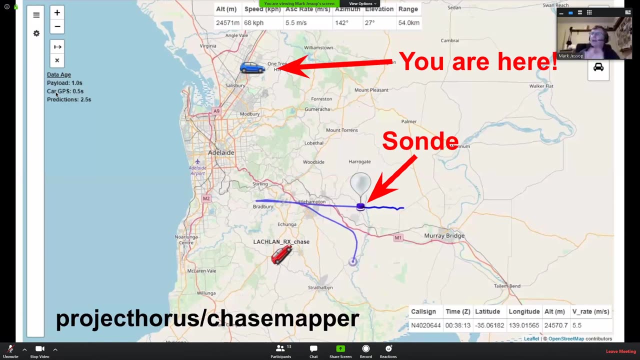 There's a little green line that shows up going to the receiving stations. Let's bring up the slides again. So ChaseMapper. So sondhub is pretty good when you've got access to the internet. If you want to go out and chase the radiosondhub yourself, you might not have net connectivity. 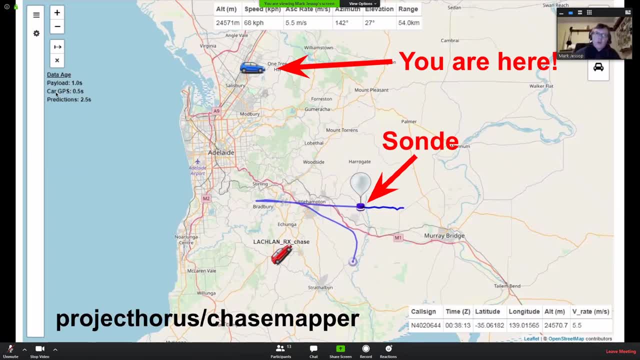 So what do we do at that point? Well, we solved this problem many years ago, So Project Horus has been launching since 2010.. And when we started, we developed a system called Aussie Explorer, And this allowed us. This was based. 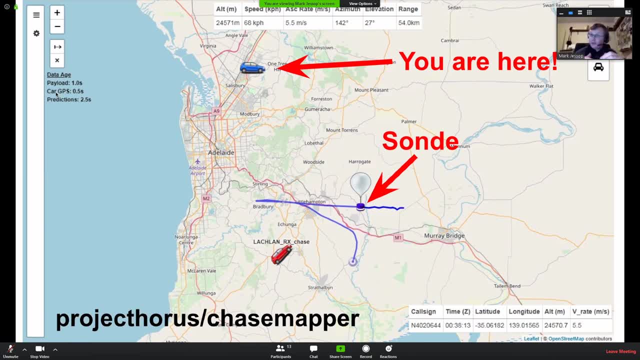 Sorry, Aussie Plotter Sorry- Which was based around a mapping software called Aussie Explorer- Windows only We used topographical maps. It was pretty good. And then we developed a system called Aussie Explorer And we had a completely offline mapping system. 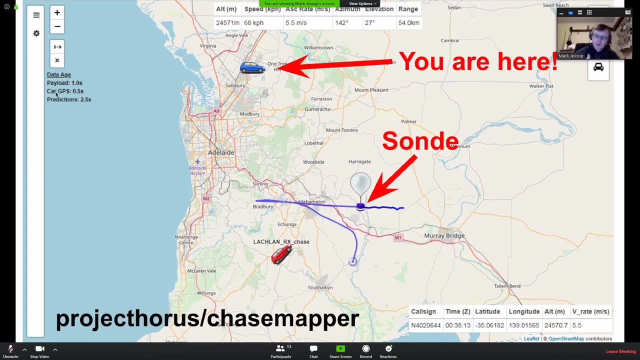 It worked really well. If we had no phone coverage, we still had maps. We would get telemetry. put it on the map, off we go. It being Windows only somewhat annoyed me for a while. Plus, Aussie Explorer was a very old bit of software, even when we started. 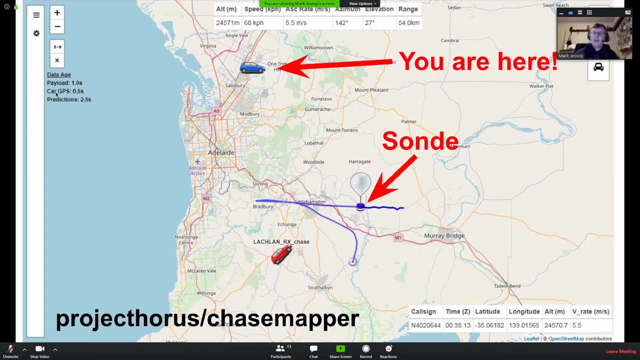 So after doing the AutoRx mapping display, I decided I'll have a crack at writing my own, And that became ChaseMapper, So I wrote this in post. I wrote this in Python using various technologies called Flask and Leaflet for mapping and interfaces. 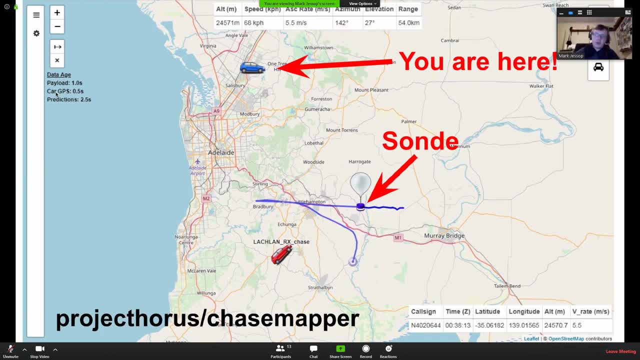 with AutoRx to show the song position on the map. It'll also show positions of other balloon flights, for example, Project Horus launches. Things like that can also be fed into ChaseMapper. You can download weather models. So one thing I didn't quite cover was that all this data these radios want to collect. 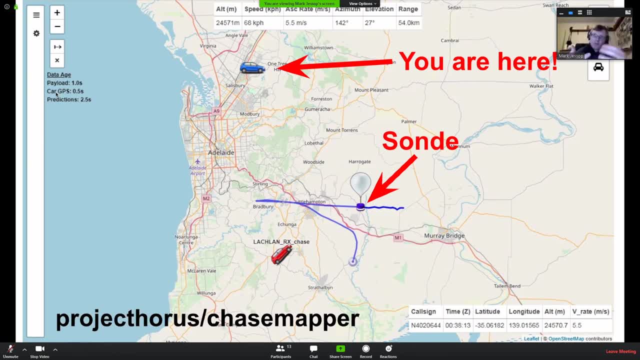 feeds into global weather models. Probably one of the biggest ones is called the Global Forecast. It's a global forecast. We can download that data or portions of it- in the case of what we're doing here- and use it to predict where a balloon is going to travel. 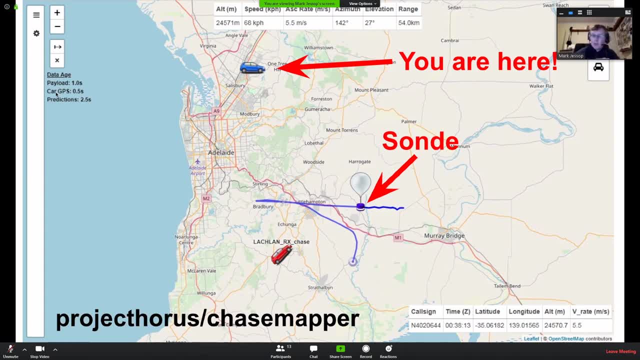 So in the case of on this slide, we can see where the radio sonde is and we can see a blue path hitting in front of the sonde, showing where the sonde is going to travel, or at least where it's predicted to travel. 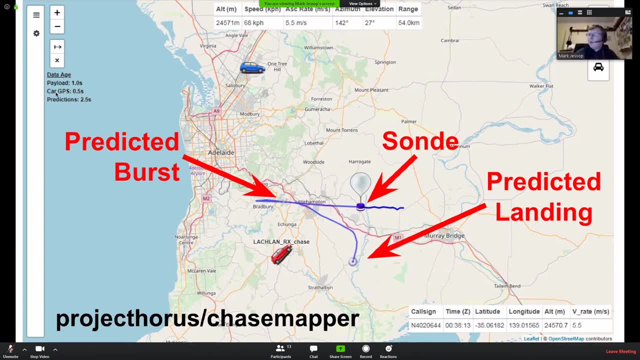 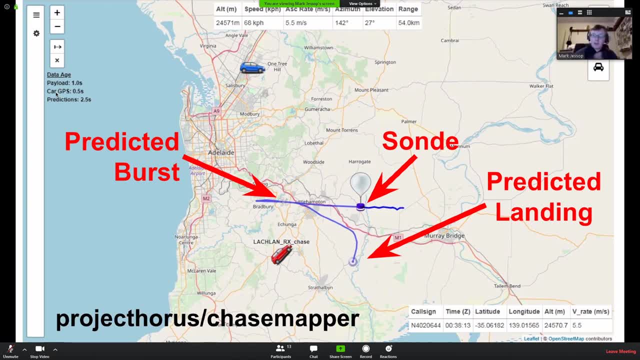 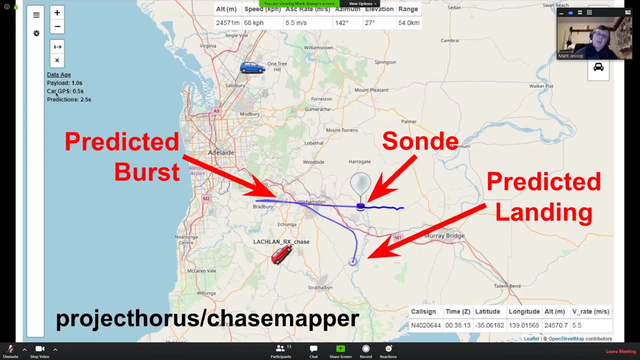 Paul has done that a few times. I've done it quite a few times as well. It's really good fun. Another nice feature which was added in about a year ago was you can share where you are with other users of ChaseMapper and also with your online map. 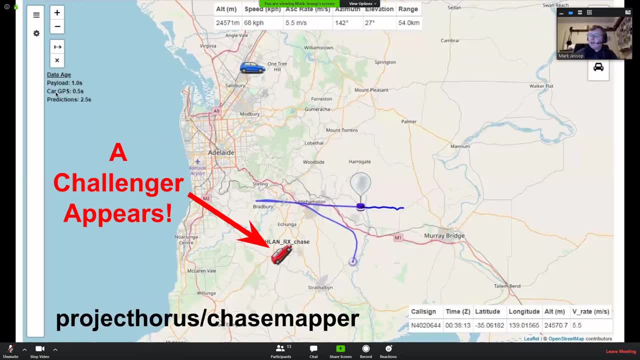 So in this case a challenger appears on the bottom of the map there so I can see when someone else is out chasing as well spectators- you might be watching trackersondhub at home- can see where those people that are out. 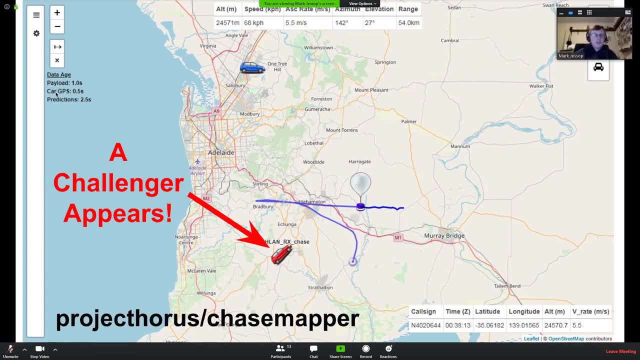 chasing are. It turns radio sonde hunting into a spectator sport. It's good fun And because it got very popular we had to. we got to the point where there were so many radio sonde chasers in Adelaide we had to start a mailing list, The sonde VK5 sonde chasers mailing list, because otherwise 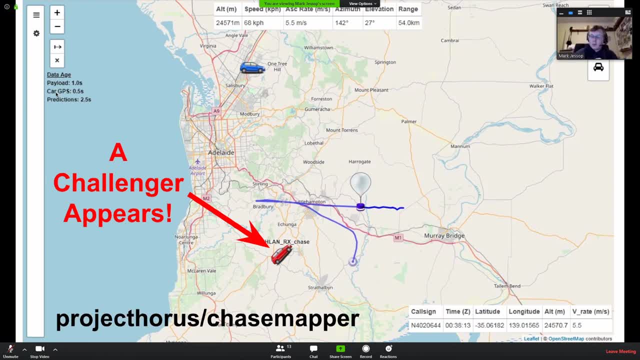 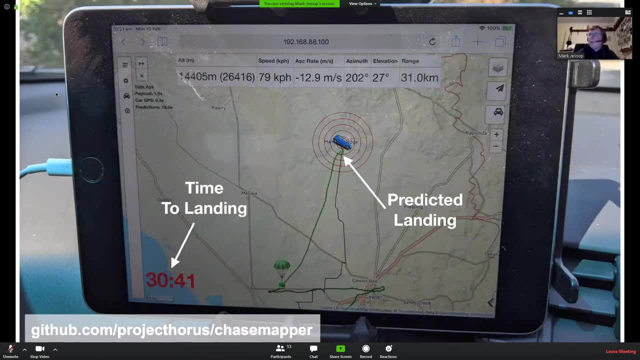 we found sondes were going missing. Still happens occasionally, but it's pretty good nowadays. So this is an example of ChaseMapper being displayed on a tablet in my car. So, just as a point of note, ChaseMapper actually runs on the same Raspberry Pi as AutoRx- or it's designed to anyway, and you access it via a. 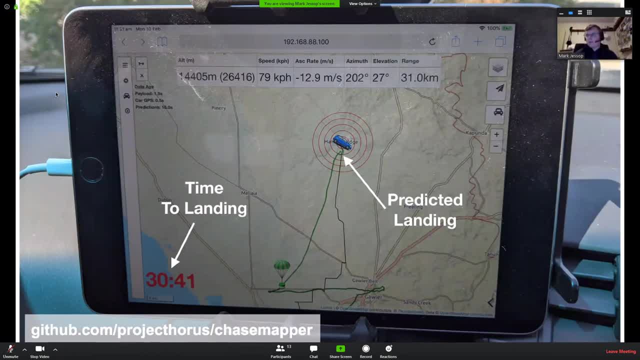 web browser on a tablet, on your phone, on a laptop, doesn't matter. In this case, I use a mobile phone, which is a mobile phone, but it's a mobile phone. It's a mobile phone. it's an iPad mini on the dashboard of my car And I just have this running throughout the chase. I 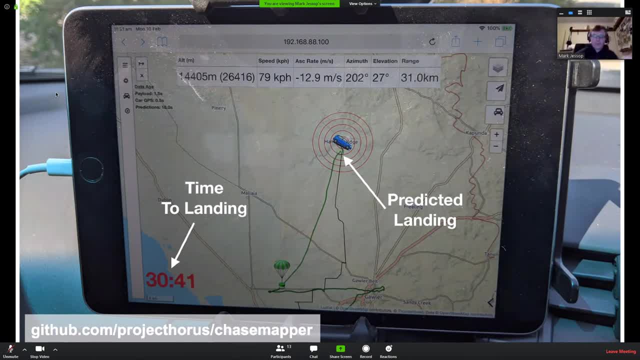 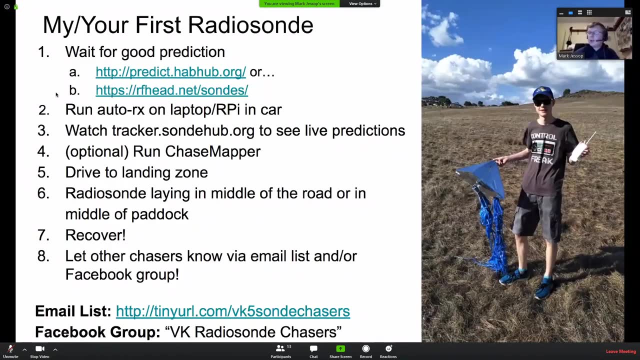 can see where the sonde's going, where I should be driving to. Of course, I'm looking at the road, not at my iPad while I'm driving. So how do you do your first radio sonde chase? Well, first up. 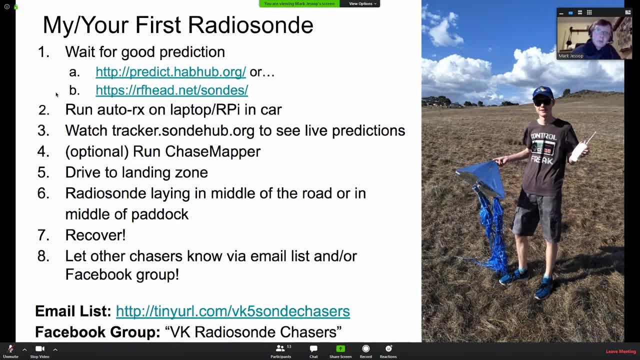 you want to make sure that the radio sonde launch is actually going to be recoverable in the first place, And we can use those weather models to do predictions. to find that out, There's a website, predicthubhuborg, which lets you just generically specify a launch location. 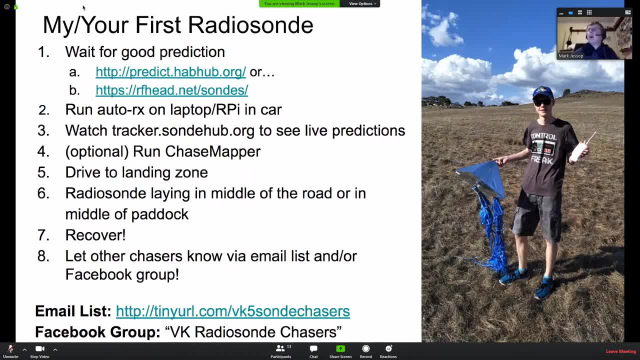 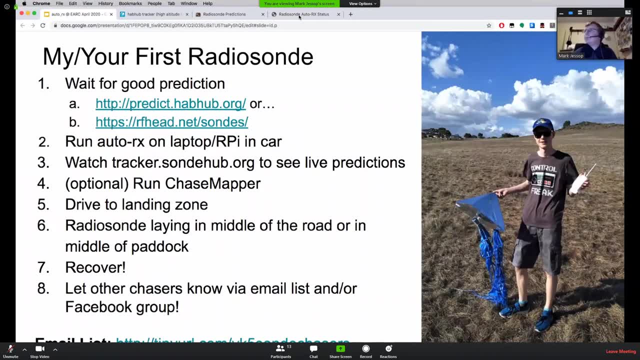 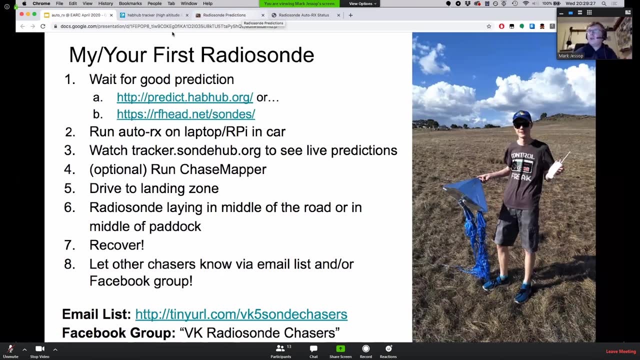 and run predictions For Australia. I've got my own website And if I just go to that- and again, apologies to people on the radio, I have the oops- I'll go to the main website first. So rfheadnet forward slash sondes And this has a list of launch sites. 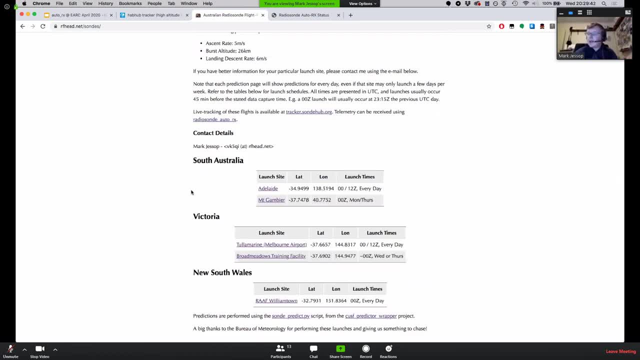 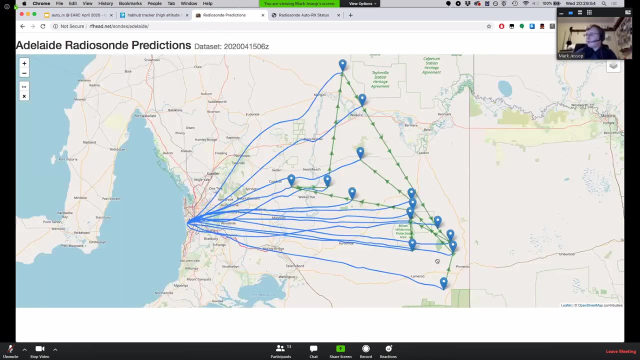 which I'm currently running predictions for a couple in SA, a couple in Victoria and also Williamstown in New South Wales, And you can choose the launch site and you can see predictions for the following week. So in this case, the launch tonight, launching in all of 15 minutes, is heading out. 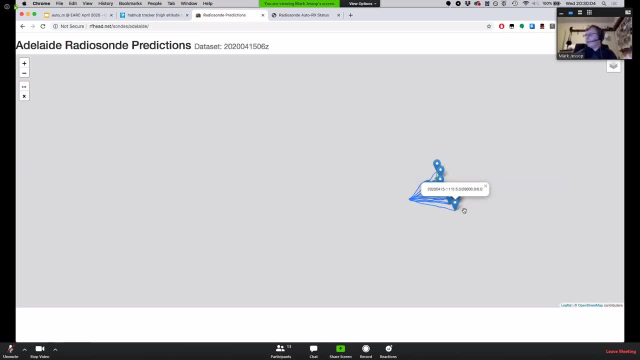 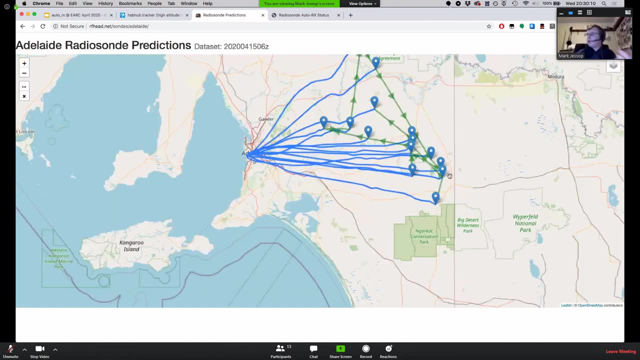 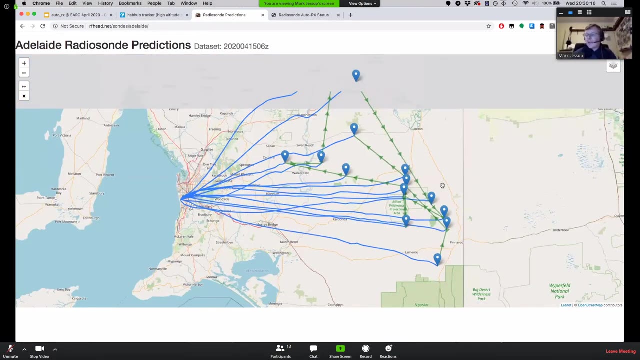 almost to the border near Corunda And that is zoomed out way too far. There we go, And the green line it shows where the landing site is moving over the next few days And from this I would say that for the next couple of days I'm not going to bother going. 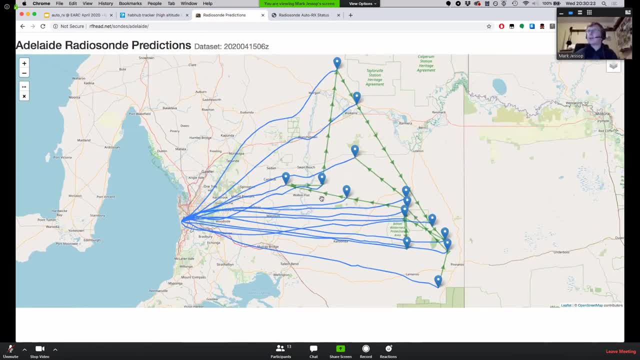 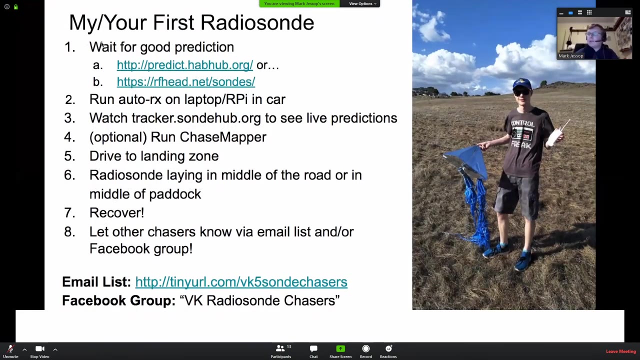 radio song chasing. That's far too long a drive for my wife. So, yeah, you can figure out whether it's worth going hunting for a radio song. So what do we do next? Well, you can just use the online mapping system and hope that someone receives the radio song down. 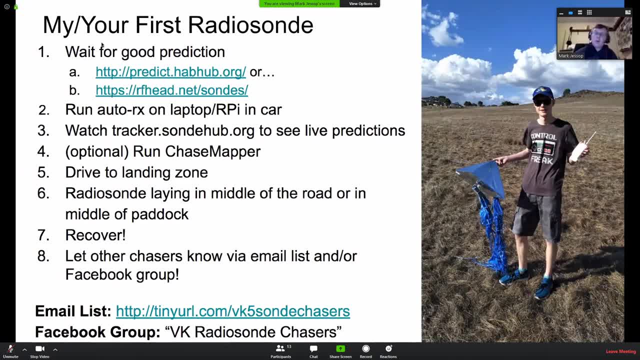 the ground and you can go and grab it, But you're probably better off running AutoRx on a laptop or on a Raspberry Pi in your car. It would help to have some kind of internet connectivity to do so. You can look online to look at the live predictions while you're out driving. 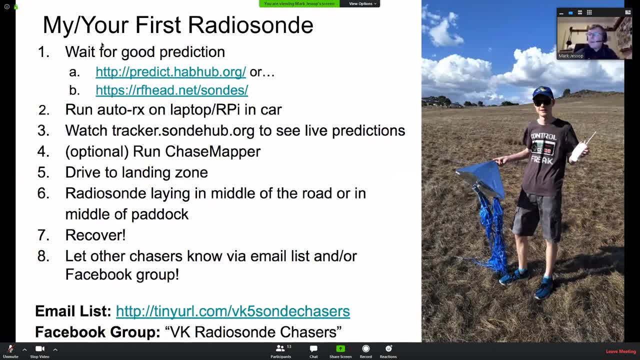 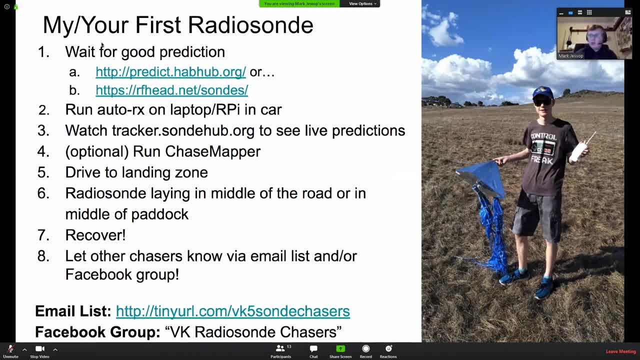 Well, once it all learns up, you drive out the landing zone, you drive around for a while, you follow the predicted landing location and, with any luck, the radio song will be landing or lands in the middle of a paddock or in the middle of a road, or hopefully not on someone's roof, but it does happen. 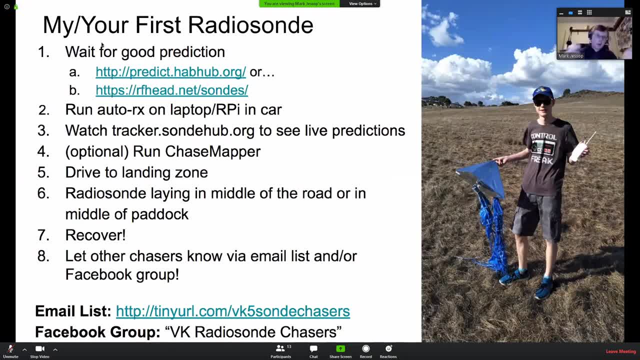 And you can go and recover it, after talking to the landowner, of course, to get permission. Once you've recovered it, you post on Facebook, you post on Twitter, you post on the mailing list to say I've recovered the radio song. 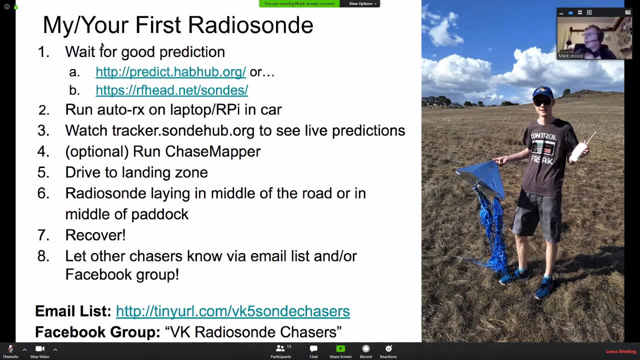 All is good. You can now go home and reuse the radio song for whatever you want. So, yeah, there's an email list for VK5, so VK5 Song Chasers, There's also a VK Radio Song Chasers Facebook group, which is worth posting on. 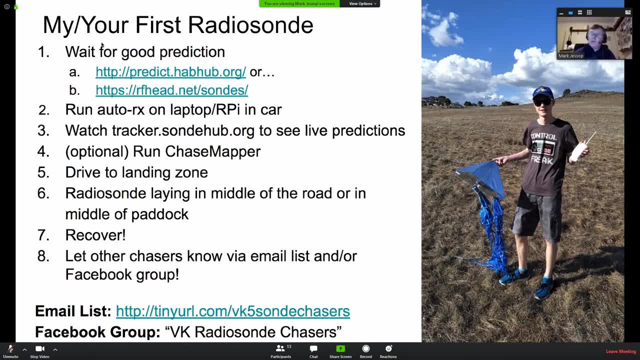 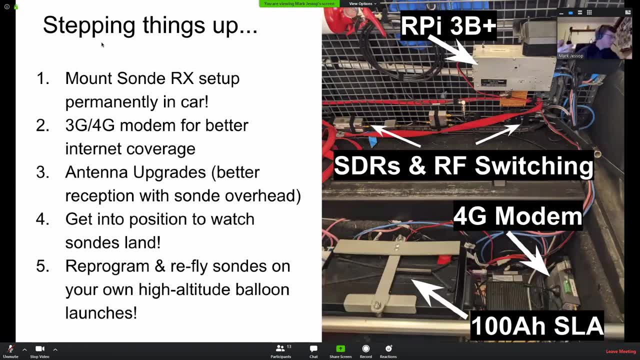 So, yeah, definitely use these systems to let other people know if you're out balloon chasing. How do we step things up from here? This is VK5 Quebec, India. This is VK5 Quebec, India. Well, this is the back of my car. 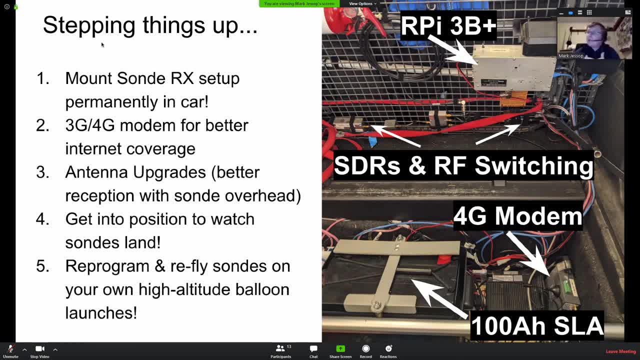 So I have a Raspberry Pi mounted permanently in the back of my car. I've got a 4G modem with an external antenna to get better internet coverage when I'm out and about. I've got a couple of different antennas which I use for doing radio song chasing. 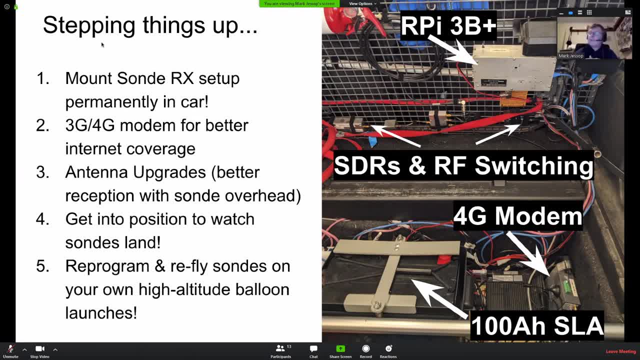 Now, those antennas were designed for Project Horus balloon flights, but they work pretty well for songs. Normally, I'll use a vertical antenna. This works well when the radio song is low to the horizon. I also have a turnstile which is designed to look upwards. 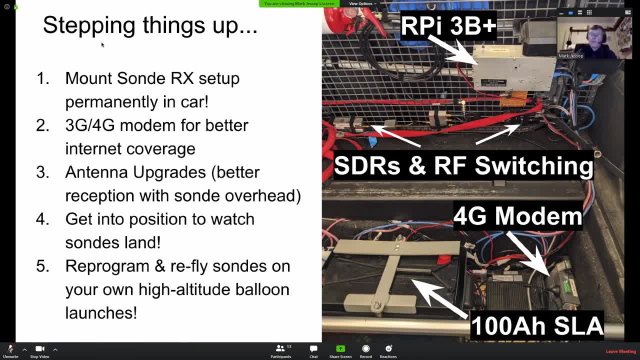 So when the radio song is directly above your car, often the vertical antenna won't work so well. You'll be in a null of the antenna pattern of the song and the song will be in the null of your antenna pattern as well. The turnstile works brilliantly in that particular situation. 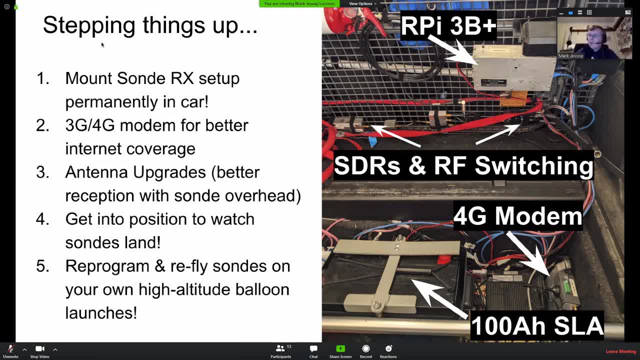 After you get good at this and do a couple of radio songs, radio song chasers, eventually you end up seeing them land And I know Paul's done this a few times. He's had the chance to see a couple of radio songs land. It's pretty good. 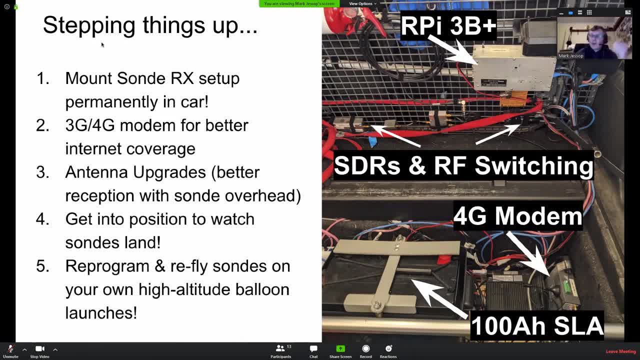 It's even better if you watch it launch at the airport and then drive to the landing site and watch it land. That's very, very, very cool. And then, of course, finally, once you've got a stack of these things, 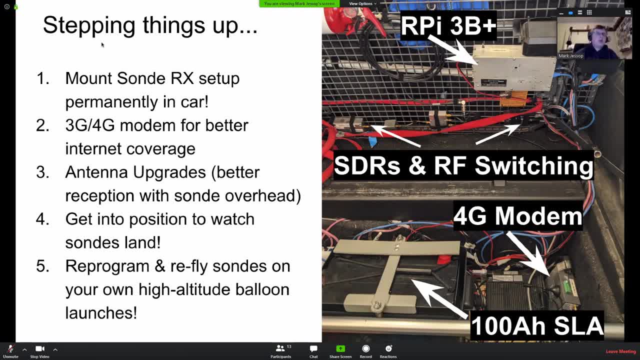 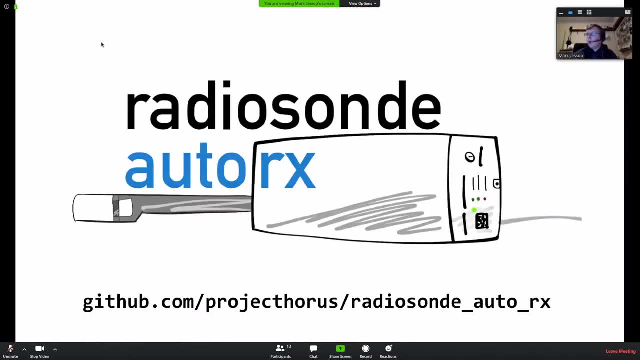 you can start reusing them. You could even do your own balloon launches. So these RS-41 radio songs are excellent for balloon tracking. They're lightweight. A couple of AA batteries Works really well, So That's pretty much all I have. 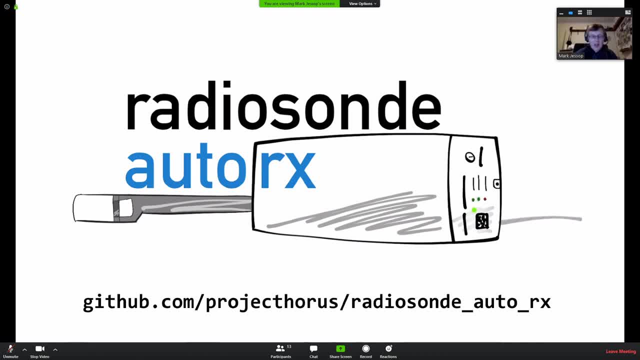 So I'm going to open it up for questions. If you could type in the chat window or raise your hand- and I'm happy to take questions at this point- Or on the repeater, for those that are sitting on the repeater as well. 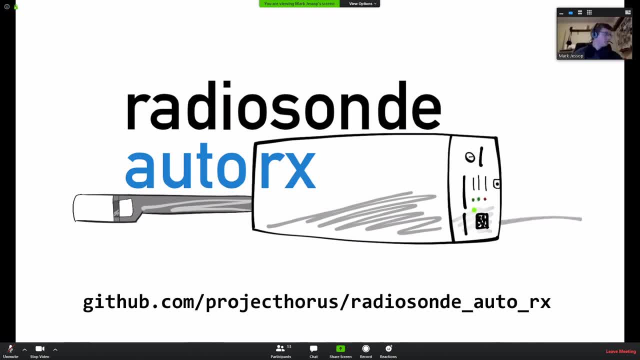 Okay, Five two one. Okay, Five two one. VK5QI, VK5ZD, VK5ZD. Are you going in? VK5QI? Okay, I don't know whether you can hear me via this repeater instead of the laptop. 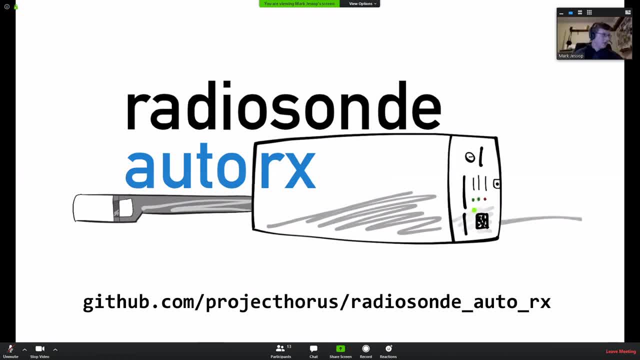 I'm getting feedback. Hang on, All right, Just go ahead, Ian. Okay, Quick question. You talked about the need for stability frequency-wise in the SDR receiver. Your software is smart enough to go and find this on, Can it not just track it? 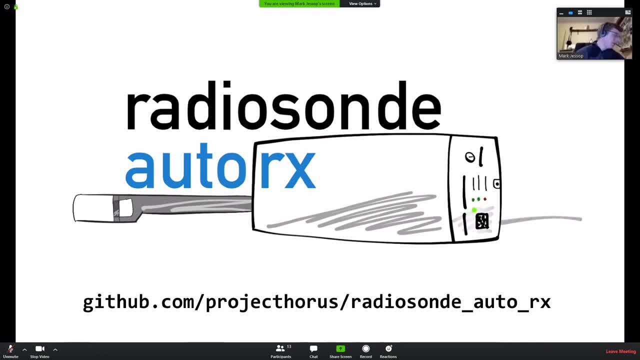 Can it track it as well if it drifts? Okay, So Ian's question there was regarding frequency stability and the point of if I can find the SOND, can I just track it as well? And the answer is yes, actually It works just fine. 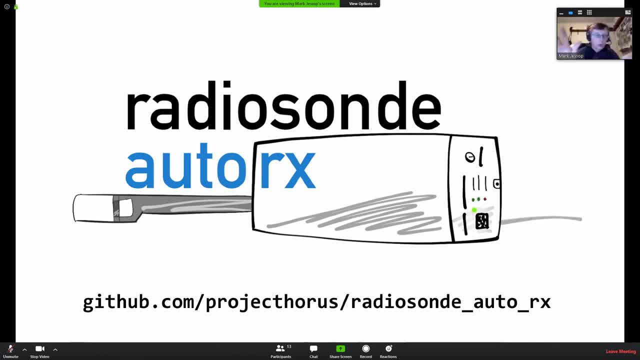 If you're using the well, the more recent versions of the software will quite happily track radio SONDs as they drift around. It is nice to have a receiver which is roughly on frequency. The reason being is the received frequency is actually reported up to the website as well, and 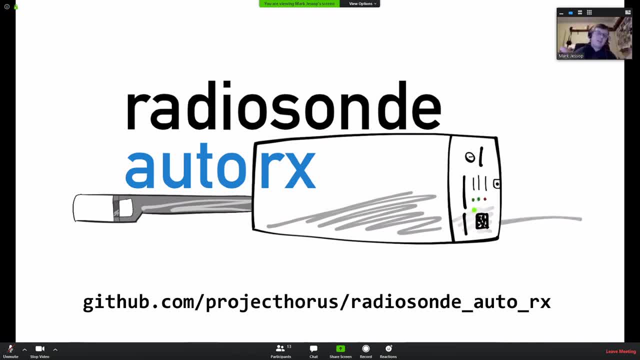 it's nice for other people to see a frequency which actually makes sense and isn't like 20 kilohertz of frequency. So does that answer your question there, Ian? No worries, does anyone else got any other questions for me? Nope, nothing else. Well, thank you for. 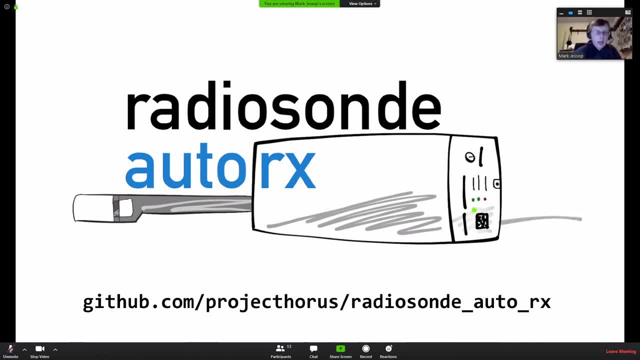 listening. It ran a bit shorter than I expected, but that's pretty good. I guess I'll hand it back to Paul to wrap up, unless anyone else has other questions. So, Paul, you're currently unmuted. Well, thank you very much. Thank you. 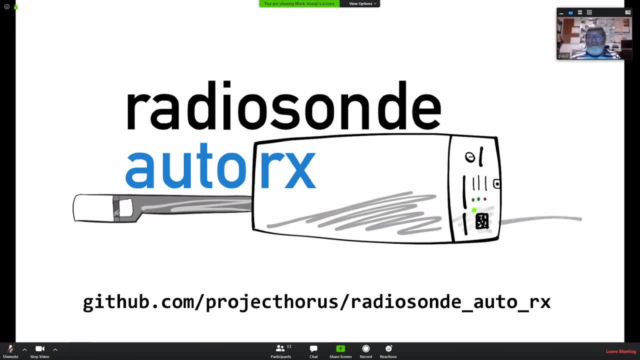 Back to you. Okay, I've got a few questions before you go. What's the closest you've ever managed to get to one coming down? I've been within 50 meters. that's about as close as I've ever got About that far. 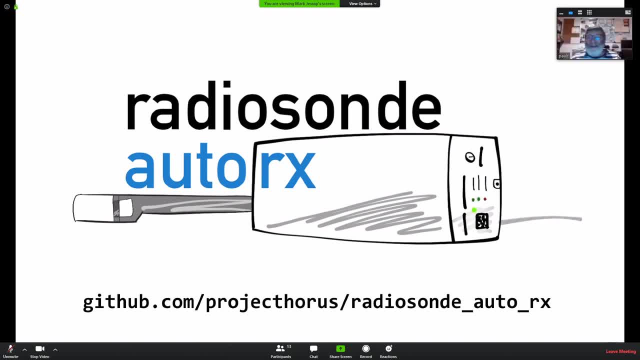 Yeah, you didn't catch it, though Didn't catch it. landed directly in front of me, Landed directly in front of my car. I should say I really wish I had my dash cam. Sorry, I should get back on the repeater there as well. Paul asked: how close have I been? 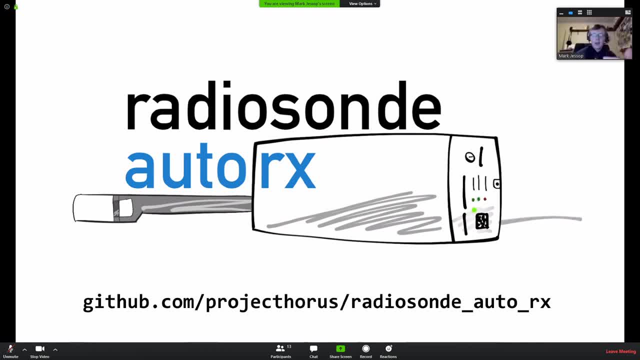 to one coming down. The answer was one landing directly in front of my car and I. it basically made me go by a dash cam, because if I had a dash cam I would have caught it on video. Yeah, and I'd take it. you've got a few on video coming down. I've tried, but I've never had much. 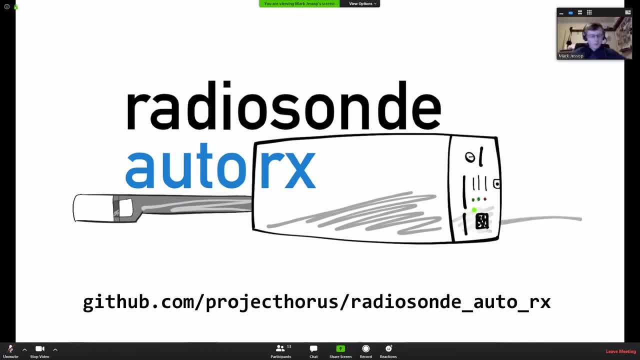 success. So Paul asked: have I got any on video? Not many, actually. um often they're too far away and yeah, I might have video but the video is terrible quality So it really hasn't been worth putting in video, the video anywhere. And another question: are there any binaries for converting? 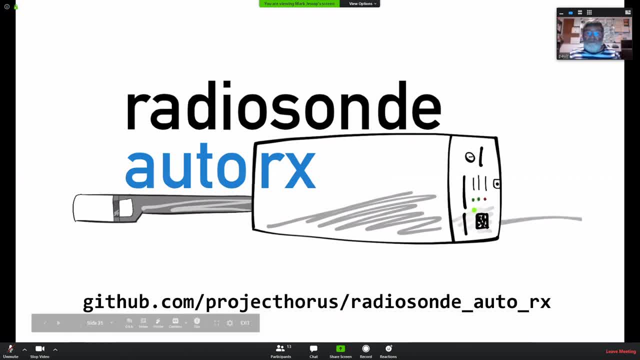 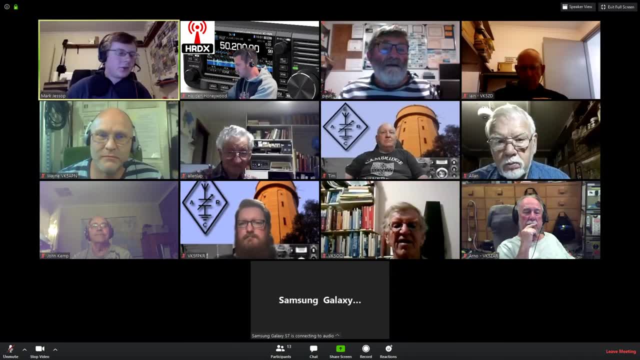 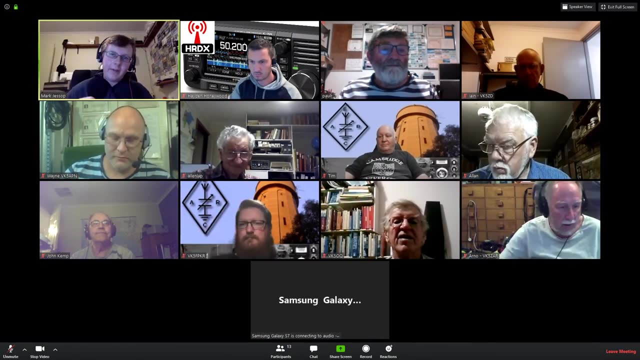 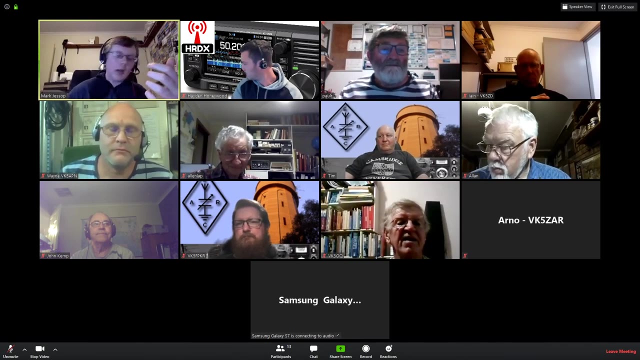 one of these to an APRS transmitter, Go back to stop the screen sharing. So in terms of firmware, there is firmware to do APRS only on the 70 centimeter band, whereas at least the radio chip only goes to the 70 centimeter band. So, yeah, you could do APRS off of them if there. 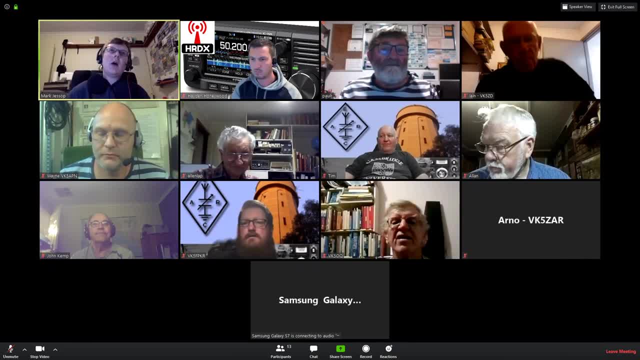 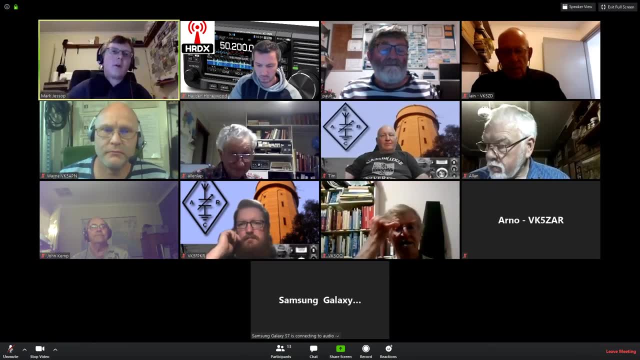 was an APRS network for that frequency. Don't forget that they're only put out about 50 milliwatts. When you use APRS, which is AFSK, you're throwing away approximately 8 dB of power from the double modulations the FSK on FM It's. 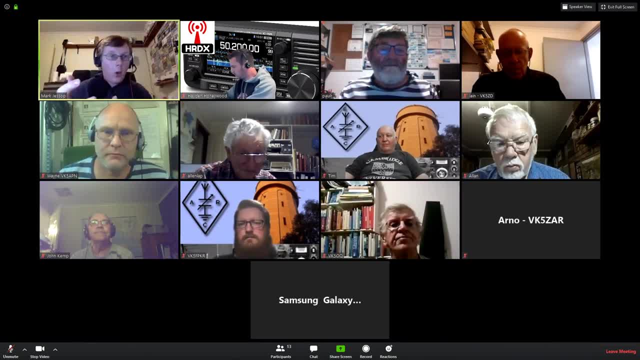 not very efficient as it is and we have to throw quite a few watts of power at it on two meters for it to work reliably. So if you're using an APRS transmitter, it's not very efficient as it is and we have to throw quite a few watts of power at it on two meters for it to work reliably. 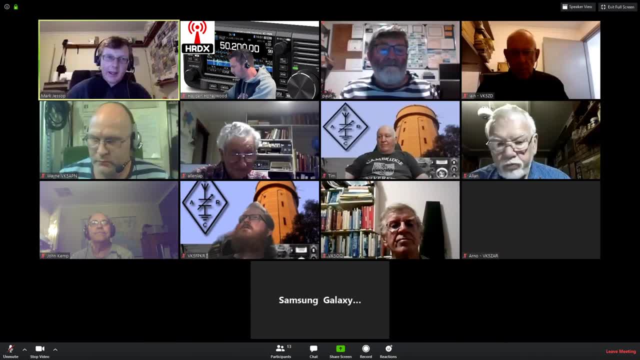 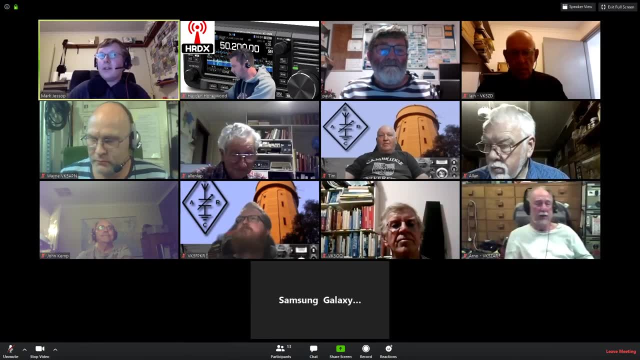 On 70 centimeters, that's the case even more. So yes, you can totally do it. There's firmware out there to do it. I wouldn't really recommend it. There's better options out there. Okay, that answers that one. We were thinking of a. 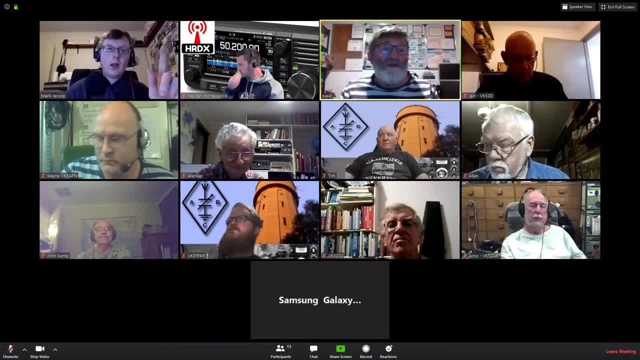 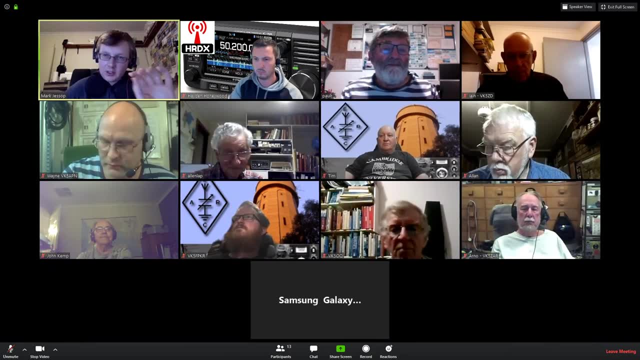 club project using them, but it's probably not going to be that practical unless we just use it for walking groups or something like that. So I think what you're talking about. so this is something that Tim was working on and Tim can pipe up here. I'm just gonna- oh, let me just 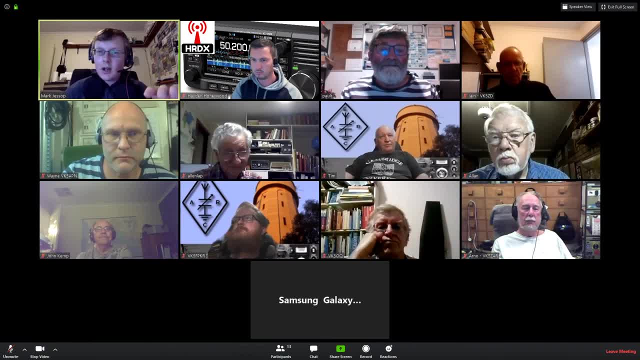 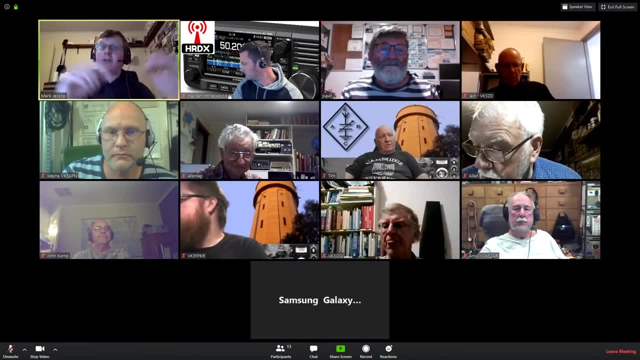 get the chat window. Sorry there, Hayden, I'll get to that question in just a second. So I know what Tim was doing was actually taking the audio out of the transmitter and using that on a different transmitter, So, for example, generating the audio on the RS-41 and then feeding a two meter transmitter. Now 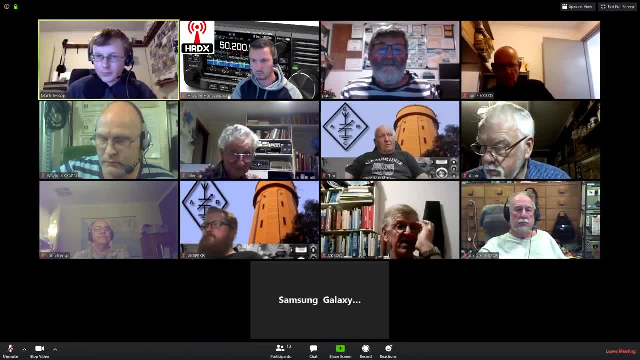 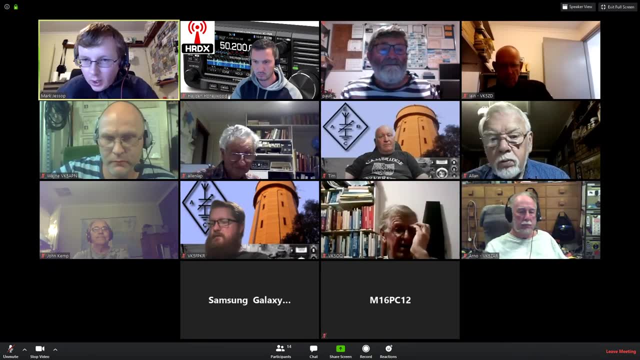 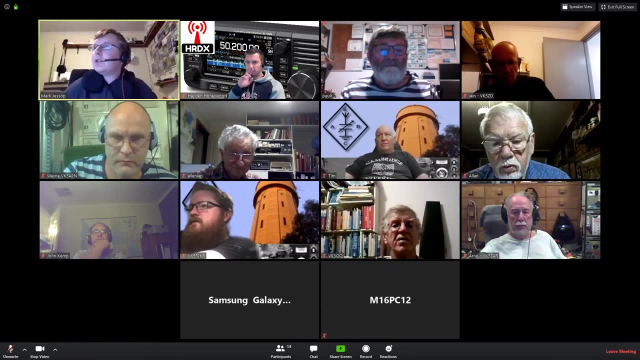 that would be totally possible to do. That's a different option. So I've got a couple questions from online. Can you get raw data from a Radiosonde in real time in a readable format such as CSV? Yes, you totally can, So AutoRx will dump. 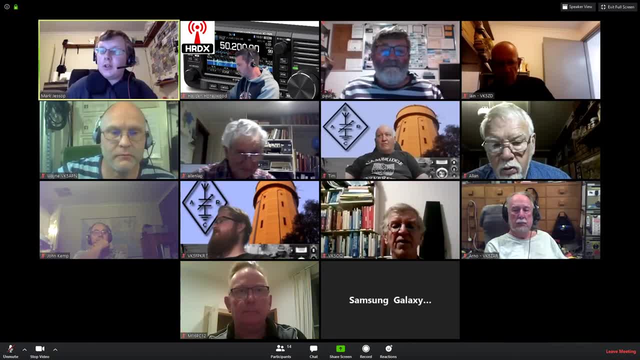 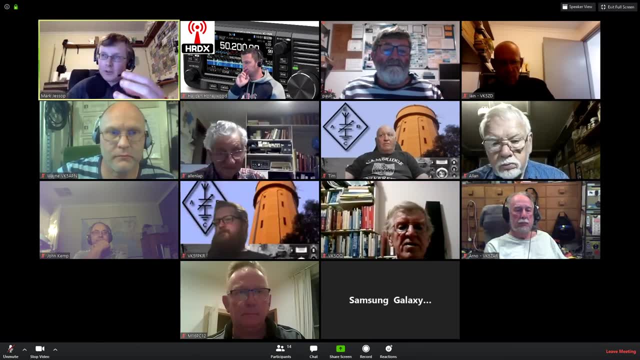 data to disk in real time in CSV. You can also get all the telemetry live via a couple of interfaces that I've written, one of which is used to do the mapping, but you can also get humidity and temperature at the same time. After the: 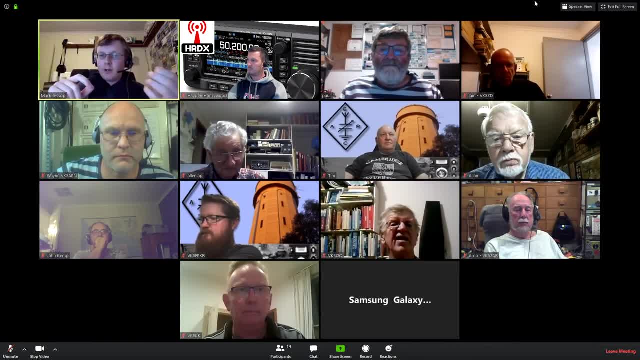 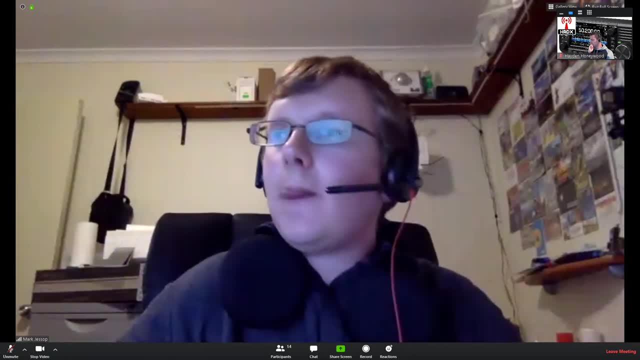 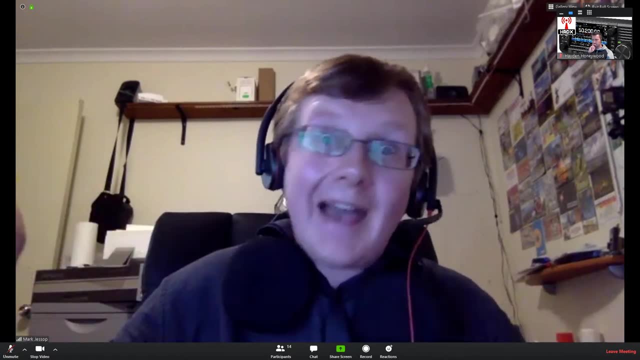 sonde has balanced flight. there's a script which you can run which will do the mapping. So if you want to get data from other launch sites, if you want to get data from other launch sites, email me vk5qi at rfheadnet. We have an interface which is 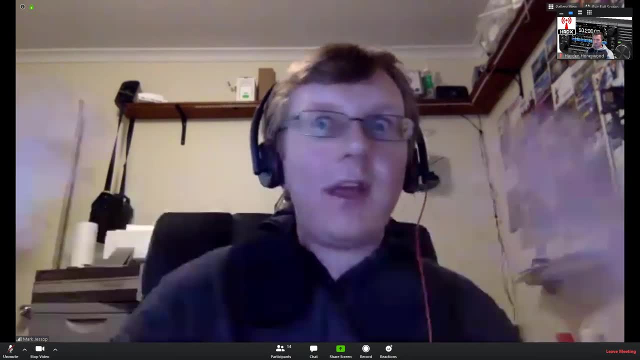 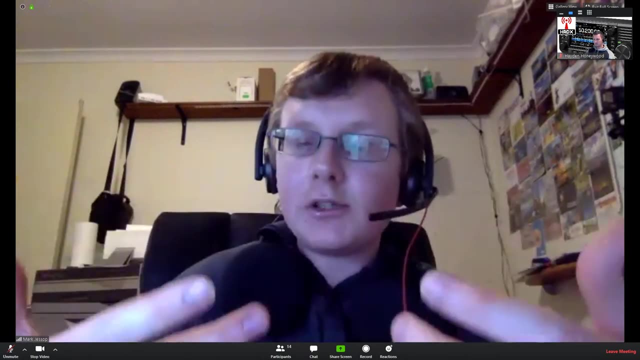 designed specifically to give you all this telemetry of every single launch site all at once, essentially all live. So if you want to start doing some real data processing with the data, it's totally there to do that. So hopefully that answers the question there From a 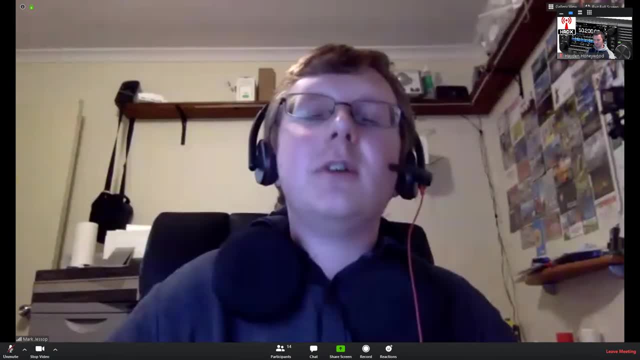 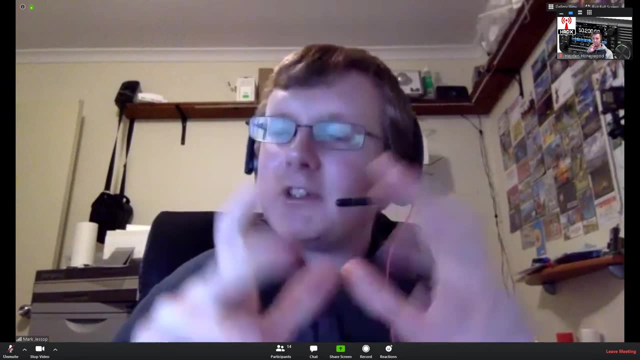 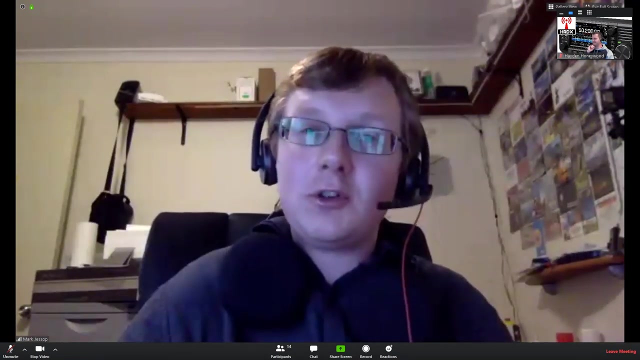 VK5 HZ. hello, I just want to say thank you, by the way, to VK5 HZ. He ran an AutoRx station at Davis Station in Antarctica for like six months. It was a really excuse the pun. it was a really, really cool to watch balloon launches from Davis Station. He also had the 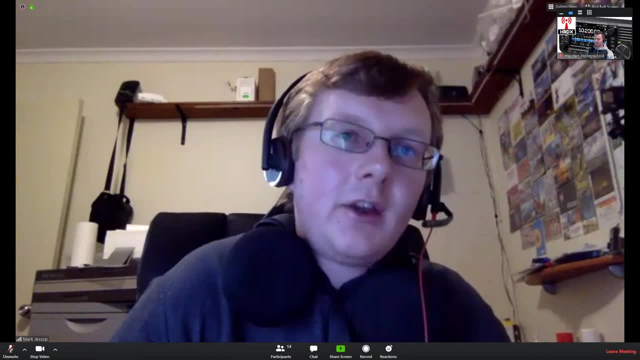 shortest radiosonde chase of all, where they launched a radiosonde from Davis Station. it broke off the string and landed within the Davis Station compound and he went and recovered it, So that's a really, really cool thing to watch balloon launches from Davis Station. 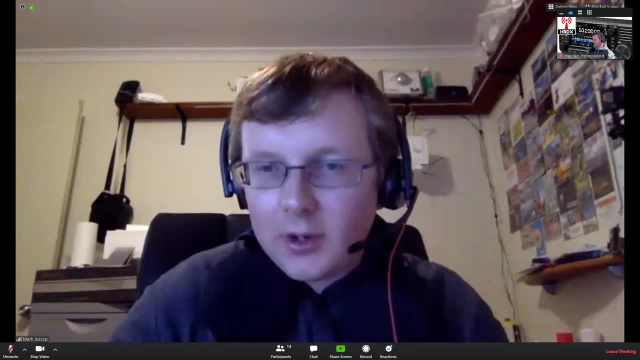 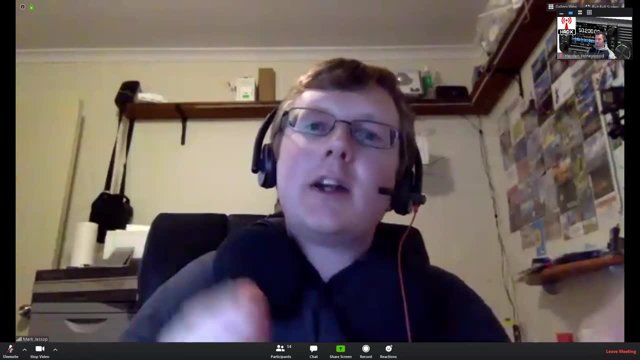 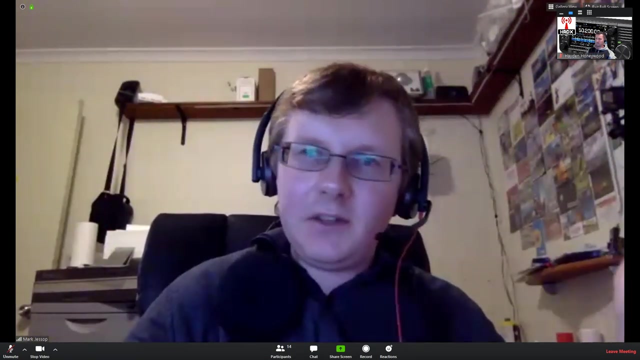 But afterwards that was pretty cool. The question was: do I have good success with landowners? And the answer is yes. Landowners- most people that own a large property- have seen a radiosonde before. These have been launching for years, many, many years- probably at least 50, I would say. 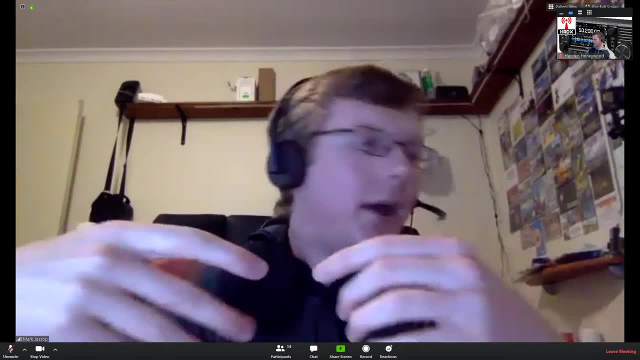 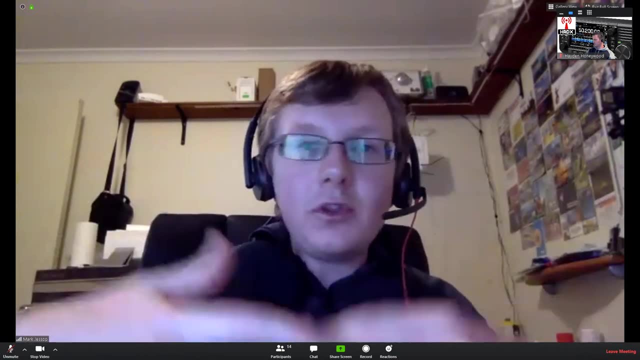 And most have found one on their property. So they know about them, they know what to look for, They know that it's not good if they get caught up in harvesting equipment, So they're more than happy to have someone go out there and recover this and have it not be an issue for them. 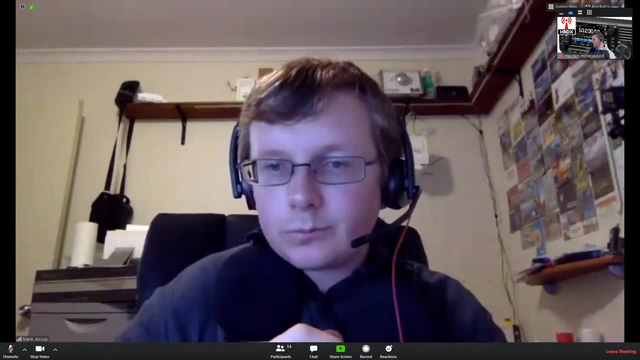 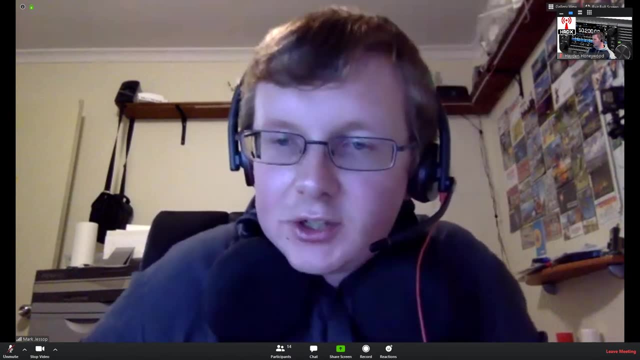 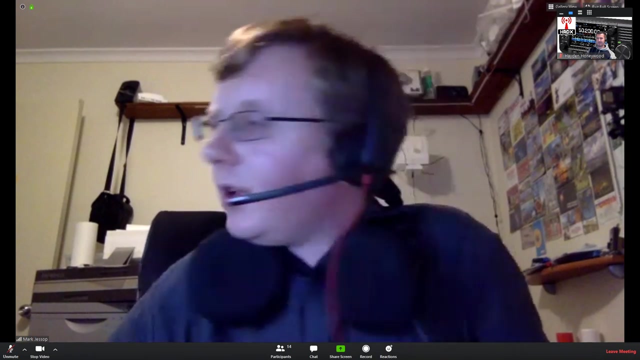 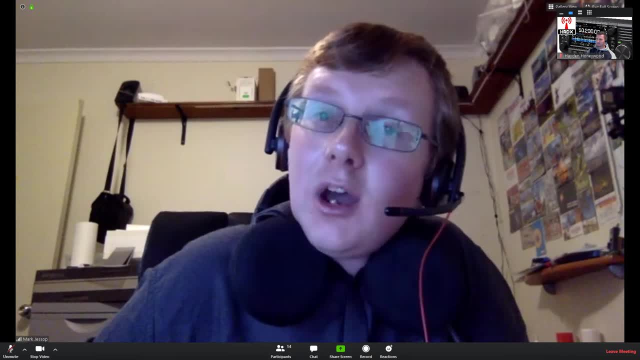 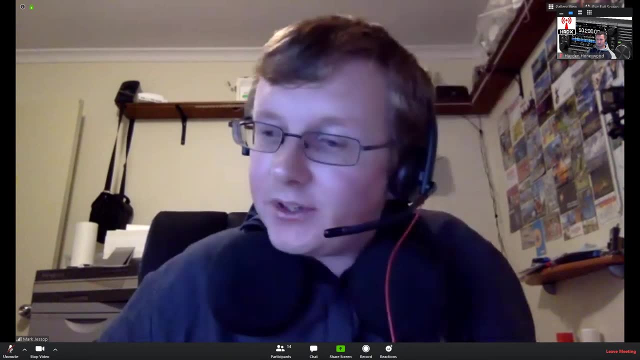 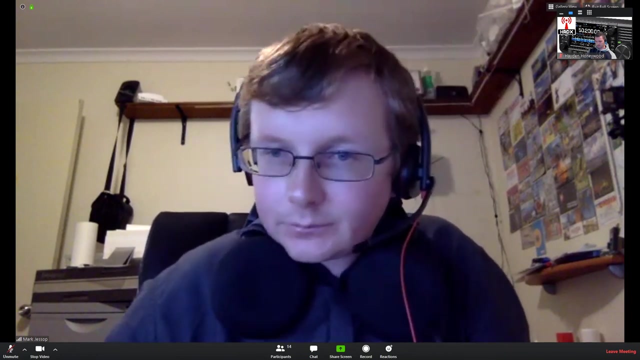 which is trying to decode more than one radiosonde at a time. with the RTL-SDR It's totally possible to do it. It's just a lot of effort to make it happen. Sadly, there's a lot of signal processing work required. It'll happen eventually, but I'll definitely need help. So anyway, that's the. 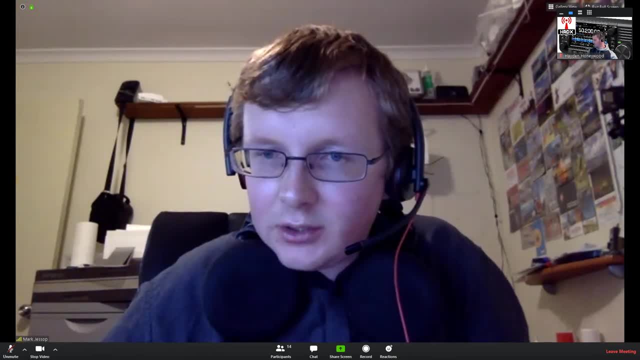 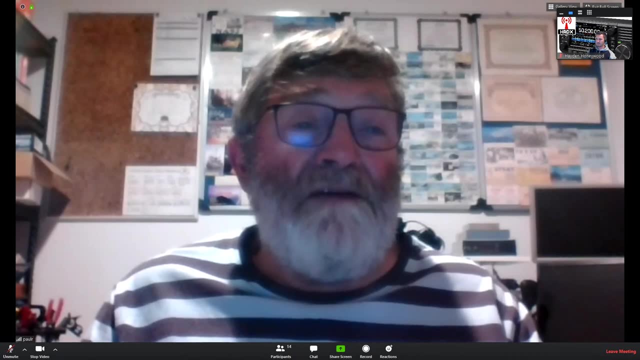 questions from online. Are there any other questions for me? Would you like to talk about port wakefield songs and the fact how you can get out there and have a good chase for half a dozen at a time? oh, okay, yeah, okay. paul comments on the port wakefield song. 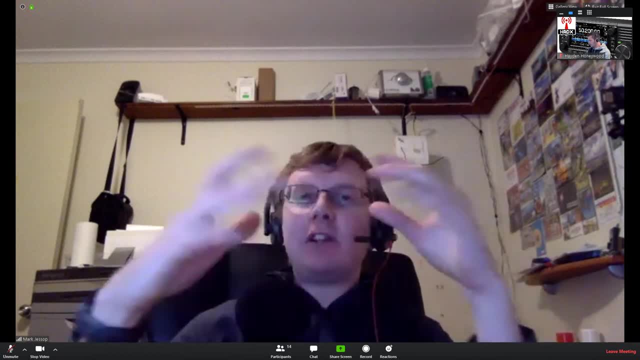 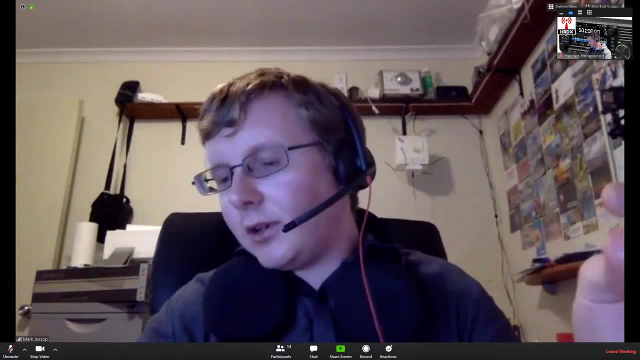 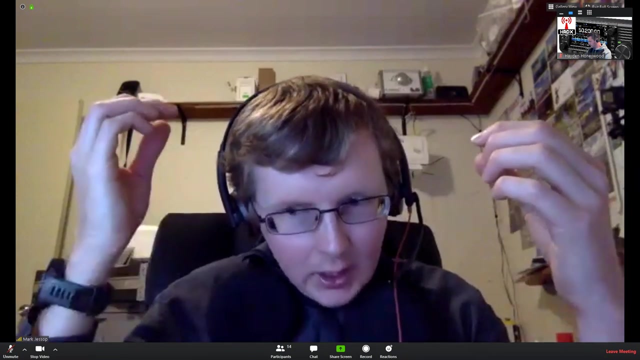 situation. uh, so there's an interesting story here about a year ago- a year ago, it must be about a year ago now. yeah, well, yeah, it was a year ago. i was in. i was on horn island when this all occurred and we started getting these reports in adelaide of people saying my receiving station is locked. 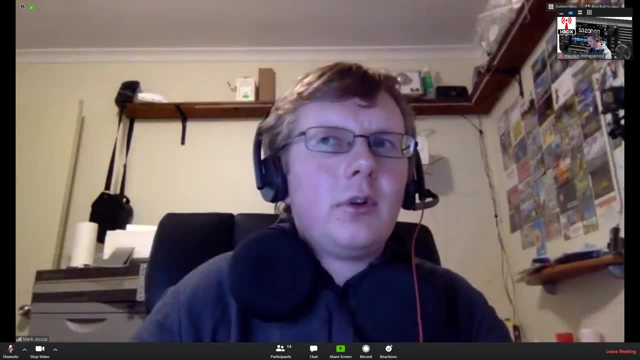 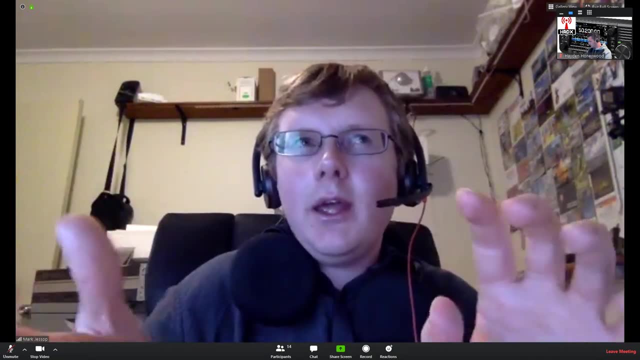 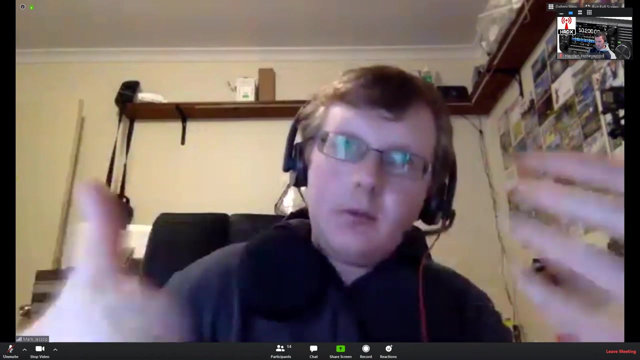 onto a radio sonde but i'm getting no data through and it was really weird. we couldn't figure out what was going on this. this was also occurring right around the time that we had a gps week number rollover. so again different sidetrack, but um, gps uses a week number and a time of week. 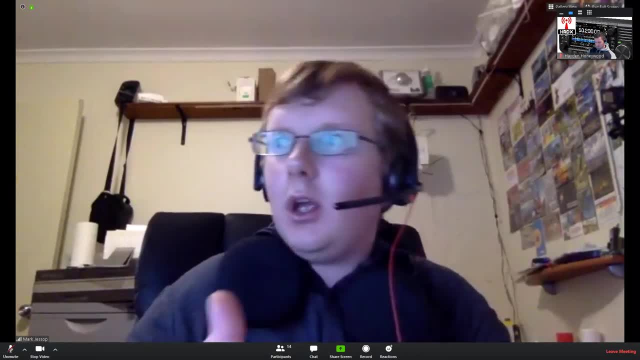 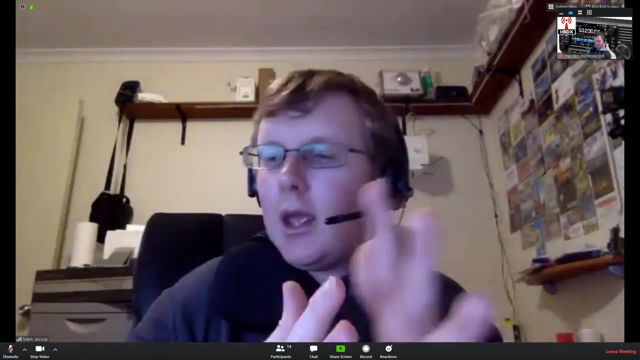 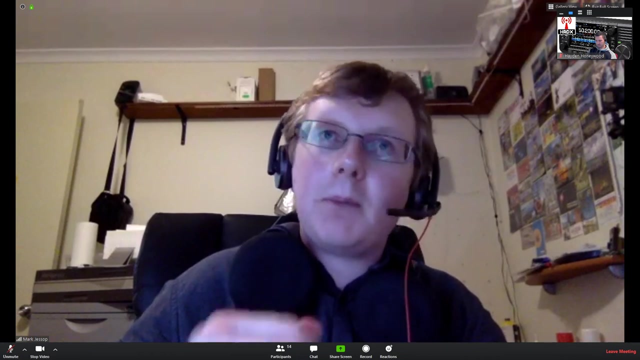 to represent time. week number is a 10-bit value. it reaches 1024, then it rolls back to zero. that occurred march or was it maybe eight april last year. when that occurred, lots of radios on launch sites, including every single vice silo launch site, broke, completely, broke um. they just didn't work at all. they had to get a. 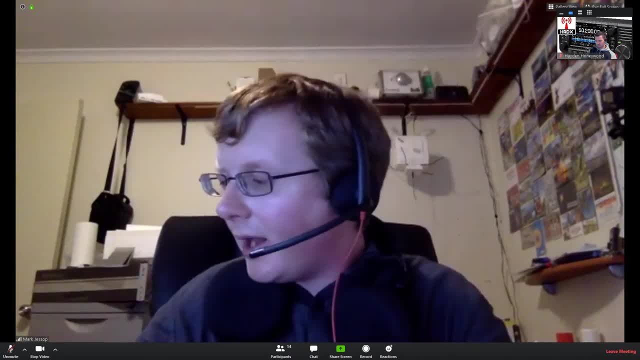 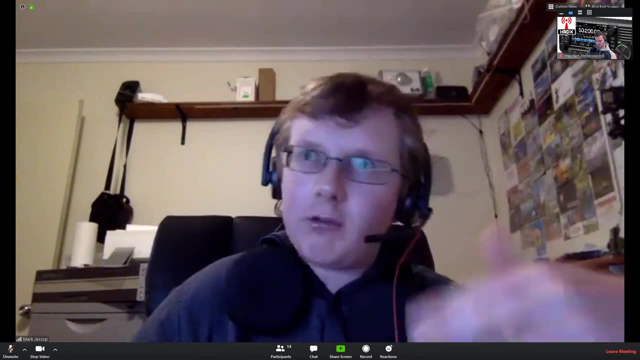 firmware update. it was about a week before the song station started launching again. during this time we noticed that these songs were showing up which we couldn't decode and we're thinking: is this something to do with the week rollover bug? and the answer was no, it wasn't. 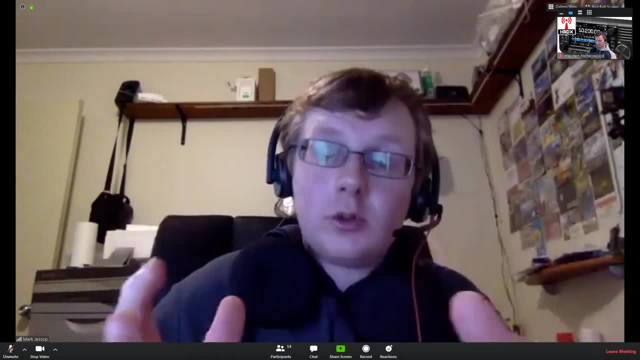 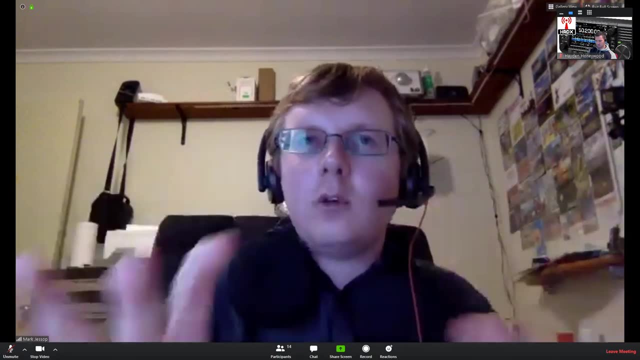 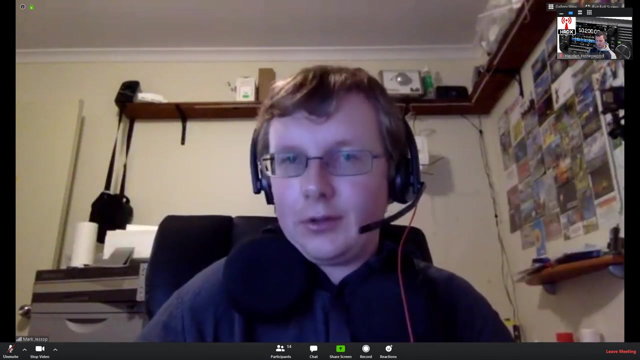 a bit of investigation and i'm sitting on horn island rules as a car. i'm sitting at a, but adding a hotel on horn island in the middle of the torres strait, playing with raw binary data, and i'm going. something doesn't make sense. here turns out that what we were receiving was encrypted. 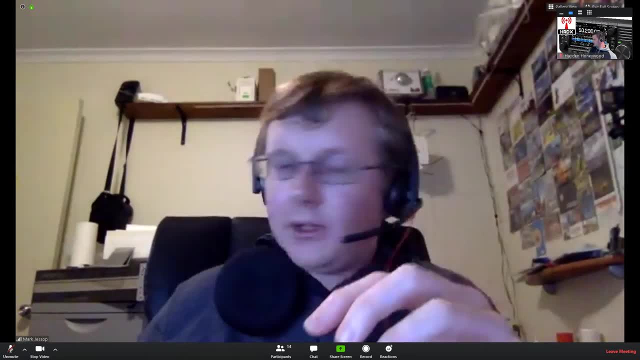 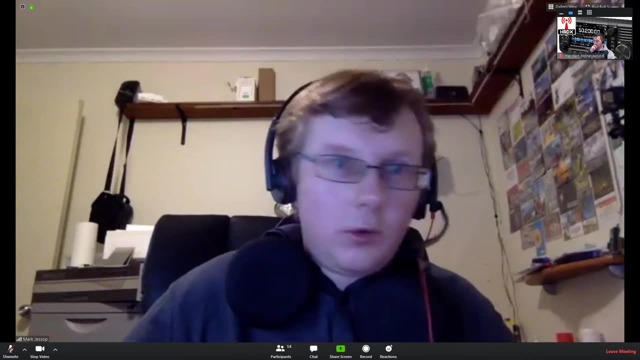 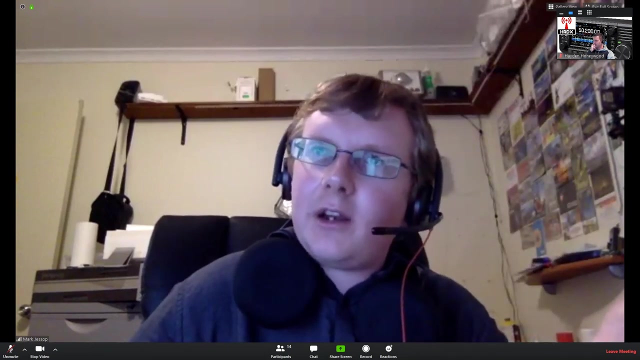 radiosongs. now there is a version of the rs-41 which is a military version, the rs-41m, which can, which by default is encrypted and we couldn't decode it. and obviously, and we're thinking where effective retraction finding, later we figure out they're launching from port wakefield now 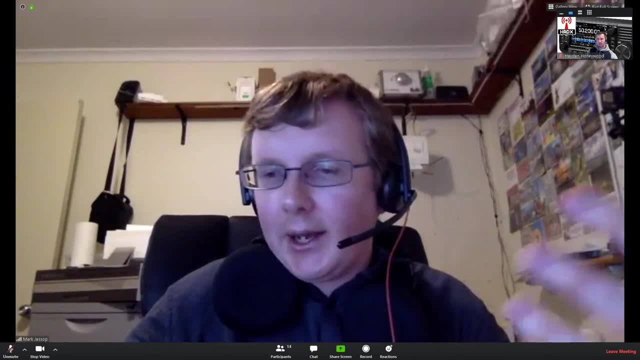 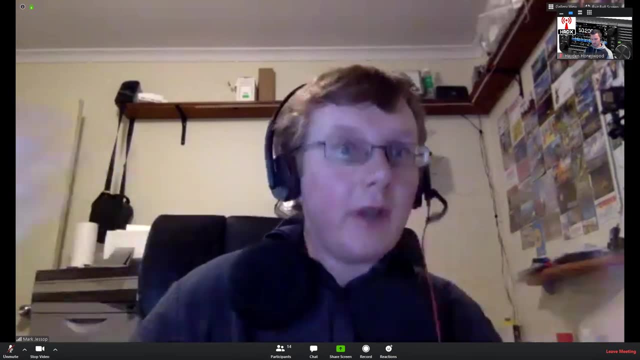 those that don't know, port wakefield proof range is a um. they do firing trials up there, all sorts of interesting things. if they're doing a firing trial, they want to know what the wind conditions are, so they launch radioscience. here we go. paul's got a rs41 sgm on the screen, not sure whether i 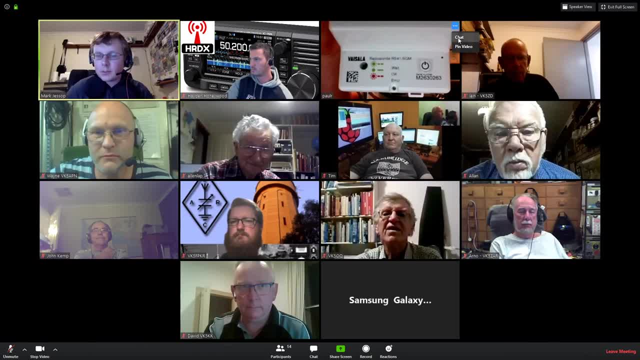 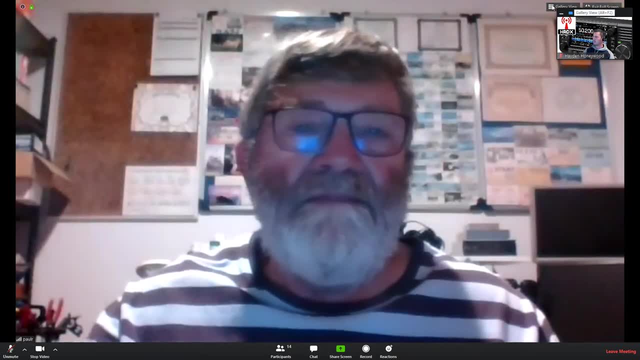 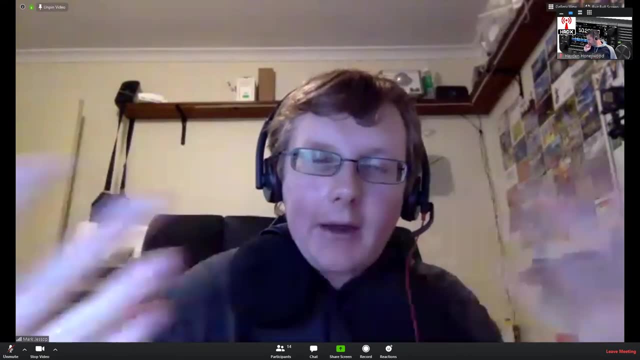 can highlight paul's video. let me just do that spotlight. paul, there you go, um, and there's an rs41 sgm. that's actually the old version, i believe. um. so anyway, um, we had a discussion with some people. uh, i managed to get a contact out of the port wakefield proof range and they 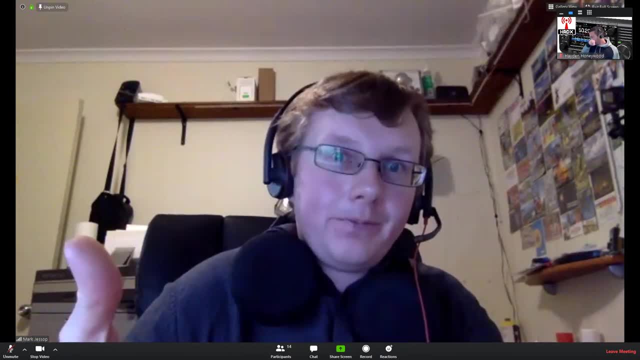 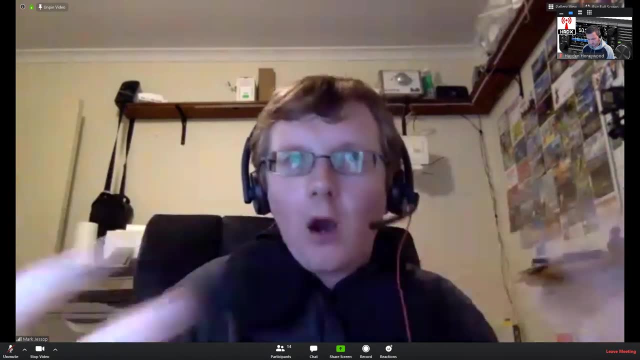 were kind enough to turn off the encryption, which was pretty awesome of them. what this meant was that we could now decode them. um, and when they do a firing trial, they launch a radio sonde on the hour every hour from about eight in the morning to the evening, and then they launch a radio sonde on the hour every hour from about eight in the 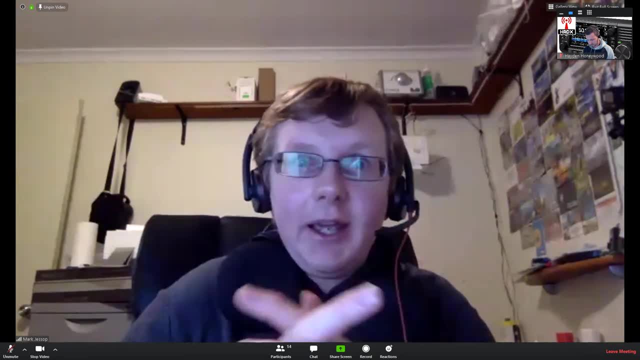 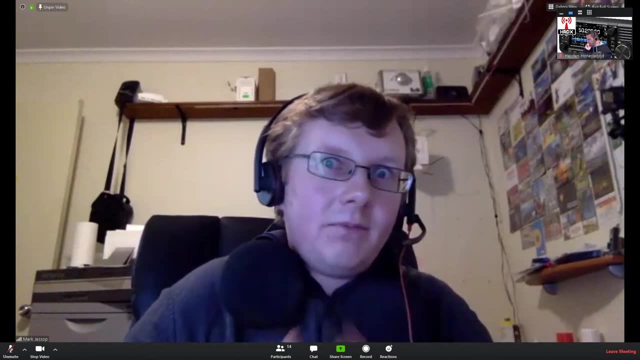 morning to the evening and then they launch a radio sonde on the hour every hour, from about eight in the morning to about three pm. that's a lot of radio songs per day, uh. so a few of us took the opportunity and spent, took a day off work and spent a whole day recovering radio songs. good, 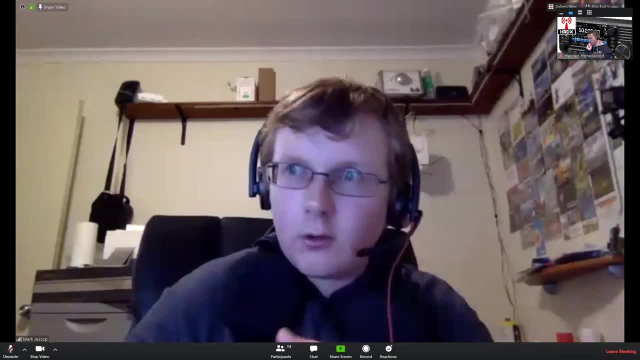 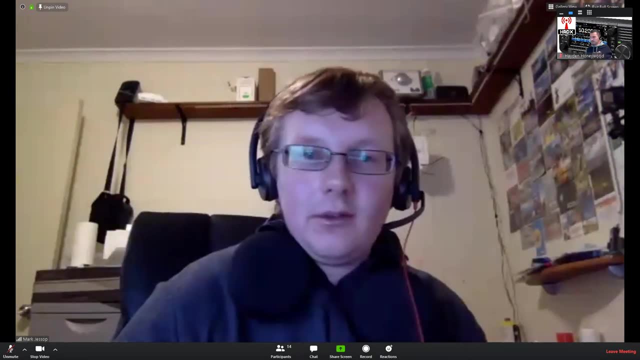 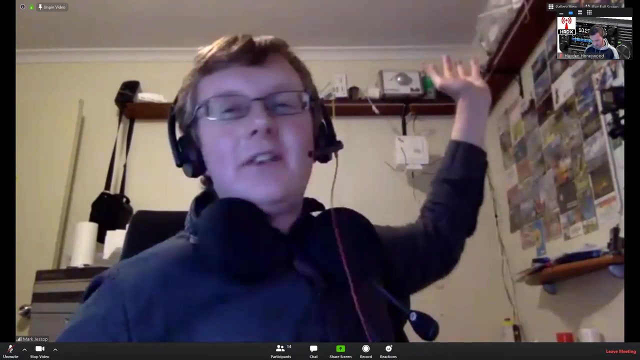 fun. uh, myself and liam gunning managed to get every sonde launch from one of the days. um, pretty cool. um, and yes, i went out once and only got one. yeah, paul says he only went out, went out and only got one of them. uh, sorry, paul. um, so i've got a whole stack of these things up on a shelf up here. um, 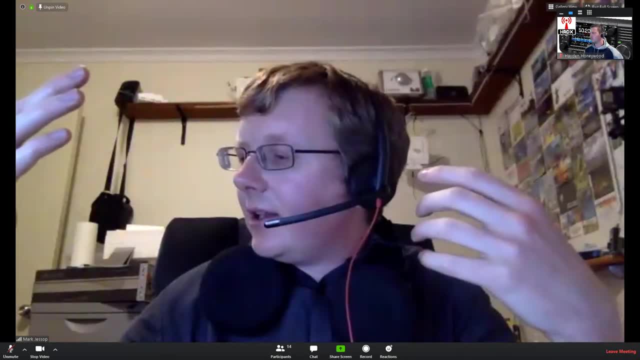 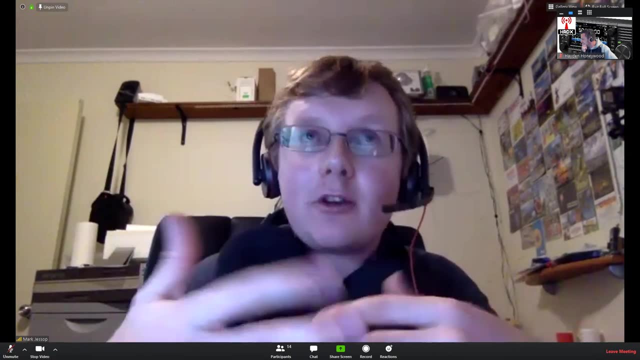 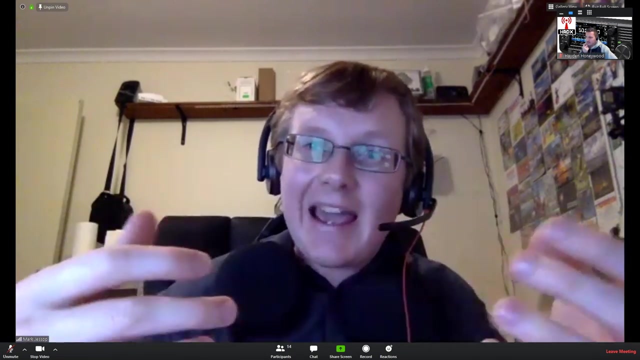 again. i just use them like regular radio songs. uh, we're not going to see that happen again. unfortunately, it's very unlikely. uh, that was for a particular trial. um, that trial has now occurred up at woomera when the trial was occurring. uh, many of the radio song receiving sites in adelaide we. 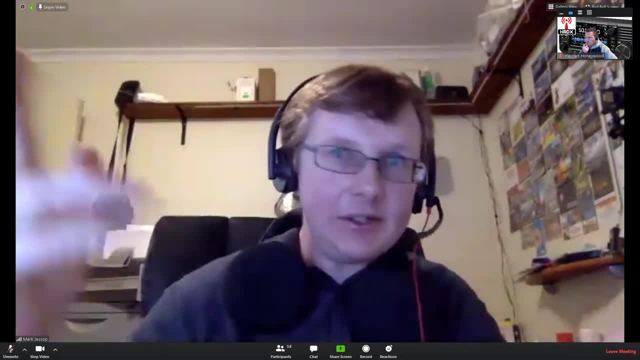 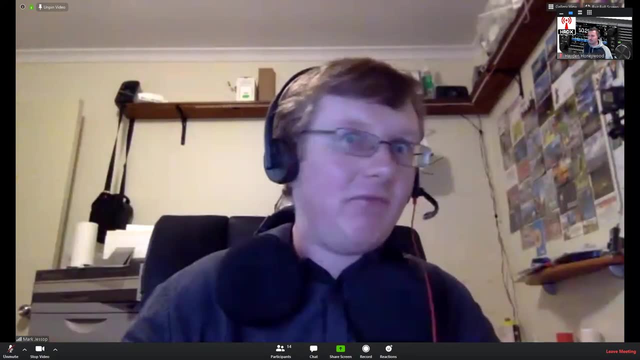 could actually see the songs from woomera. we would see, you know, seven in a day showing up at woomera. i don't know what they're doing, i don't want to know, but as a result, we got a whole bunch of radio songs to play with. it was awesome. so, yeah, thanks for that one, paul. 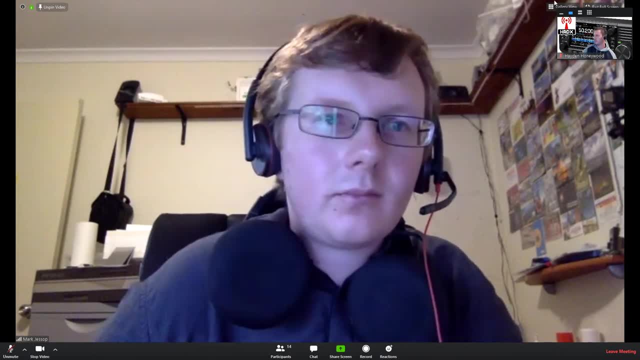 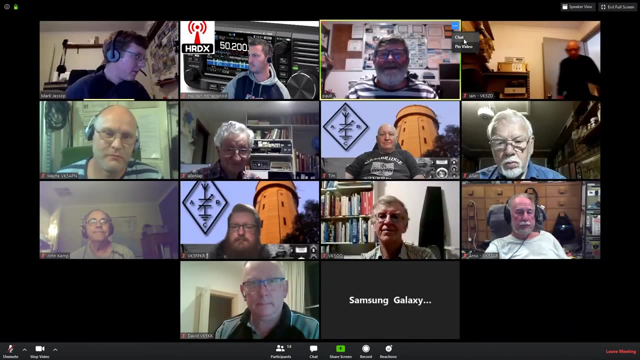 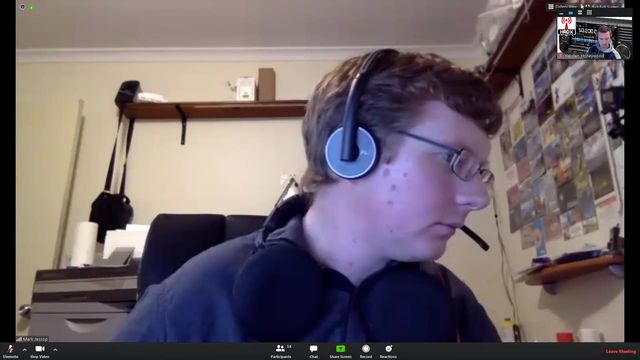 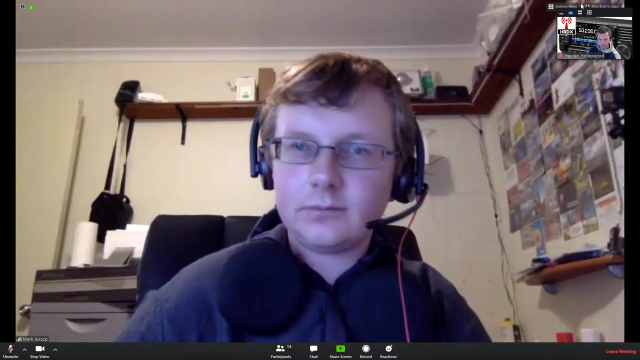 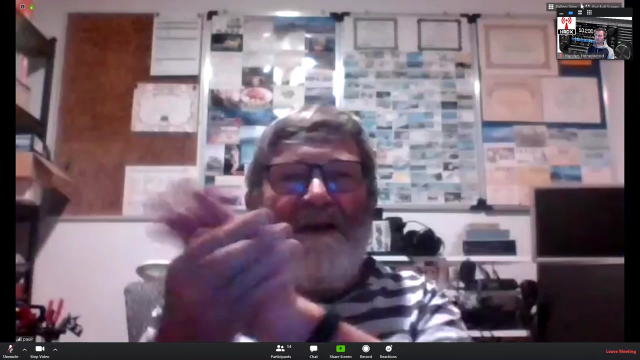 no more questions, any other questions before we wrap up. any questions from the people on vk5 rlz. this is vk5 qi. no nothing, no, nothing heard. i just want to say thank you, mark, that was excellent and, uh, a round of applause from everyone. please, no worries, thanks everyone and um hope to be back. 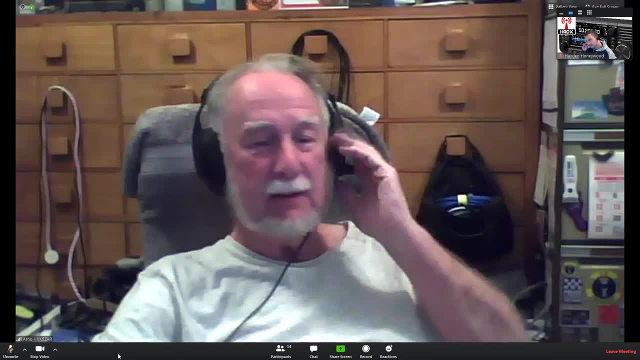 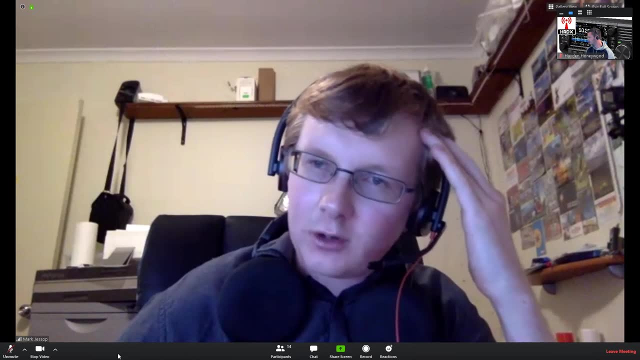 and talk about something else in the future. yeah, well, thanks very much, very, very good. just unmuted everyone and, um, yeah, thanks all. uh, thanks to hayden for streaming this as well on youtube. hello to everyone on youtube as well. yeah, and uh, i'll see you next time. bye, bye.